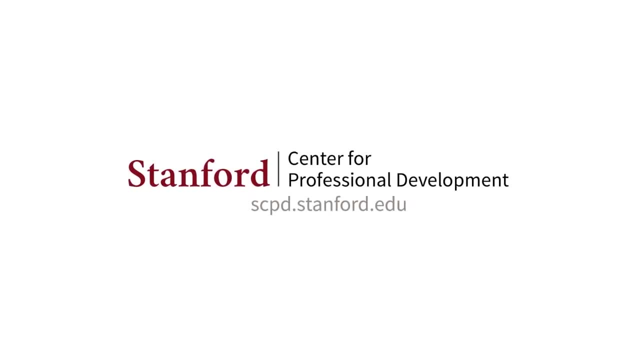 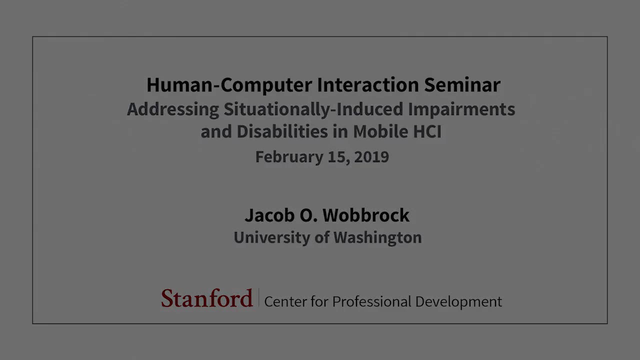 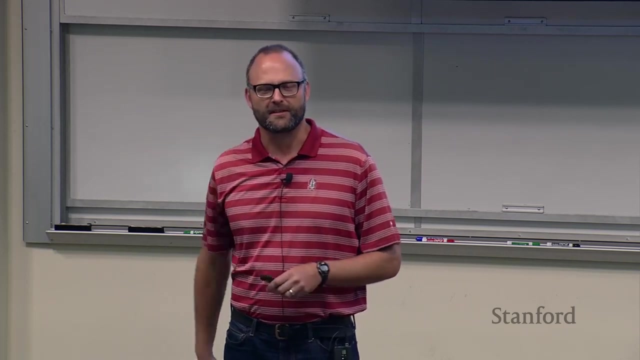 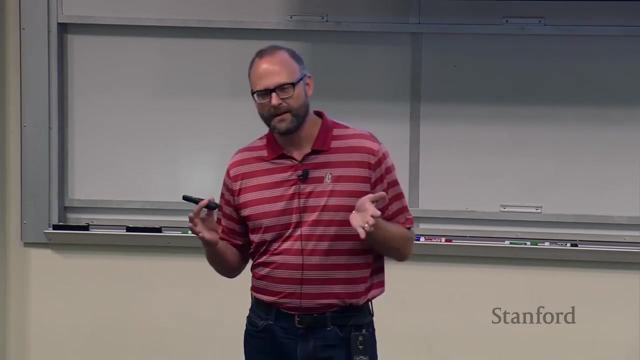 Well, that's probably the nicest introduction I've ever had. Thank you. I'm actually really experiencing a little bit of nostalgia because I've taken classes in this room. I've sat in those seats looking this direction, And I also have two of my mentors in the room. 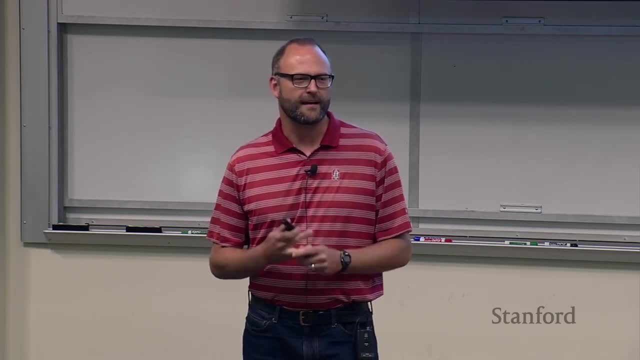 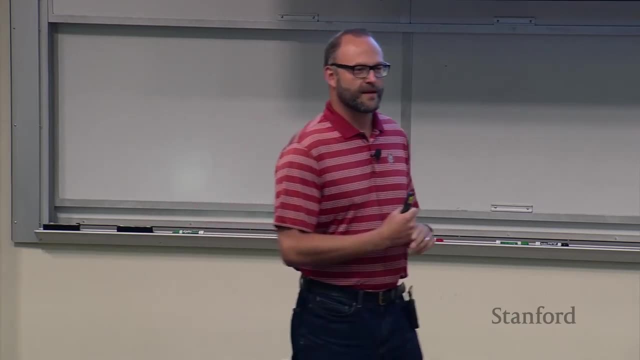 James Landay and Terry Winograd, who I can confidently say if I didn't know them and they hadn't played a large part in my life, I would not be standing here. So it's really special for me. It's also special to the point that I put on the last shirt I ever bought as 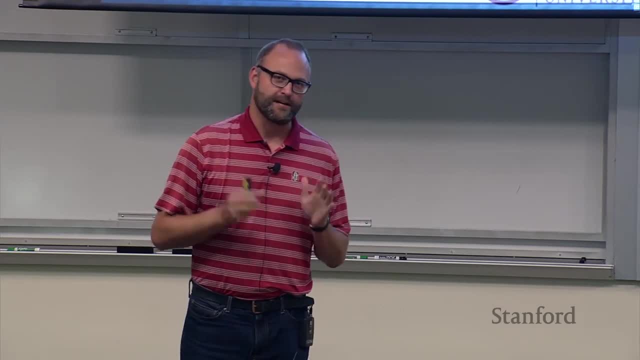 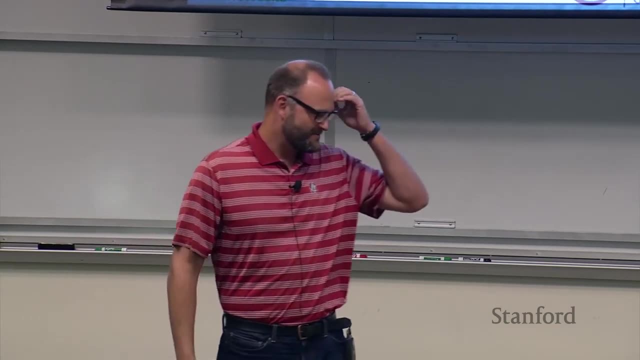 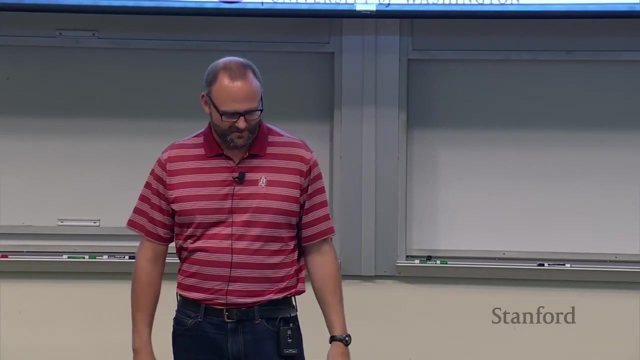 a Stanford student which was in the late 90s. Well, 2000, actually right on the number. So it's somehow shrunk over the last 19 years. It must be the humidity in Seattle. Don't tell anyone at UW I didn't wear a UW shirt, please. Okay, so today I want to talk. 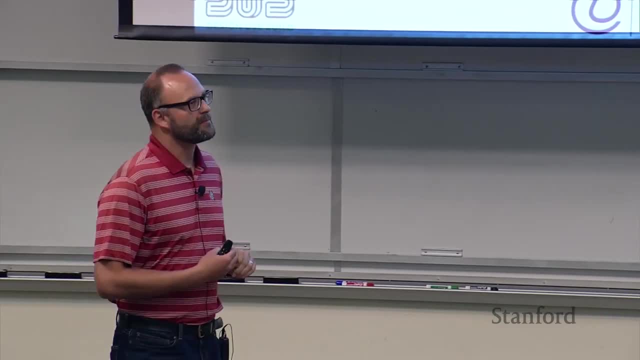 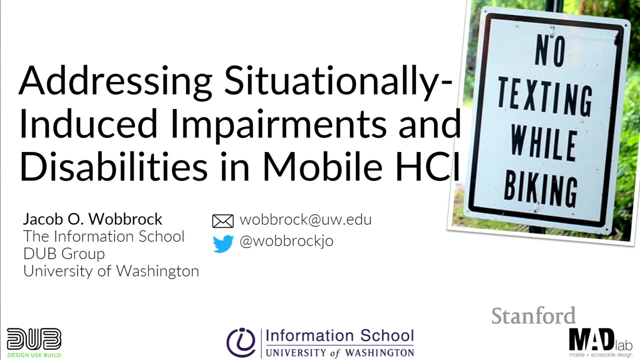 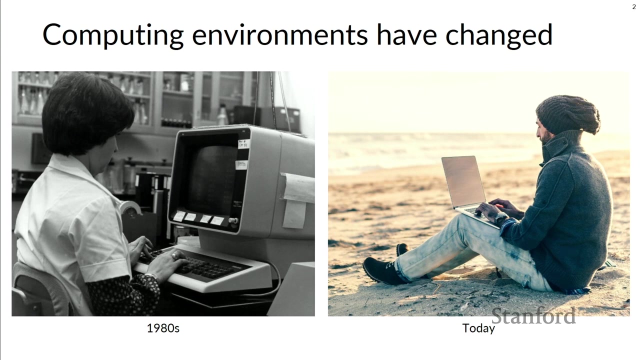 about addressing situationally induced impairments and disabilities in mobile HCI. No texting while biking. Those signs, that's a real thing. That's a real sign- I didn't make- that Computing environments have changed drastically in the last many decades, When 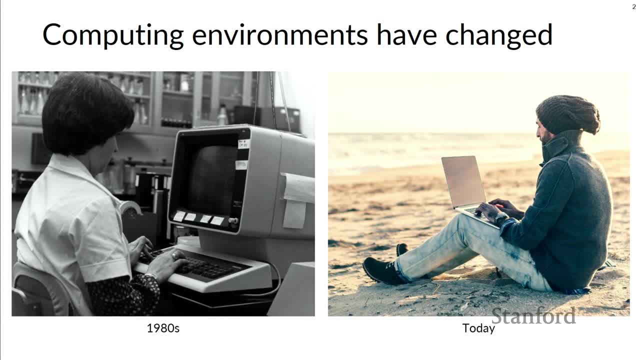 we were computing, interacting with a computer system, in, say, the 80s and I'm old enough to actually have done that. the assumptions about the environment we were in are very different than the assumptions we make today. We could assume we were in a stable temperature, maybe an 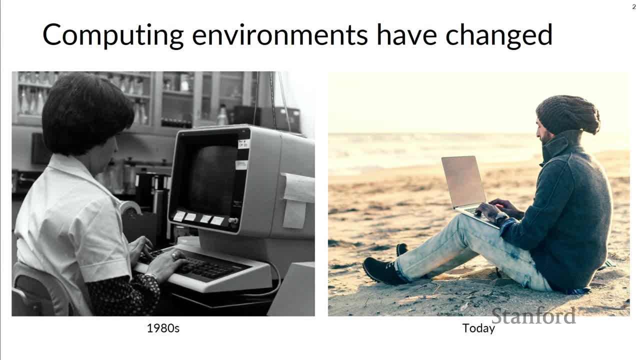 office environment. Things aren't moving, There's minimum distractions, Light levels are pretty steady. Generally it's a fairly- you know- staid environment. Today, like the picture shows, we might interact on a beach even with a laptop, which is still awfully close to the desktop. 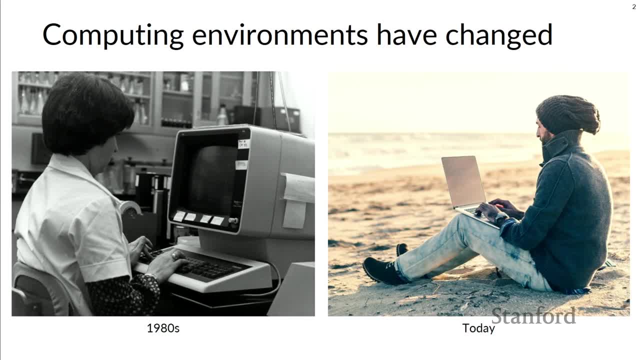 machine On the left in so many ways and yet sitting on the beach with sunlight, glare, it looks maybe like it's a cold weather beach, given the hat and so on, So it's maybe not very warm The hands might. 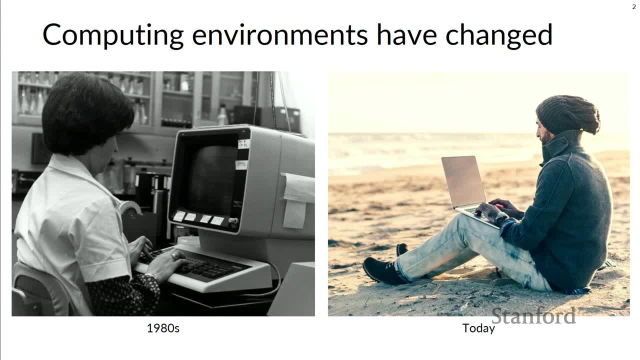 be cold, The fingers are stiff, And you know the posture is entirely different. There's no chair involved, All of those changes, And so that's just one example. But if we go even further, to smartphones and things, think about all the ways that we interact, both discretion at our 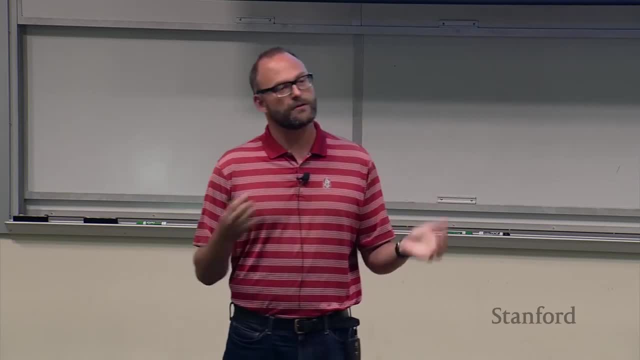 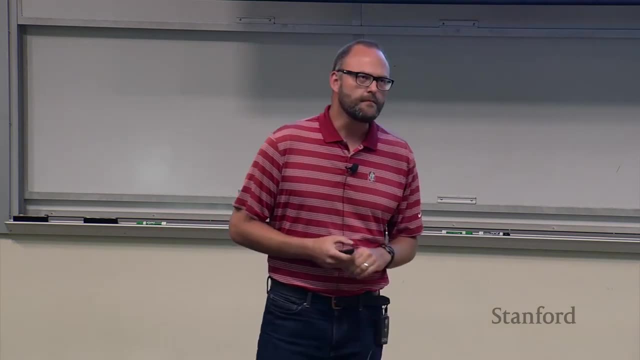 discretion, you know, just for enjoyment with your own personal phone. But also increasingly many jobs, many roles in the workplace are out of the office and in the field And there's a cost to this. So we have cognitive, perceptual and motor costs. probably others too. 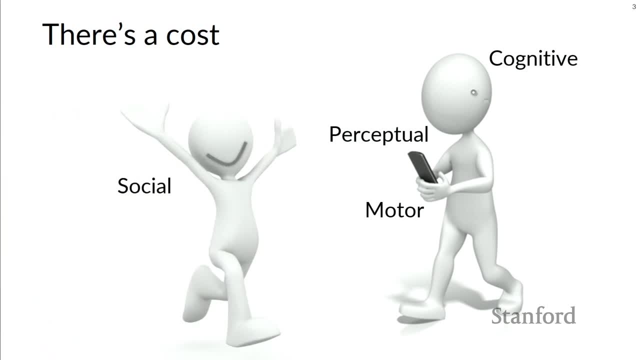 like social costs. You know, hello, it's great to see you, And we're distracted and don't notice, and then we make people sad. So it's important to recognize that this doesn't come for free. this flexibility of environments- How many times have you? 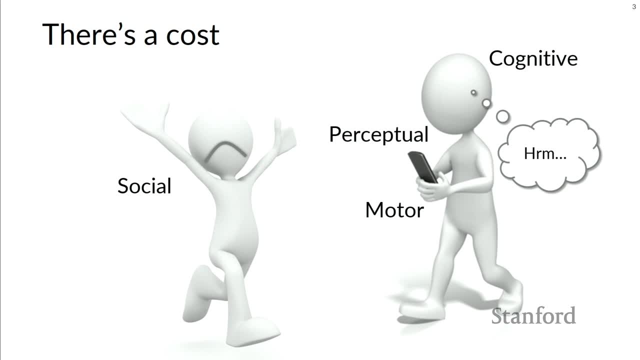 you know, been trying to get on or off a bus and someone doesn't notice you're trying to move past them because they're glued to their phone right, Or you've been that person, And it's not about making ourselves feel bad, but it is a recognition that this comes at a cost, because our attention is so. 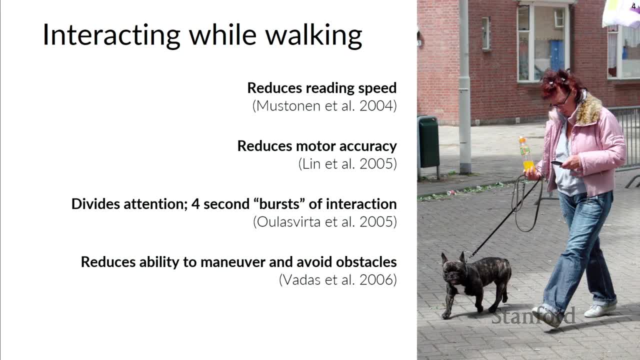 limited And studies have confirmed this. So we know that we have reduced, you know- reading speed, reduced motor accuracy- Actually, we tend to look at our screens in a way again with a smartphone when we're moving every four seconds. So that's a very, very important thing, And so you know. 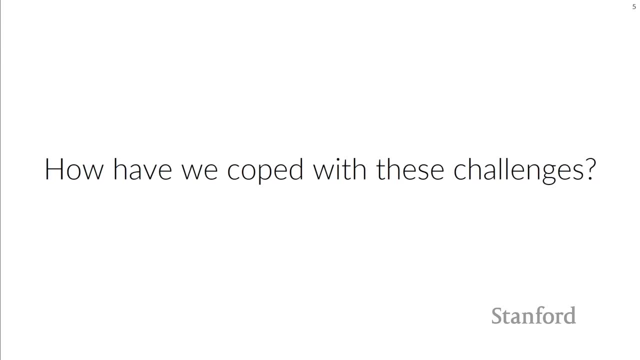 it's a very short burst of interactive time And we can't avoid obstacles as easily, and so on. So how have we been coping? When I say we, I mean kind of society like the world, the developed world at least. How have we been coping with these types of challenges? Well, 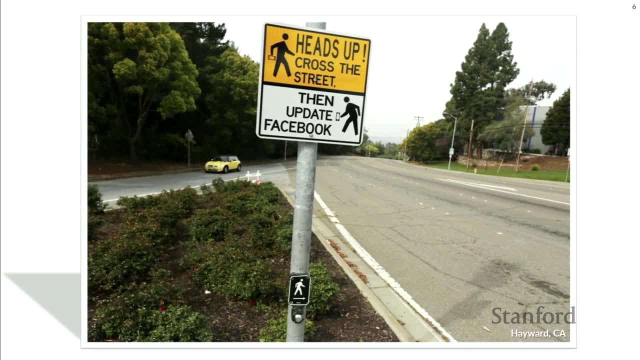 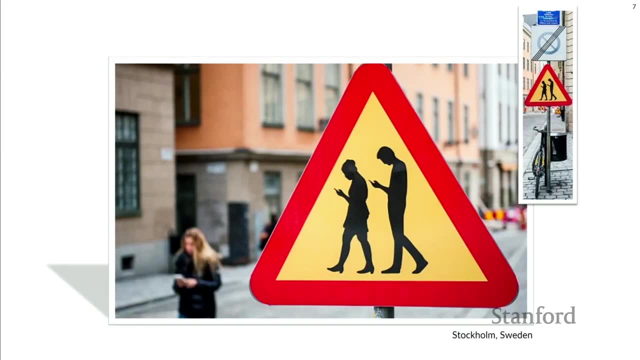 here's one way: Heads up, cross the street and then update Facebook. This is a real sign from Hayward, California, in the state we're in Further afield, Stockholm, Sweden, decided they were tired of trying to notify the texters to wait, And so they started to wait, And so they. 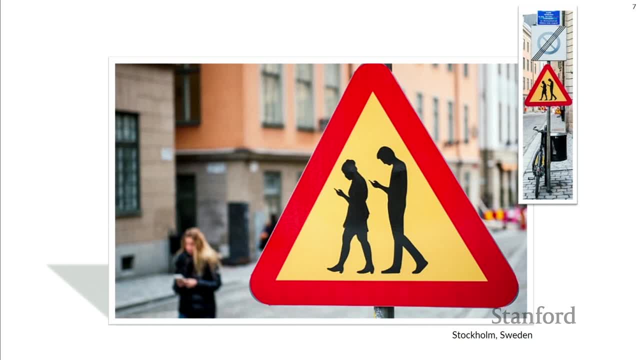 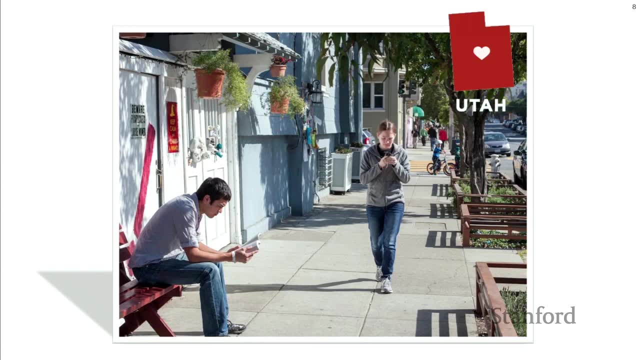 started notifying the drivers not to hit them, So beware of the drivers. Yield to the texter who's not paying attention. In Utah you can get a distracted walking fine now, which includes texting. It's a $50 fine the first time and $100 the second time. That's not, I think, statewide. 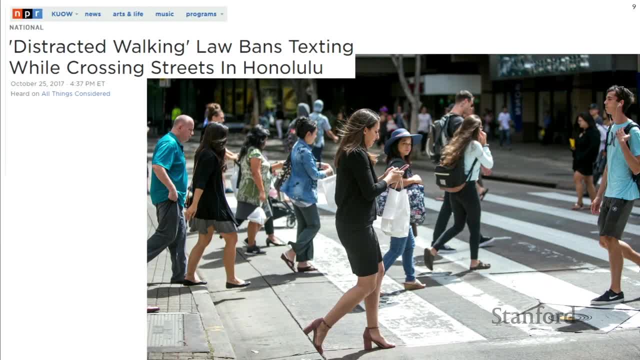 I think it's Salt Lake. Honolulu was in the news last October because they passed a law that if you're caught texting while in the crosswalk, so you're in the crosswalk, which you know. that's where you should be right, You're not jaywalking, But if you're texting while doing, 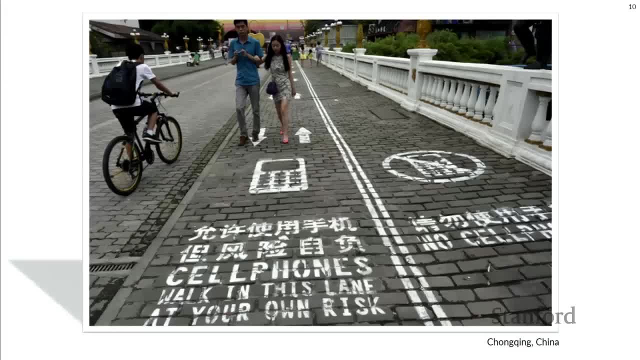 so you can be slapped a fine right on the spot. This is over in China. They experimented with two different lanes Cell phones. If you want to walk with your cell phone, go over here- It's at your own risk, Or you know, the cell phone-free lane Turns out this as a social experiment failed. 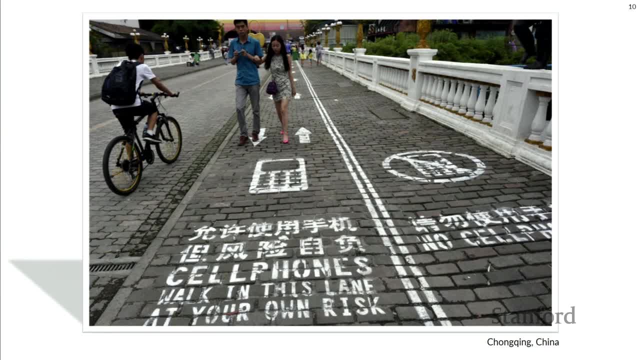 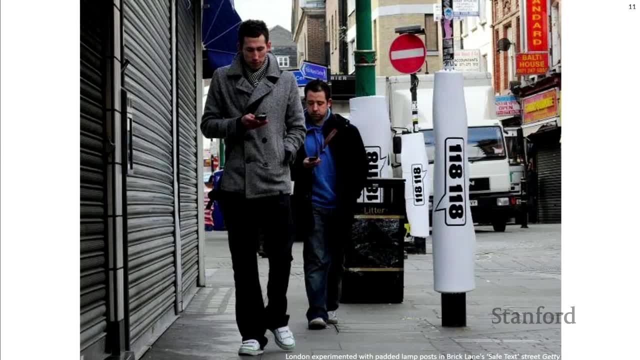 because people were so enamored by the instructions they would actually crowd the cell phone lane reading the instructions and kind of, oh, look at this. And then people would run into them. Actually there's a whole neighborhood in London that put padded. 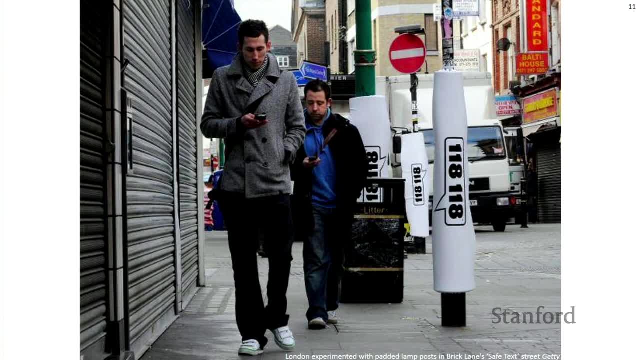 lampposts around because people were running into lampposts. So notice what we're doing here. We're actually changing the environment to accommodate behavior that is based on our interaction with these devices that consume us. In Amsterdam they said: well, you're already. 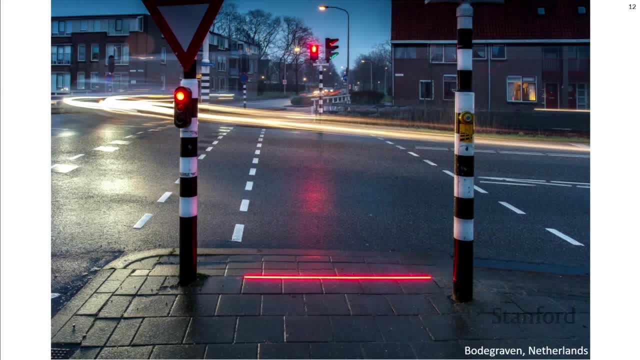 looking down in some fashion. so maybe we should actually be putting the signals on the ground. That's kind of clever, Nice design idea. It's kind of an elegant image. I like that one. The US Federal Communications Commission, which is the US Federal Communications Commission, is a very good. 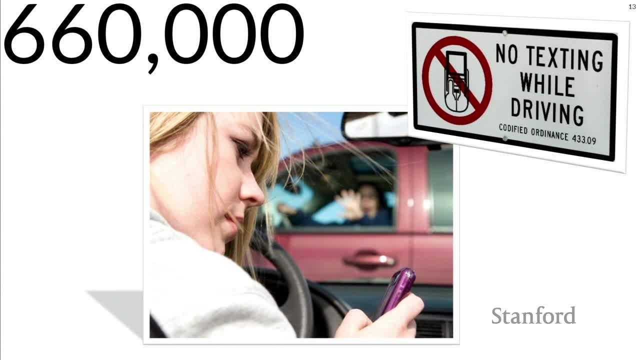 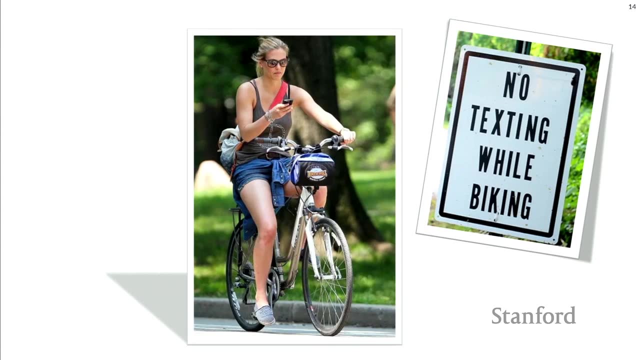 organization, The Federal Communications Commission, estimates that at any one daylight moment in the United States, 660,000 people are texting while driving. If you kind of divide that out and sort of portion it out by cities and geography, that means someone near you. Don't do that, And it doesn't just have to be you know driving, It could be. 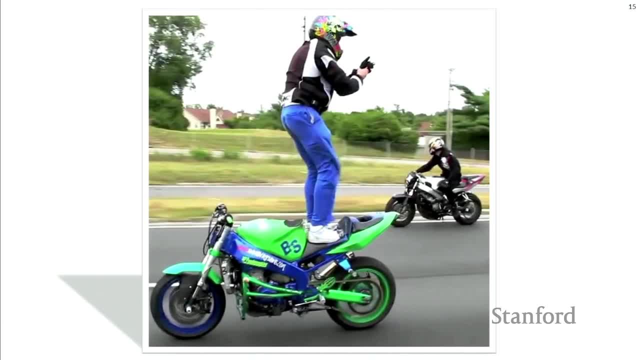 on bikes, bicycles, right. I don't know what this is all about exactly, although there was an article attached to it which said that this person wanted to show that they could stand on their motorcycle and say, oh my God, I'm driving, I'm driving, I'm driving, I'm. 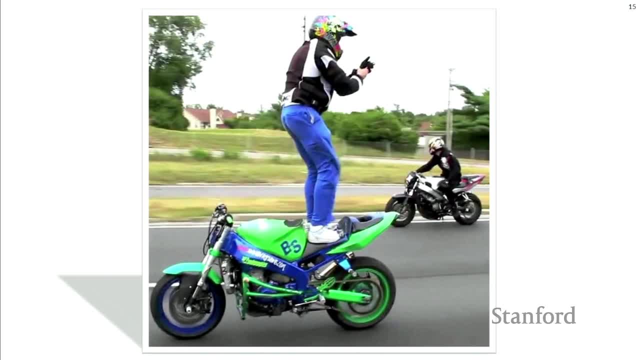 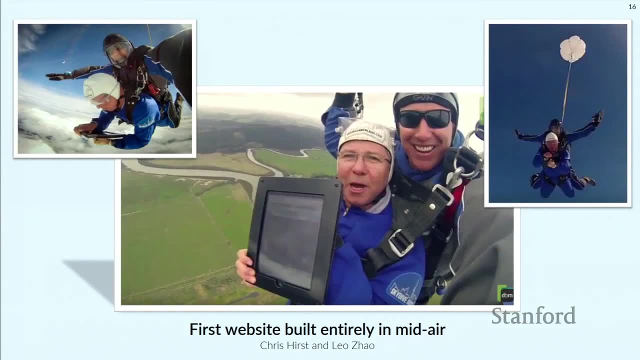 going to send a text while riding backwards. But notice also, they had to remove the glove from their hand, So there was a clothing encumbrance there as well. We'll break some of those down later. These folks went really to an extreme and this is getting a little absurd. but that's. 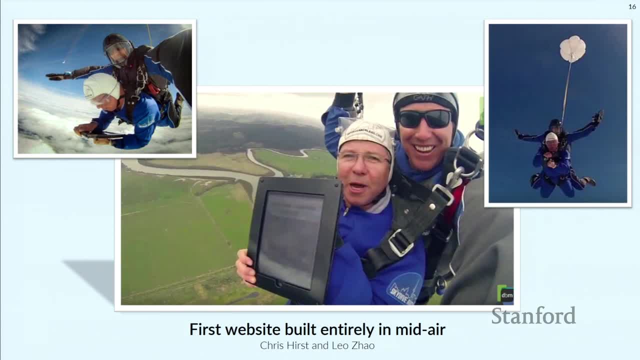 why it's funny. They actually jumped out of an airplane and used their company's software on a tablet to build a website from start to finish before they hit the ground. So they said: it's so easy to use. You can be this. 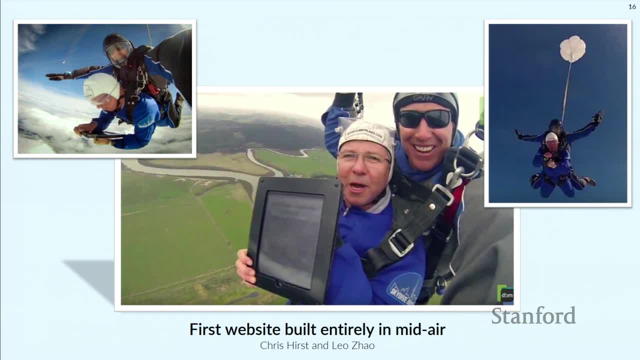 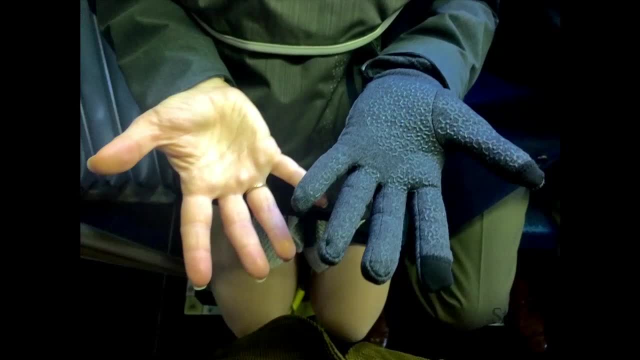 Situationally constrained and you'll still be able to build a website that fast. I don't know how high they were. Maybe they went really high so they had more time, But we don't have to get that ridiculous. So how many of you have owned gloves that specifically have the? 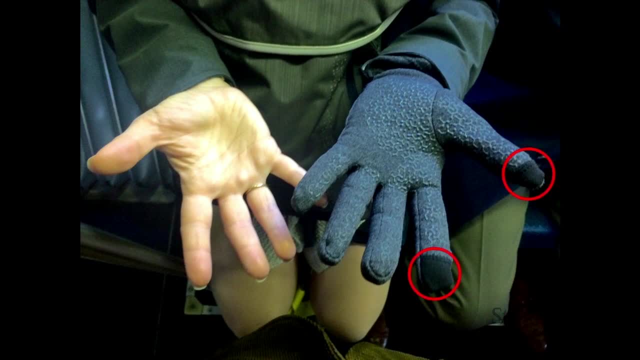 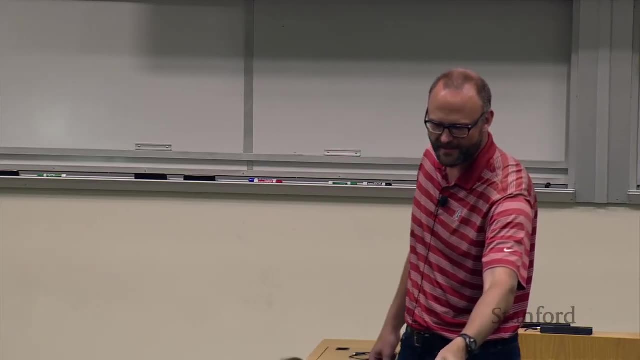 capacitive sensing fingertips and yet you still take off your glove to interact with Exhibit one. Do you take these off when you actually need to like on the bus, or do you leave them on? I need fine-grained, precision light control. 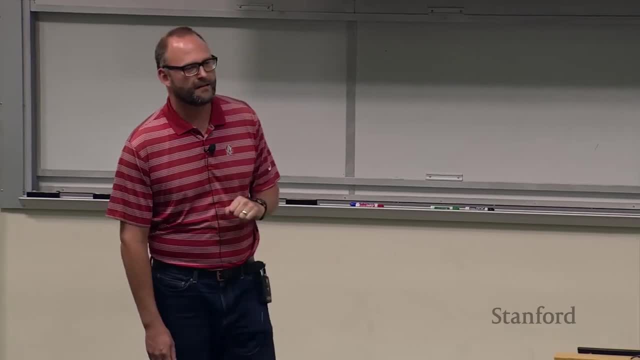 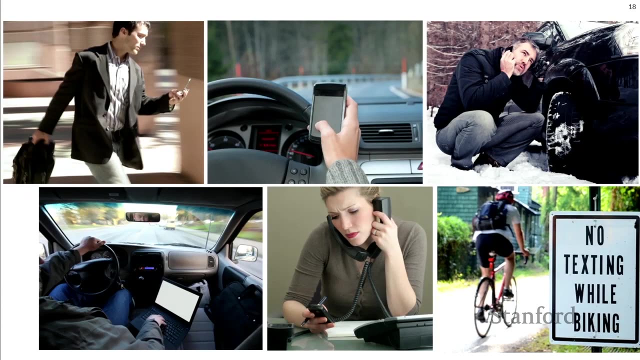 Yeah, Yeah, I mean some work better than others and they're improving, but it's not suddenly the magic bullet usually. So the point of all this is that we interact in ways that constrain us, that affect our abilities. The environments exert a lot of pressure on us. 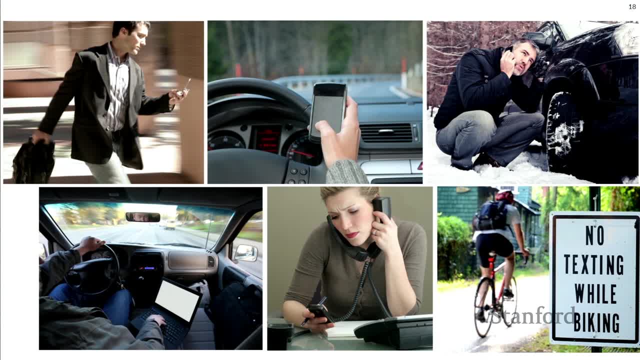 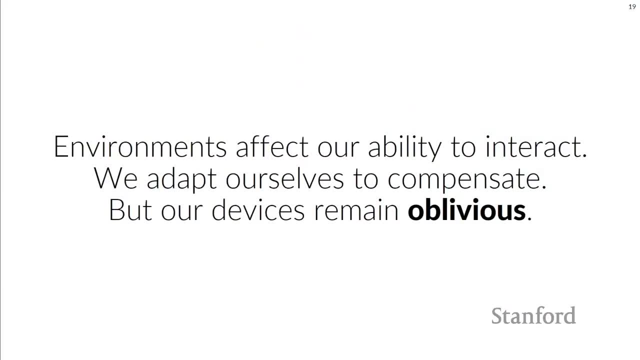 and our attention is diverted in ways that make that challenging- And there's lots of ways that this can happen And our abilities to interact are compromised, and then we go and adapt ourselves. But the point I want to leave you with from this is think how little the computer and 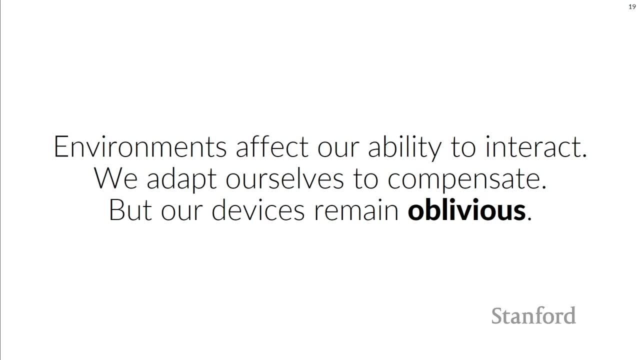 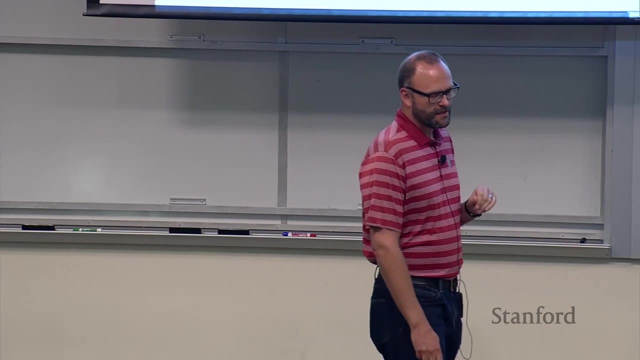 I say computer meaning very broadly the smartphone, laptop, whatever. think how little it actually knows about where you are and what you're doing. It knows almost nothing GPS-wise. it kind of knows a Latin longitude, but that's not really your context. It just doesn't know. 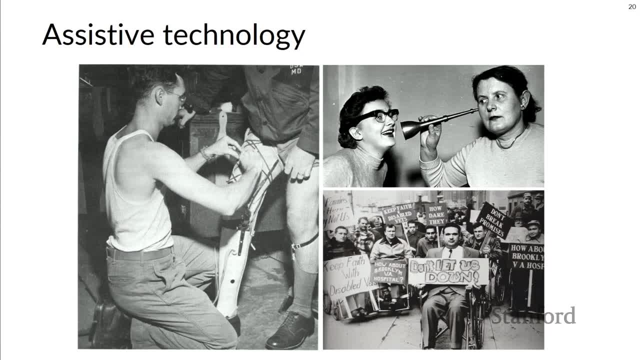 They're pretty oblivious And we have a long history of again advanced computer science And I think we need to keep a long history of adapting ourselves to a rigid world And we see that very prominently in assistive technology. So these are images in the post-World War II era. 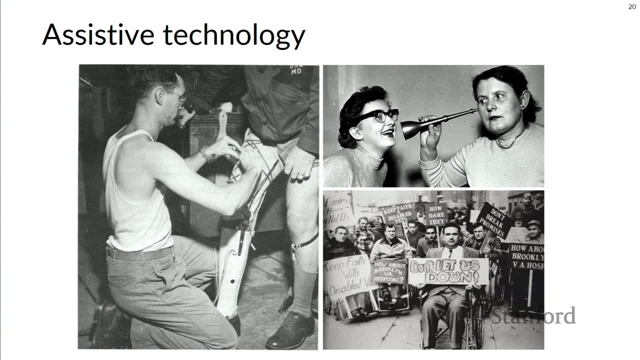 The belief was that the environment is static. disability exists within the person, So if you've lost a leg, we're gonna give you a replacement so that you can now adapt back to the environment. right, We're gonna make you what you. 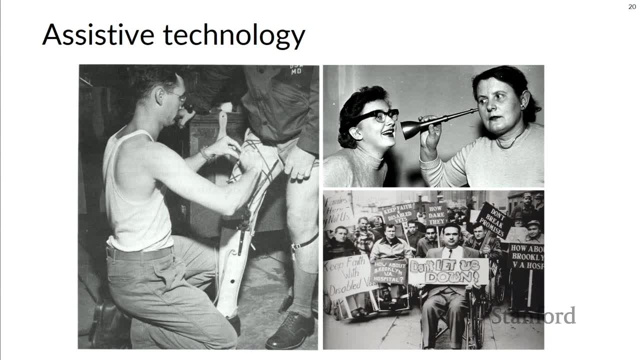 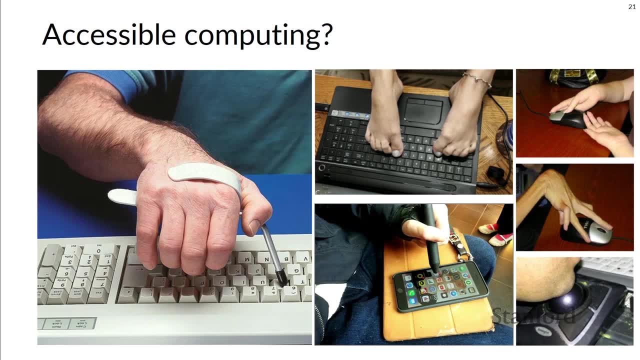 we're gonna restore you to what you had before. perhaps, And this is kind of an old image set of images, but we still have this adaptation today. Here are images of people working with devices that don't have any idea that in this case, there's a motor limitation. 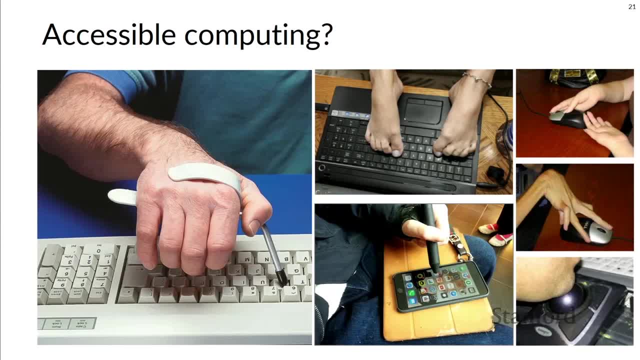 The image up in the top. that person has no arms, so they actually learn to type with their feet And some other using a trackball with your chin. some of these images are actually from my studies And again, the devices don't know, the computer systems don't know. 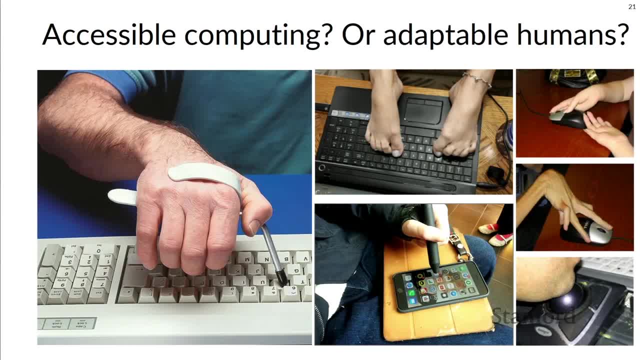 So is this really accessible computing, or is it actually evidence of adaptable humanity? right, Humans are incredibly adaptable. that's why we're still here for now, And so I would submit that these kinds of things are less about accessible computing and more about adaptable humans. 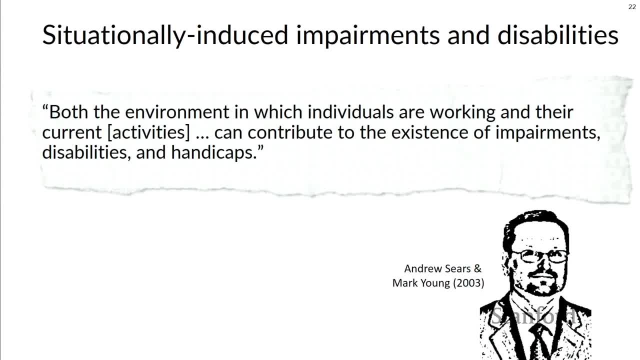 So it's because of that intersection that people in accessible computing have realized and kind of tied a link to say: the environment can actually impair you, The environment, the situation can disable you. Andrew Sears was the first to put some language to this with these exact terms. but 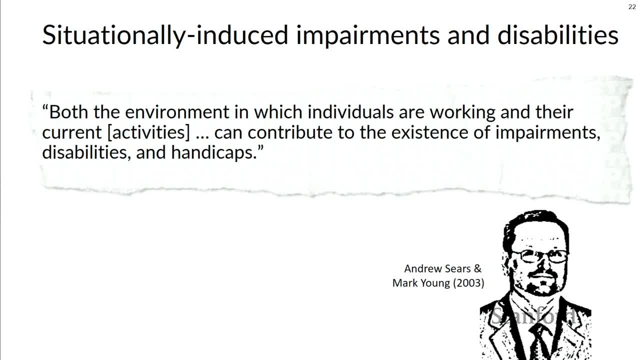 as I'll show you in a moment. it's been thought about for a while, He says, both the environment in which individuals are working and their current activities. so what they're doing, what they're trying to do, can contribute to the existence of impairments, disabilities and handicaps. 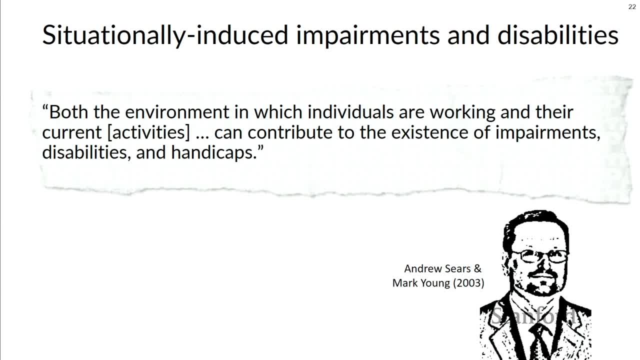 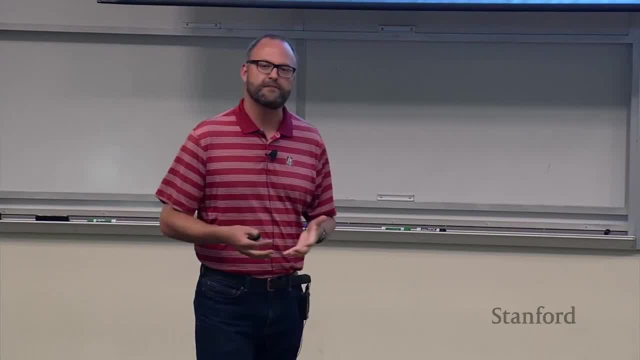 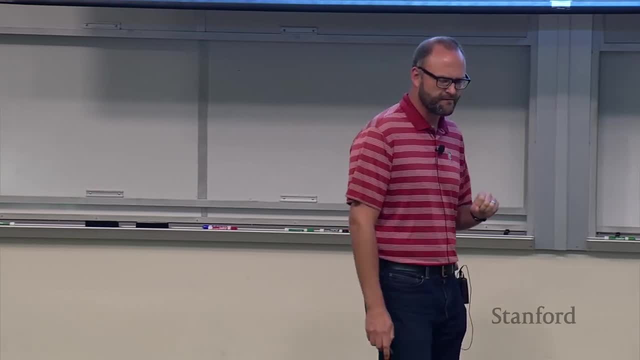 Well, that's kind of interesting because that means any of us could be disabled, Depending on the environment and the activity. Okay, well, we'll come back to that, because maybe that takes something away from other kinds of disabilities. But let's go with that for now. 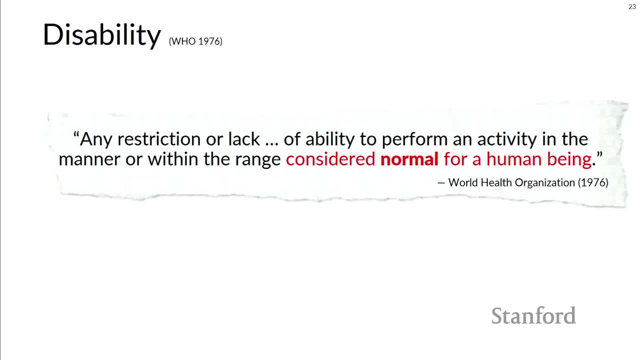 Now this might seem at some level obvious, Like: well, sure, of course the environment, especially after all the images I've shown you, the environment clearly can cause you to be impaired in some way, or disabled maybe in some way. 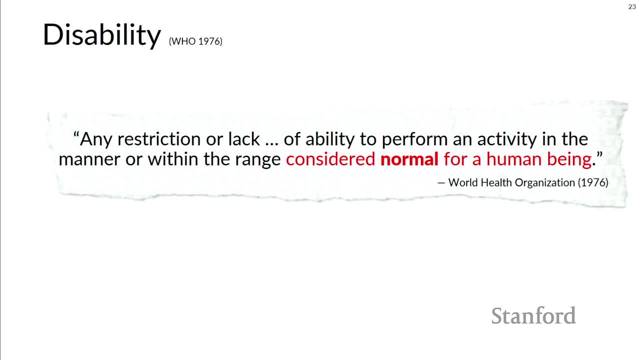 But it wasn't always thought about that way, As I said, with those images of the assistive technology after World War II. disability, originally by the World Health Organization when it was finally formalized in a definition, was defined as any restriction or lack of ability to perform an activity in the manner or within the range considered normal for a human being. 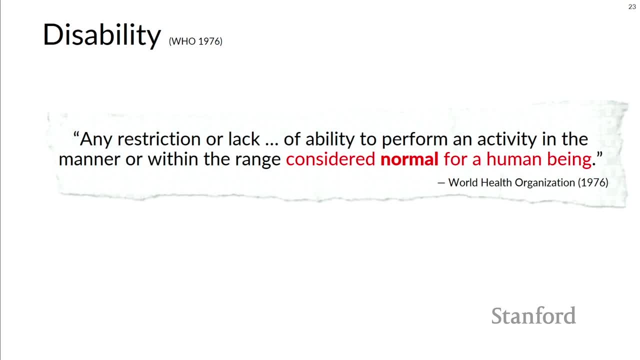 It's from the 70s, It's obviously very normative language. You know what's normal? It's kind of like the myth of the average person. Everybody's different Individual differences are the only normal thing. Fortunately, this is deprecated and we no longer place disability just within the person. 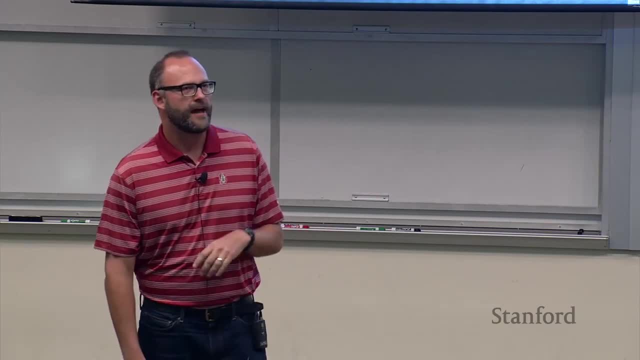 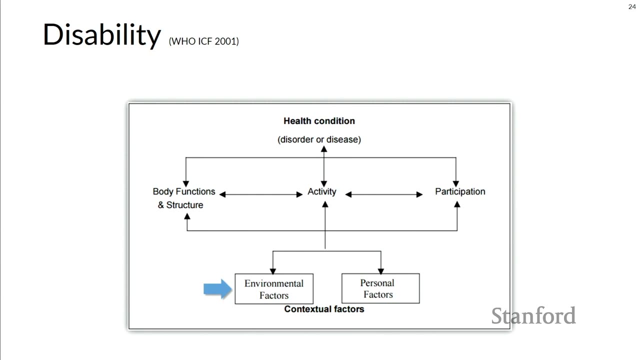 It's not just inside you and only there. In fact, there's a complex model, but I'll point out that environmental factors are now called out, as well as the activity and other things. We haven't lost body functions and structure, But there's more at work here that contribute to a notion of disability. 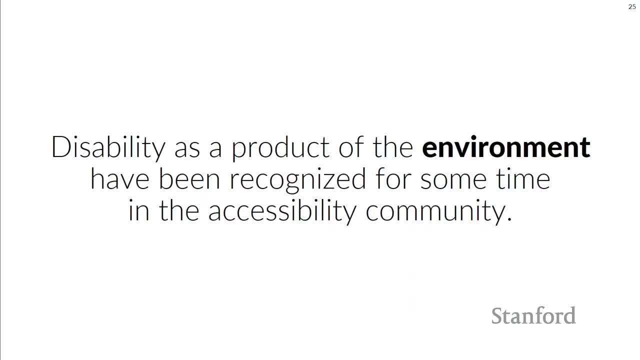 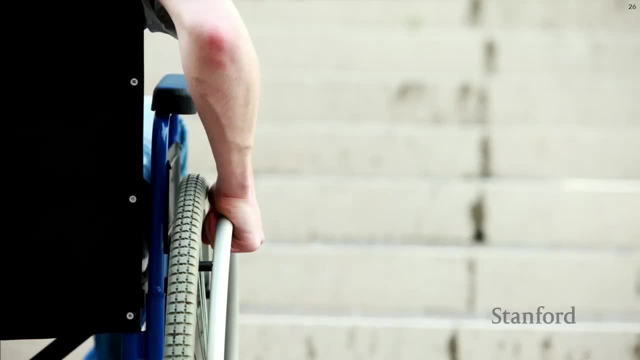 It's a more complex phenomenon, It's not just within the person. So disability as a product of the environment has been recognized for some time in the accessibility community. So when I show you this image and I say where's the disability, what do you first think? if you're honest, 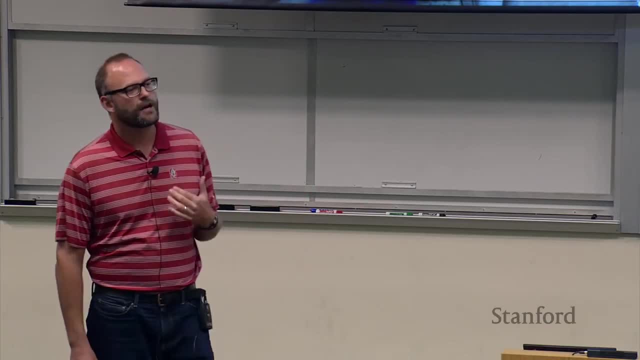 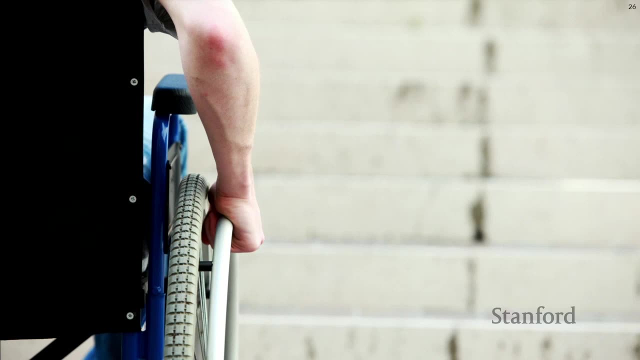 Well, there's a guy in a wheelchair right. Well, yeah, that's not untrue, but it's not really the whole story. The disability: it's a little blurry on the big screen, But the disability also is because there's a set of stairs there. 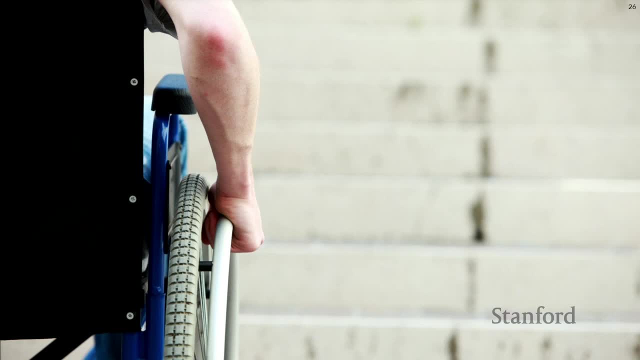 And presumably, given his orientation, maybe he wants to go up the stairs or wishes he could be at the top. That would be the goal. But the disability therefore lies not just within him but also within the environment, Because if that was a smooth ramp, he would not be experiencing a disability in that moment. 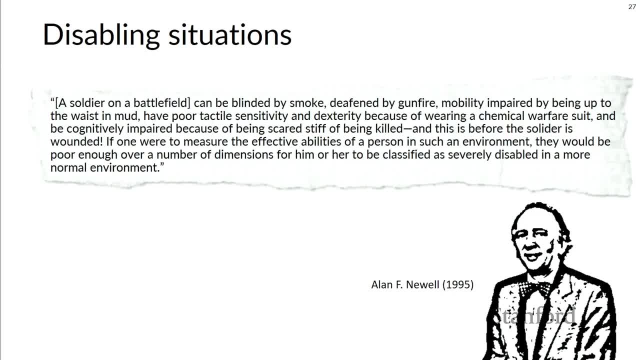 So clearly in a simple example like that, we see the environment plays a big role. Now I do have a little bit of text. I try not to make slides with too much text, But there's some quotes I want to read you before we go on to some projects that we're going to talk about. 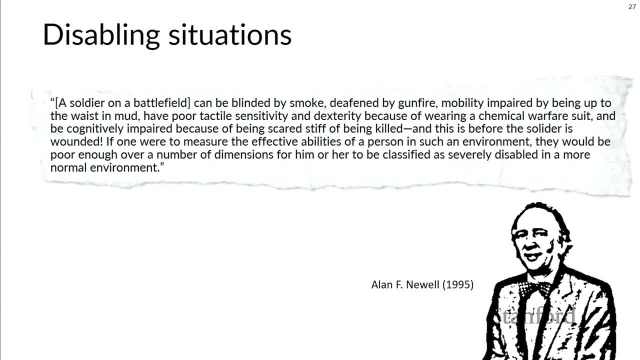 So I'm going to read you a couple of quotes. So I'm going to read you a couple of quotes before we go on to some projects that we're going to talk about. So I'm going to read you a couple of quotes before we go on to some projects that we've done to address these things. 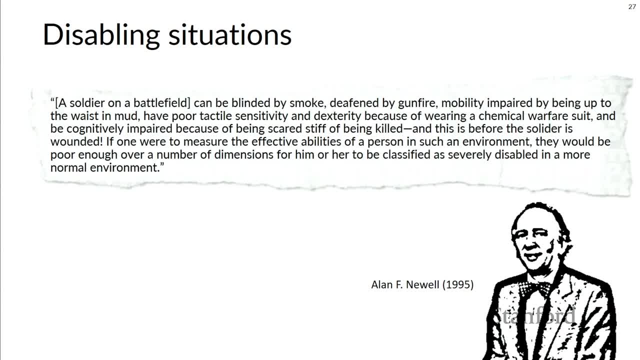 And they're kind of early, foundational quotes. Alan F Newell also was a CHI Social Impact Award winner years ago And he observed a very similar thing, without the language of situational impairments, but a similar thing way back in 1995.. 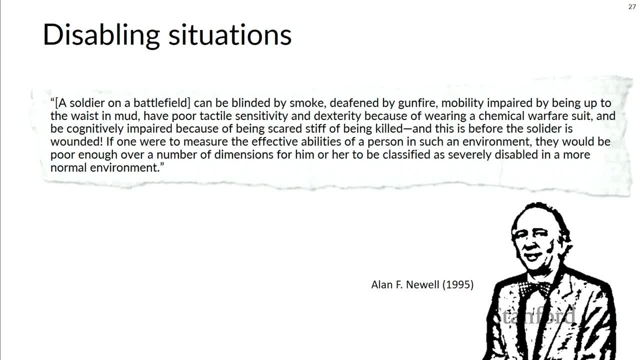 He said, a soldier on a battlefield can be blinded by smoke, deafened by gunfire, mobility impaired by being up to the waist in mud, have poor tactile sensitivity and dexterity because of wearing a chemical warfare suit and be cognitively impaired because of being scared stiff of being killed. 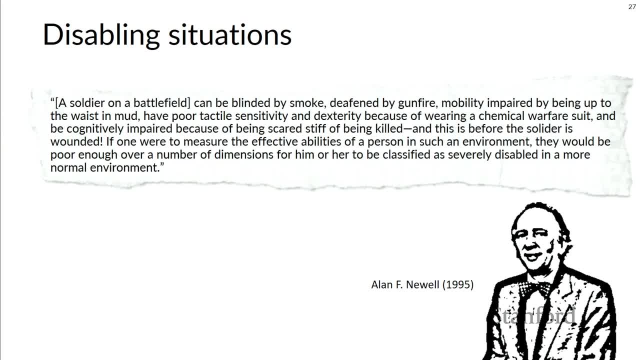 And this is before the soldier is wounded. If one were to measure the effective abilities of a person in such an environment, they would be poor enough over a number of dimensions for him or her to be classified as severely disabled in a more normal environment. 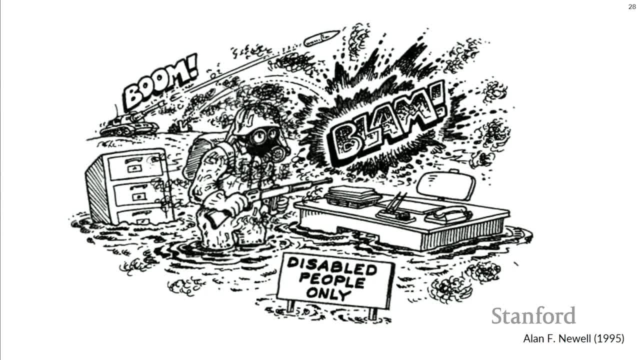 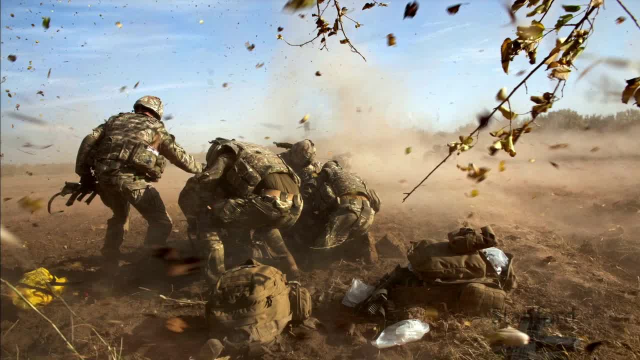 And he had this picture in his black and white, you know, hand-drawn textbook, Kind of a classic image. if you like something a little more recent. This is Newsweek's shot in Afghanistan not too long ago. Think about the abilities of these otherwise very abled- presumably abled- soldiers. 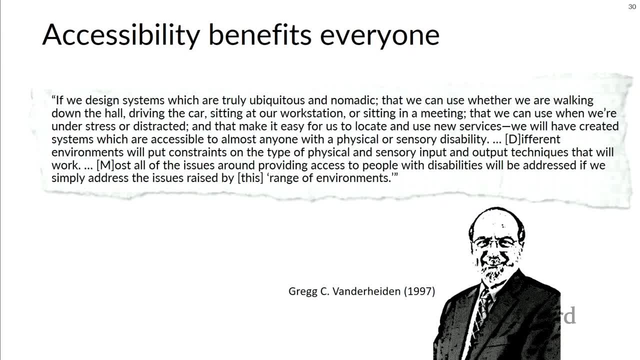 Greg van der Heiden, also a Social Impact Award winner. a little pattern here. I suppose These people have been really foundational in this kind of thinking. He talks about how accessibility benefits everyone, And that's a message we like to say, but then it's often not kind of fully lived out. 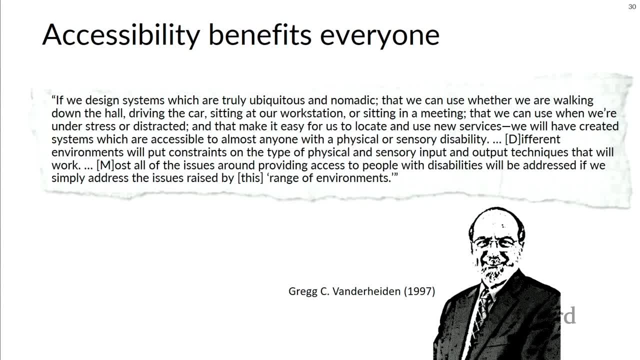 Usually people go as far as the curb cuts. example, If we have a curb cut, then it helps a 10-speed bicyclist and a person in a wheelchair and then it helps the other person And a person pushing a baby stroller. 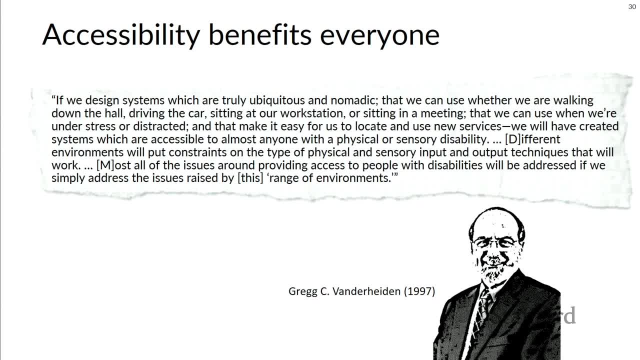 Well, that's true, And then it kind of stops. But how do we think more broadly about how accessibility can benefit anyone? If it's true we could all be impaired or disabled by situation and context as we interact, then it seems to hold that in fact this could be for all of us. 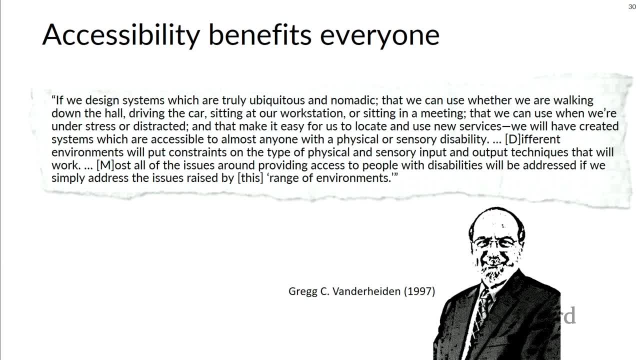 If we design systems which are truly ubiquitous and nomadic, that we can use whether we are walking down the hall, driving the car, sitting at our workstation or sitting in a meeting, that we can use when we're under stress or distracted. 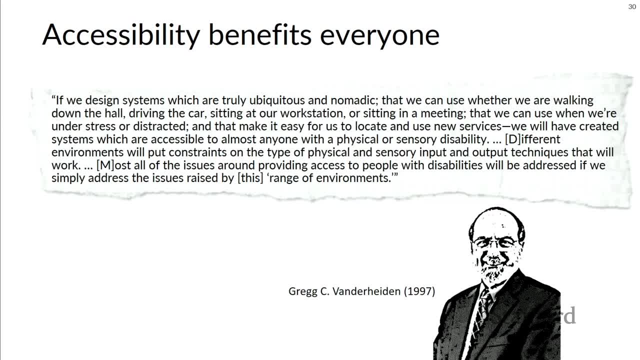 and that make it easy for us to locate and use new services. we will have created systems which are accessible to almost anyone with a physical or sensory disability. Different environments will put constraints on the type of physical and sensory input and output techniques that will work. 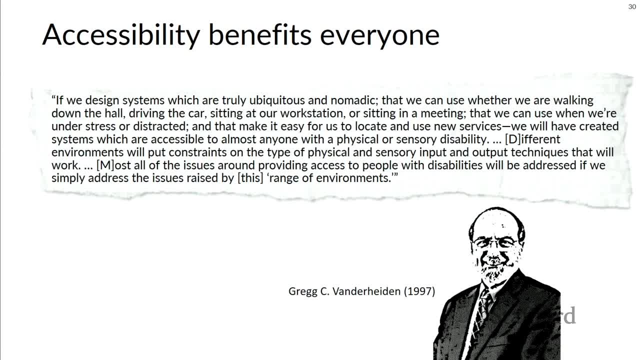 Most all of the issues around providing access to people with disabilities will be addressed if we simply address the issues raised by this range of environments. So that is kind of an agenda setting idea that we pursue these kinds of systems that allow everyone to have better access. 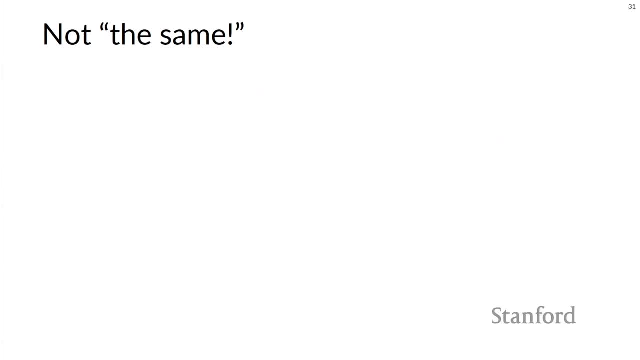 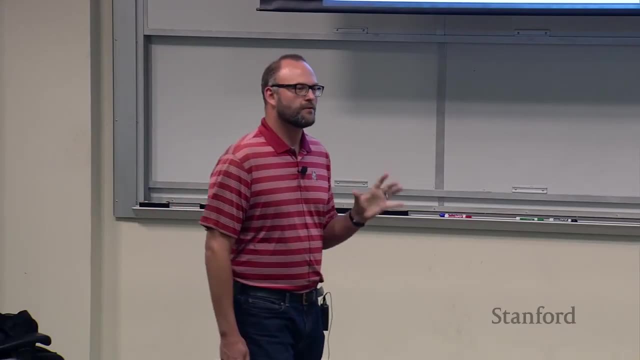 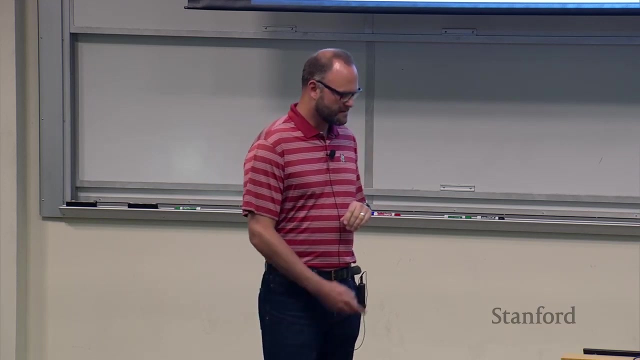 Now I want to highlight something that I touched on earlier but I wanted to come back to. There is not a claim here- and I'm certainly not making it- that situationally or environmentally induced impairments and disabilities are somehow the same as physical or functional disabilities. 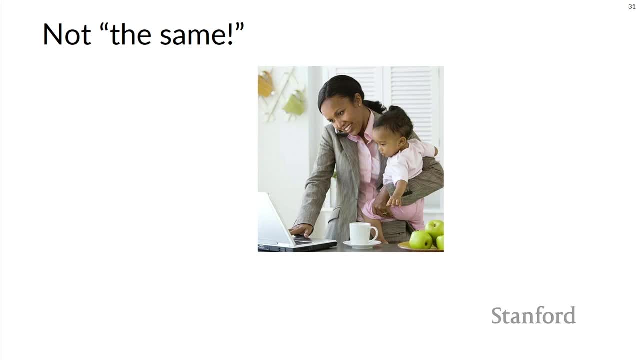 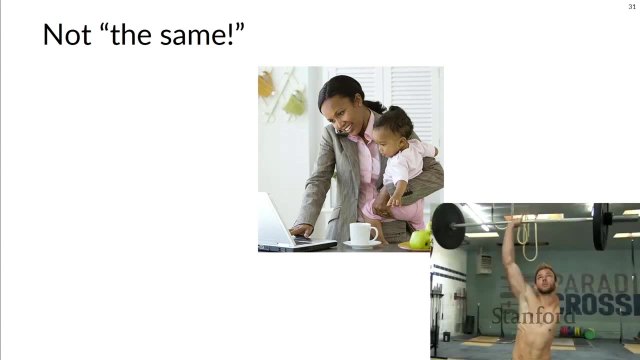 They're not the same. So, for example, a woman trying to interact one-handed with a laptop while on the phone holding a baby clearly has a lot going on. there is not experiencing the same one-handed life experience as a one-handed individual. 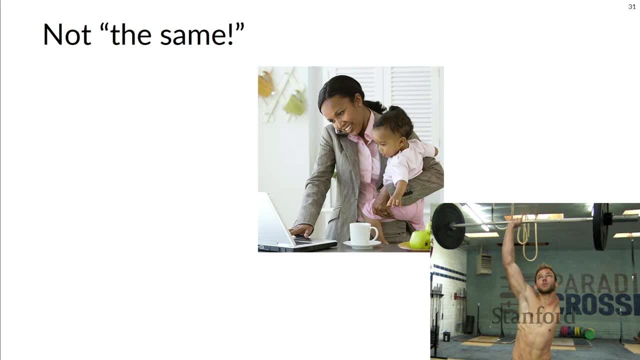 I like this photo because although this person has one arm, clearly he's very able. That's a strong individual, very fit, strong individual. So we're not saying these are the same kinds of things. There's a different lived experience. There's not stigma attached to that top image. 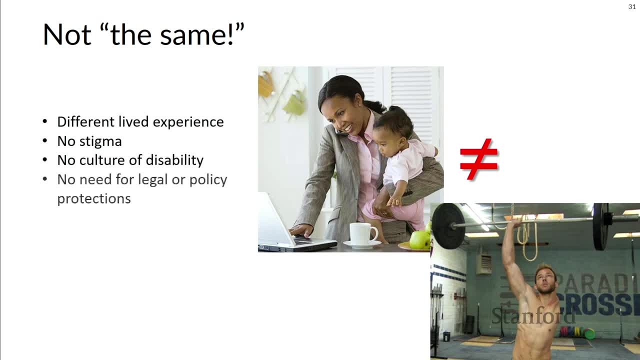 There's no culture of disability. There's no need for legal or policy protections in that upper case. But there are real impairing effects there And the key point for design is that a design that benefits a laptop design, for example, that benefits that woman in that situation, might also well benefit a one-armed individual. 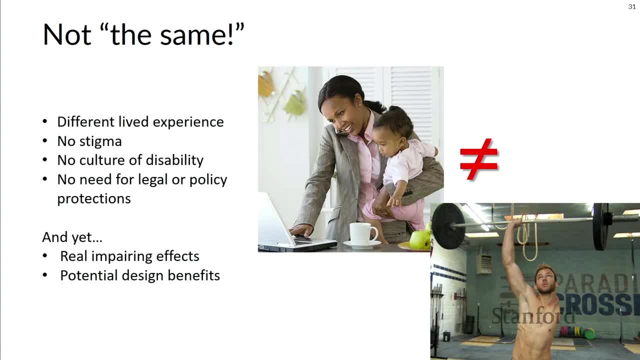 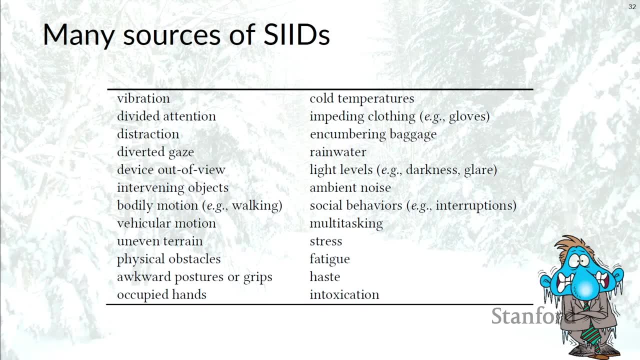 And so if we think about design for all, we can think about how we can benefit both. There are lots of potential solutions. There are lots of potential sources of situationally induced impairments and disabilities. I've listed a handful here, But I won't read them all. 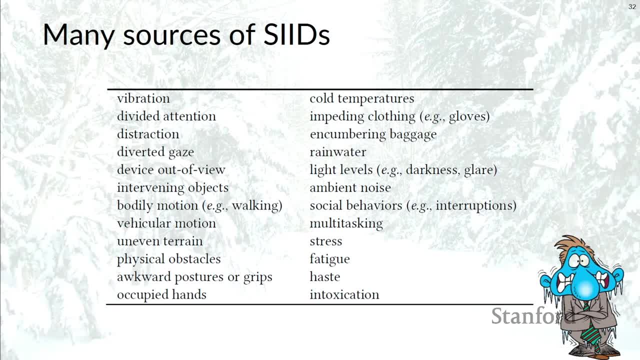 But you can see, it's not just physical or kind of motor disabilities, It's attention, It's stress, fatigue, intoxication. I'll show you a project, actually at the end, about detecting intoxication: Rainwater can impede your ability to interact, and so forth. 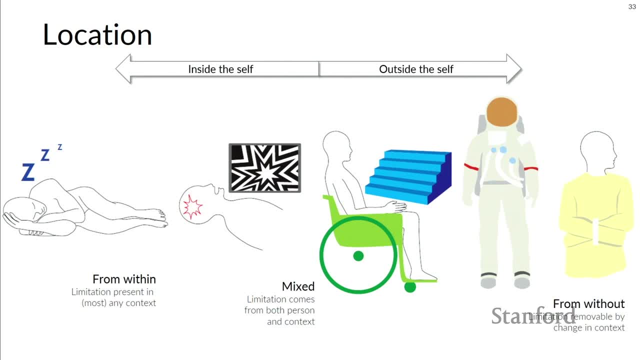 We can actually get our head around this space rather than just having like a big long list like this. If we think about two dimensions, one is location. Does the source of the impairment come from outside the self or inside the self? And it's not just a binary. 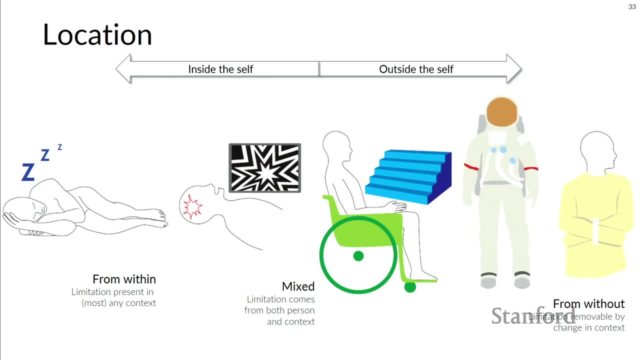 I think there's a bit of a spectrum here where there's kind of a mixed middle place. So photosensitive epilepsy, for example, is both from the light source and its pattern and the condition within the person. But I could also take someone. 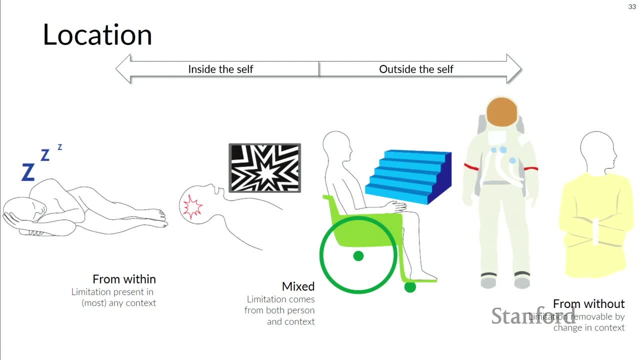 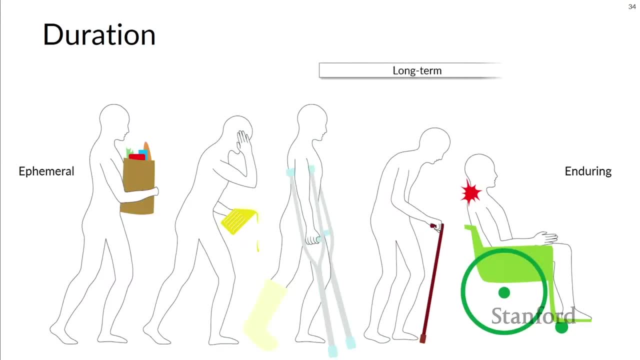 I could take the most fit active, you know, Michael Jordan, and put him in a straight jacket And although he's very able, otherwise he's not able to do much right. So that's entirely from without himself. On the other axis, 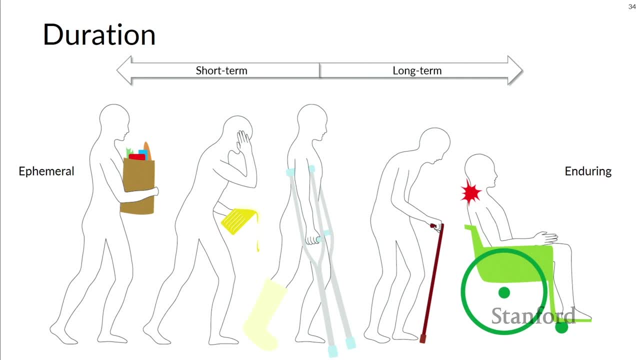 we can think about the duration. Are they kind of ephemeral? As soon as I set down the baby or the groceries, I'm no longer losing the lack of use of my arm to more enduring or even permanent, And we can then make a space. 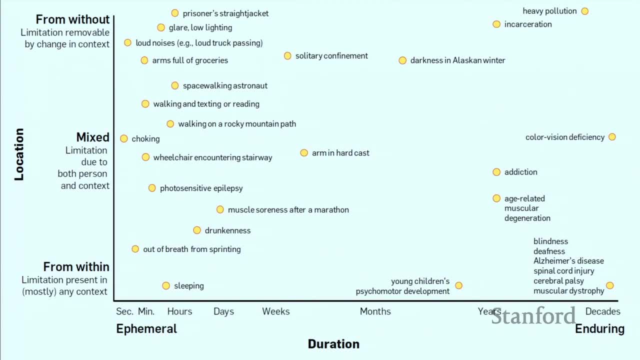 right, We like to make 2D spaces- I do at least- And we can put a whole lot of things on it which I won't read, But there are a bunch of things we could address that would enable us to interact better. 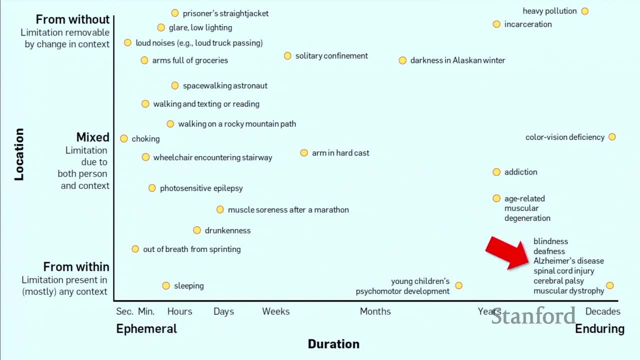 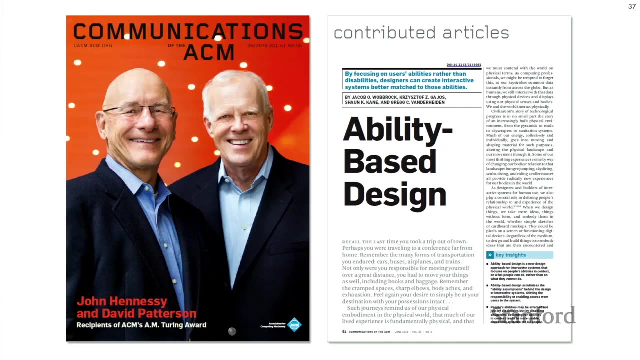 in these environments, in these situations. Most of conventional assistive technology and accessible computing has been just in this far bottom right corner, And there's a whole lot else going on here. If you want to see more, including that diagram, the communications of the ACM from last June. 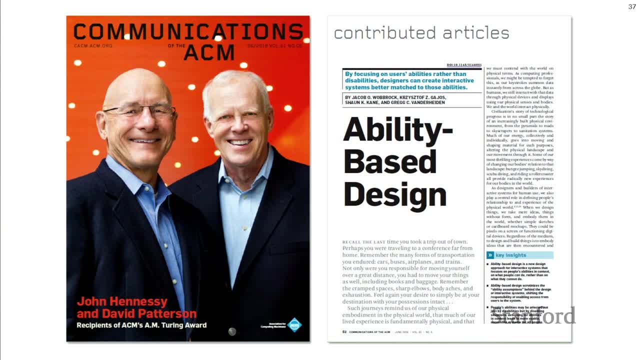 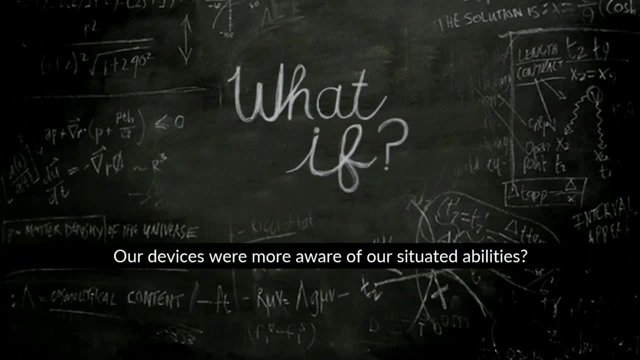 there's your own. former president and faculty member had an article of mine with some colleagues called Ability Based Design, where all these ideas are kind of laid out and put together. So let me ask you a few questions: What if? what if our devices were more aware of our situated abilities? 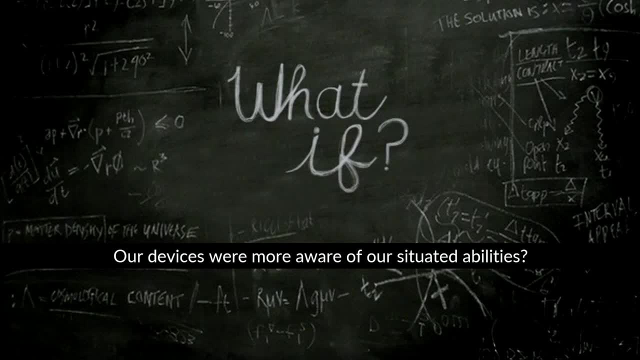 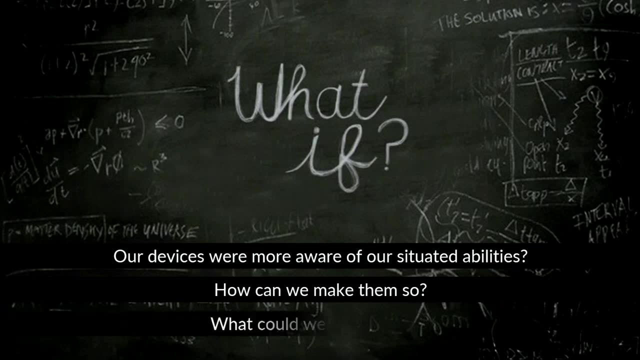 Not just our abilities but in our situations. What if, sorry, what if if they were? how could we make them so? And then, what could we do with that? All right, so there's kind of a what, how? 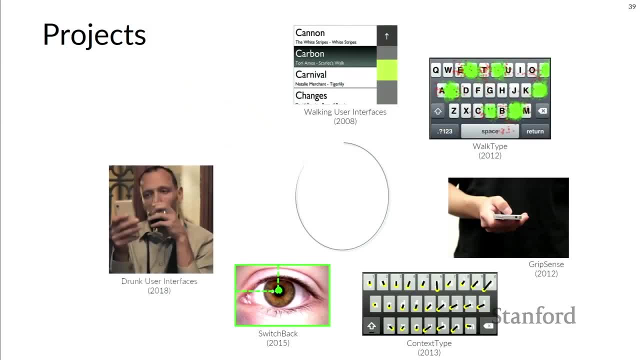 and then so I'm going to tour some projects, not all of these, But over the last ten years or so, along with multiple, many other research streams that we've done, we have pursued kind of here and there different projects that fall into this space of improving. 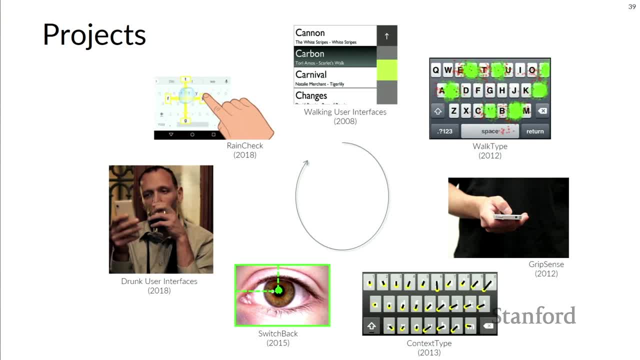 our ability to interact under situational impairments: Walking user interfaces, walk type grip sense, context type switch bag, drunk user interfaces- that's a fun one- and rain check. And I'll talk about four and I'm going to go through them at a higher level. 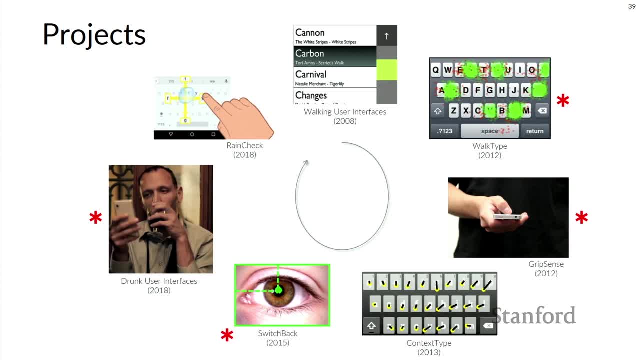 than I would if they were each their own. you know conference paper or journal paper- They all have been, but I don't have time to give that level of detail. But you can look them up very easily just by their name here and find the details in the paper. 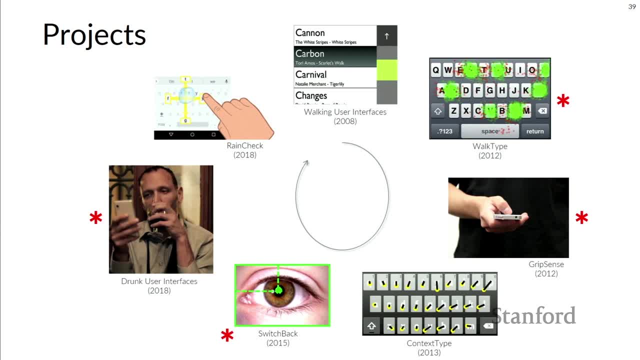 But let me give you kind of a flyover because I want to show you what's possible And one of the driving forces behind these projects is to not add additional sensors to phones. Use the onboard commercial stuff with no extra custom stuff. 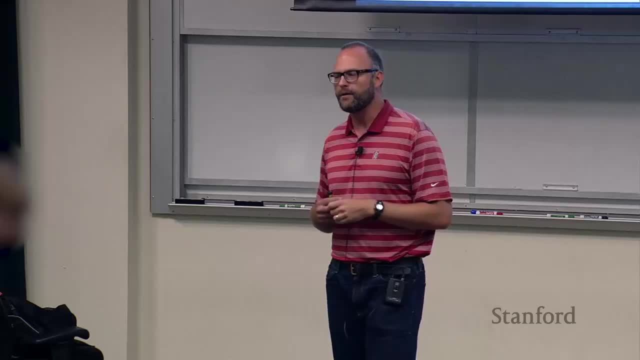 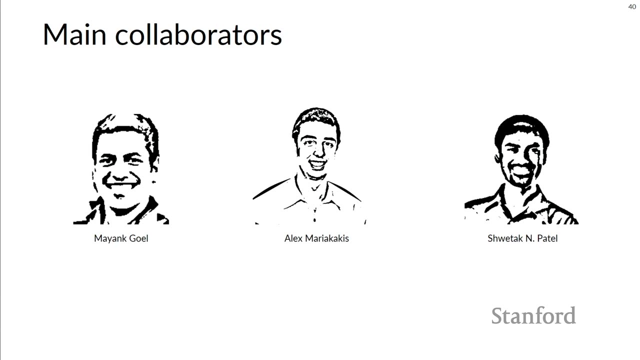 because if we do that, while that's also an interesting way to go, we limit our ability to deploy. I do want to give credit where credit is due. I've worked on the projects I'm going to talk about mainly with these folks. 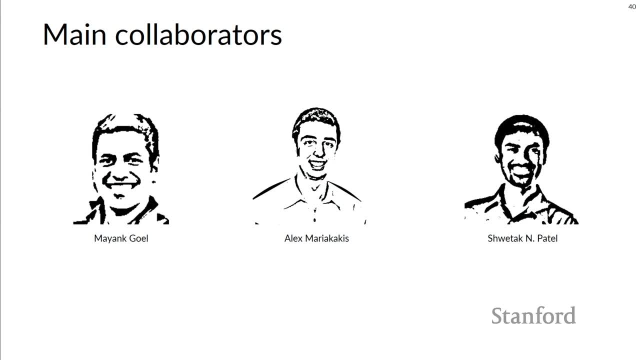 Mayank Goel, Alex Mariokakis and Shwetak Patel. Mayank is a professor at Carnegie Mellon now, having started, I think, a year or two ago. Alex is on the job market currently. He did apply to Stanford. 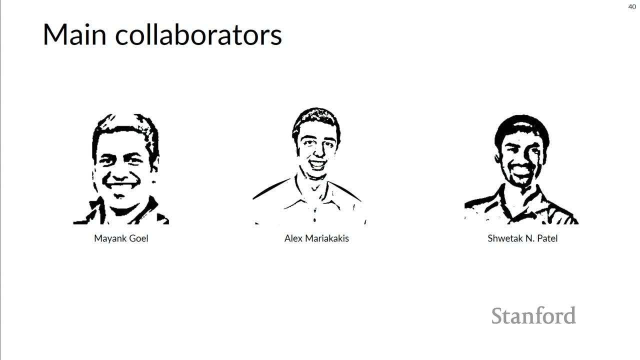 You should interview him. He's very good. I hope he does. I hope I will do him justice here. If it's not good, it's my fault. If it's great, it's his credit. And Shwetak Patel is a MacArthur Genius Award winner. 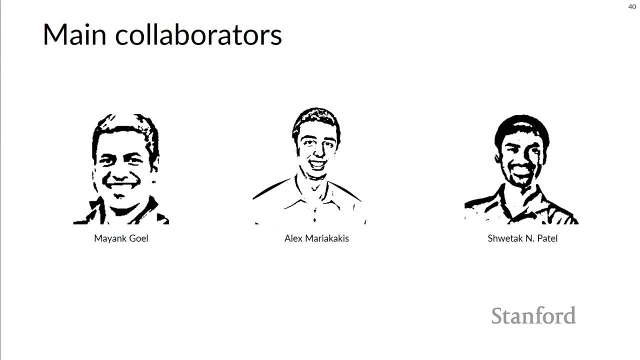 who at least the faculty in the room probably have heard of, And you're meant to interview Alex, not Shwetak. We like having him at UW, So you interview Alex, just to be clear. All right, Let's start with walk type. 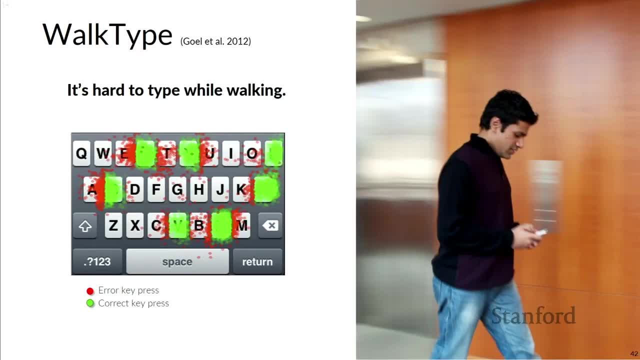 So the challenge here was- and this was back before the most advanced soft keyboards were out. This was back in the work was mainly in 2010 and 11. And the challenge was typing on a soft keyboard. and it's still the case somewhat. 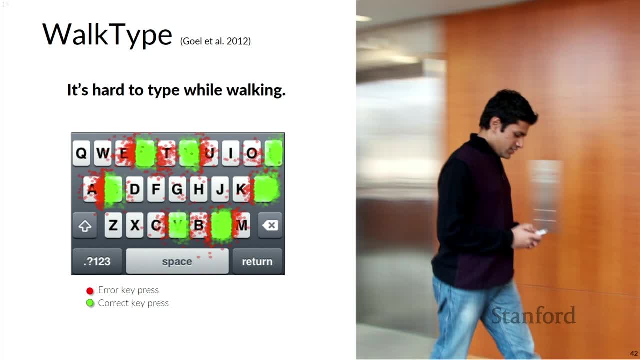 although they've gotten much better, But typing on a soft keyboard was fairly inaccurate, especially if you're actually walking. I would argue, in fact, that most of our phones are really portable devices, but I don't know if they're actually mobile. 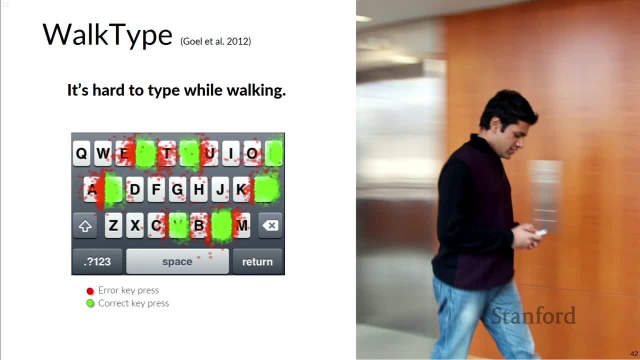 in the sense that you're using them while moving. You know, are they mobile? I don't know We could debate that, But they certainly were less mobile then And this image shows red key presses are errors and green ones are correct strikes. 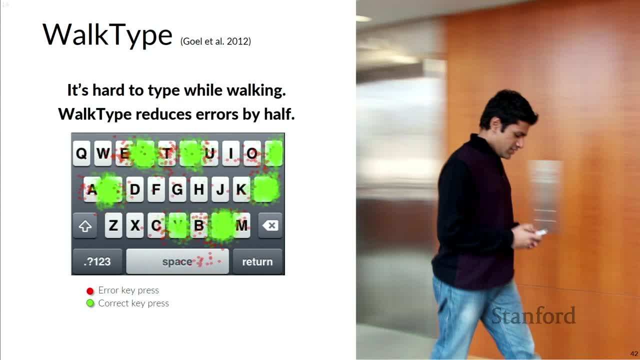 in this particular image And we can do this with it. So we can actually, through some pretty basic machine learning, reclassify these key presses while you're walking, to make them much more accurate. In fact, we can reduce errors by about half. 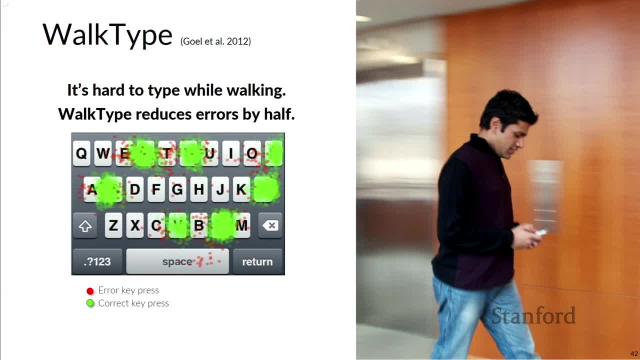 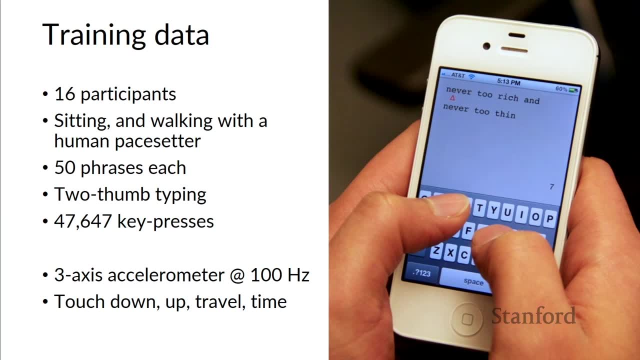 which is in text entry research. if you can cut errors by 5%, you've done something really well, And so half is a huge win. Let's go through this a little bit more. So we trained, you know, we captured training data. 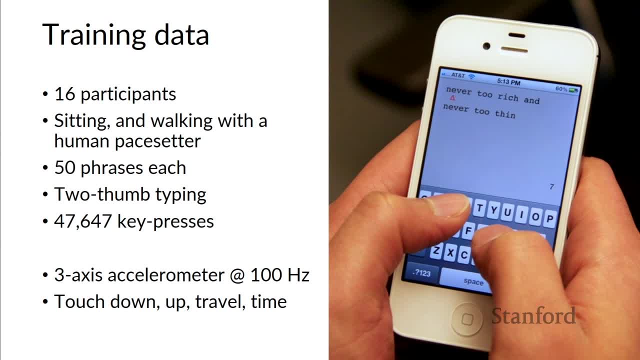 kind of a familiar pipeline here of how these projects go. We had 16 participants. They were sitting and they were walking In walking. we had to control that, so we had a human pace setter that led them at a pace. They entered 50 phrases each. 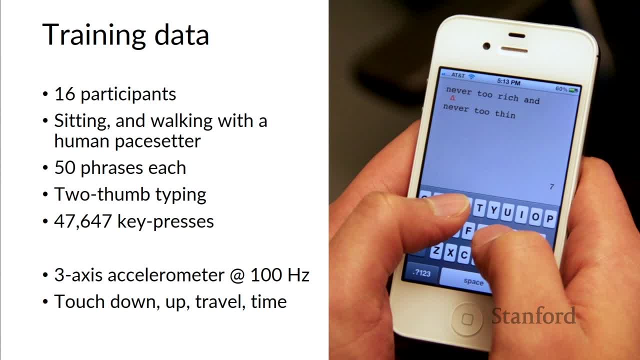 They did type with just two thumbs, so we were restricting to that posture in this case, But there's no reason this wouldn't generalize to other postures. We collected almost 50,000 key presses, so there's a fair bit of low-level data here. 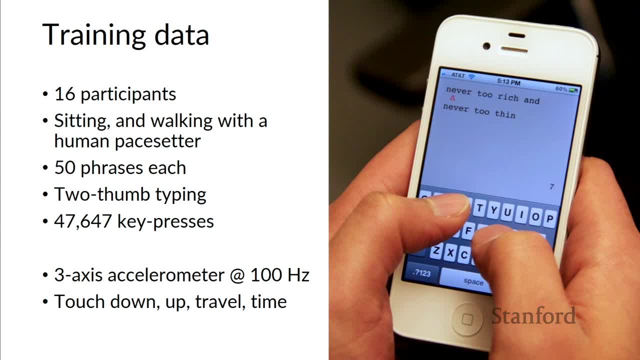 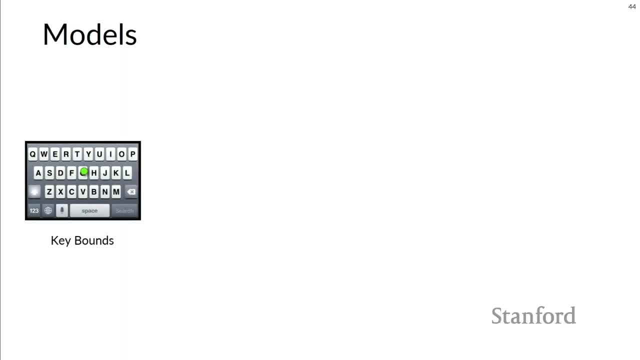 We also collected three-axis accelerometer data and touch events, so up down travel duration, so on, And we built some models. So the simplest first model we built we call the key balance model, which is simply just a baseline model of. 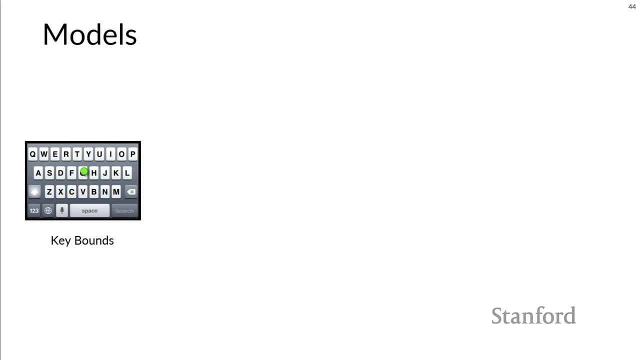 if you're in the key boundary it's a hit and if you're off, it's a miss. And we know that because we've issued the sentences they're typing and we can figure out the character-level error rates And even just with touch down. 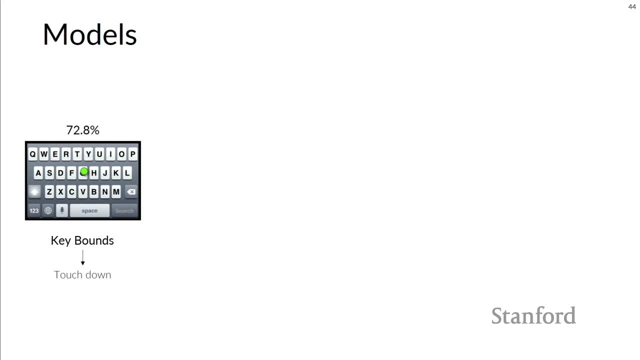 the baseline here gives us a 72% tenfold cross-validation classification accuracy. Okay, now let's do something more interesting. But that's kind of what we're comparing to right. That's sort of the most basic, If we add those other touch events to the model. 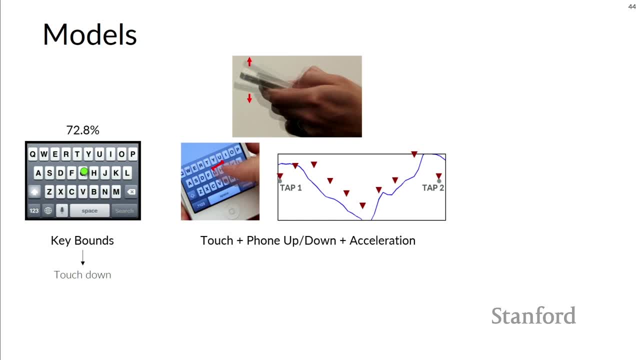 we also noticed that people when hitting the phone- we looked at some high-res video in slow motion- The key presses make the phone go up and down in the z-axis quite a lot, So we suspected that might matter a great deal. And then we also thought: well, 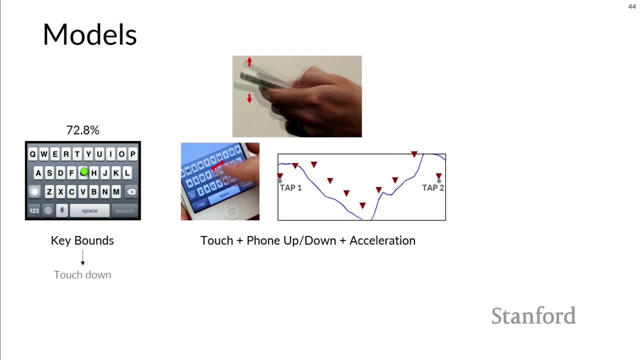 general motion of the phone is also something to capture. So let's capture acceleration in all three axes. And so we grab more touch events. You can see those there. We grab the vertical direction at each tap when a tap happens. We also double integrate to get 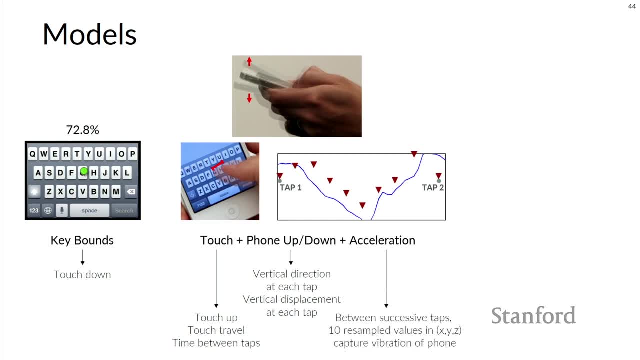 the vertical displacement of the phone And then we also get the acceleration between successive taps. We resample that to get some finer data points within it And that gives us the overall vibration, essentially, of the phone And that brings us to 94.6% in our accuracy. 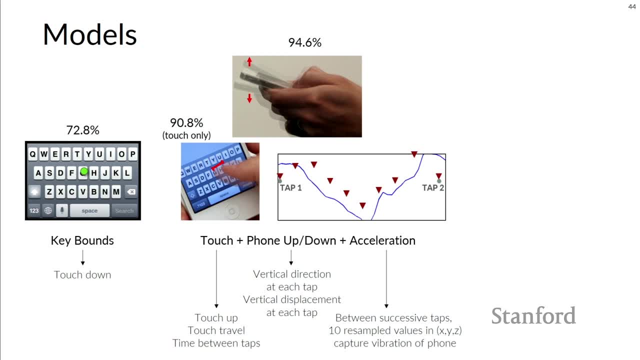 which seems better, obviously, If we take out the acceleration features and just do the touch features. just in case you're curious, touch only would bring us those other touch events, bring us to 90.. Okay, now here's the fun part. 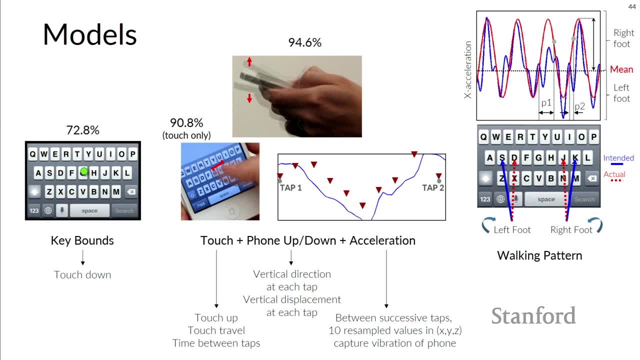 Actually we could figure out which foot's hitting the ground, And we didn't believe we could do that, but we figured out we could. It was kind of a surprise to us too. The idea was that if we look at the x-axis, 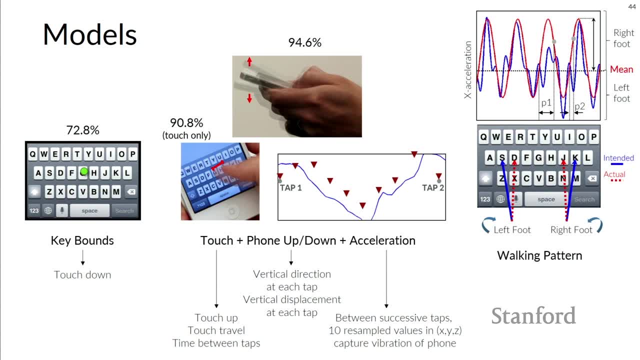 which is the side motion, there's a systematic inward rotation of the device. just enough, as you step- I'm exaggerating that- we could detect that- And it causes an inward rotation of the corresponding thumb. So people are systematically slightly inside their intended target. 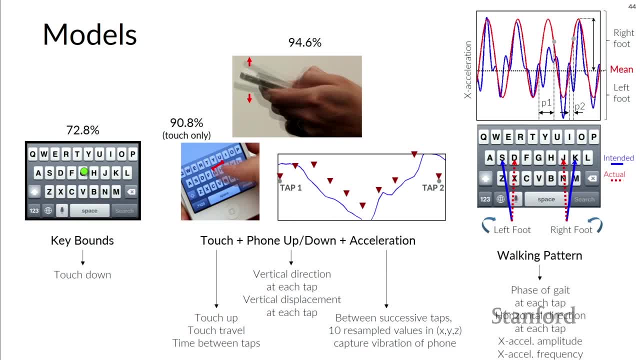 And because of that we can develop a phase of gait model where we know which foot is moving forward at each tap. If you're above the mean line, essentially it's the right foot. If you're below the moving mean, it's the left. 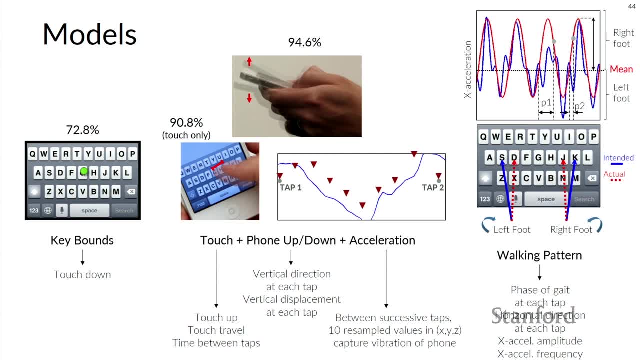 And then we also know the x-axis. you know information as well. So when we combine all that together, we actually go up a little bit more as well. That's just kind of fun to think that you could actually tell which foot is moving forward. 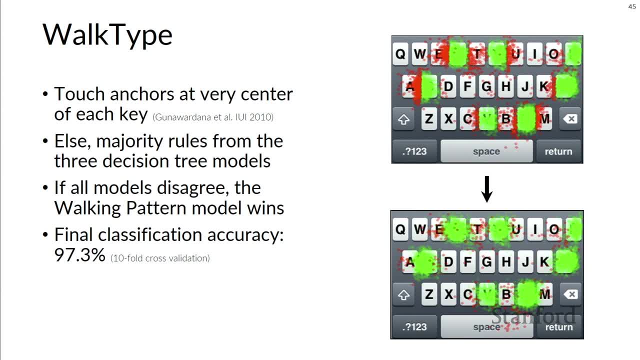 So the final walk type model worked as follows. There's a concept we did not come up with- It's a simple one but it's important- called touch anchors. You have a space at the center of the key where you just declare: they must have meant this key. 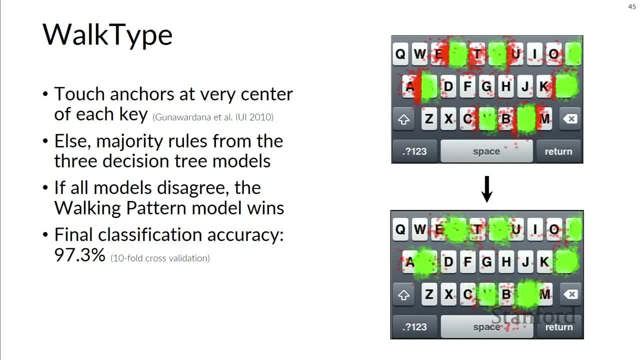 because they're so dead in the middle, And it was about 20% of the key width in, I think, in x and 50% in y. But if they miss the touch anchor, which happens a lot, then majority rules from the three models. 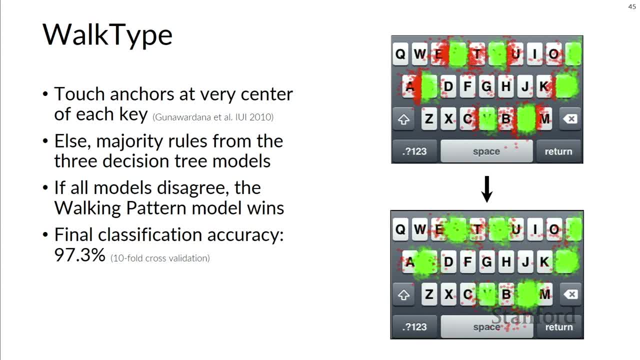 you just saw, if they all disagree, the walking pattern model wins because it was most accurate And our final classification accuracy with this approach was 97.3%, which allows us to correct a lot of those misses. But then we have to evaluate it right. 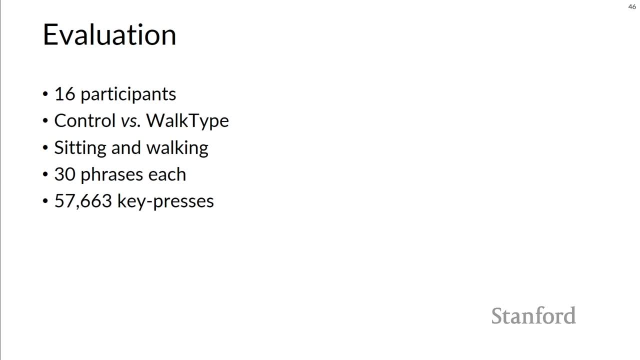 We're not just doing the offline evaluation. So in an interactive study where participants were blinded to whether or not they were using the walk type or the regular keyboard, they were sitting and walking. There were 16 of them. They entered 30 phrases each. 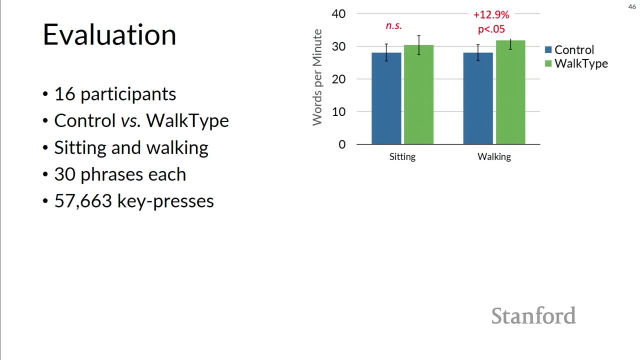 about 60,000 key presses And we see that with sitting there's no significant difference in their words per minute for entry speed, But while walking they were actually about 13% faster. That's nice. We were mostly focused on accuracy. 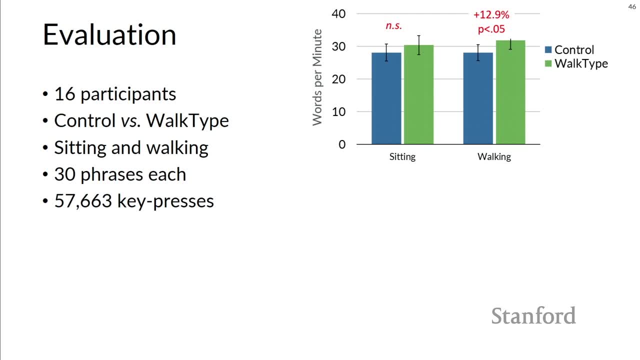 But if you're more accurate, you're also probably going to be a little faster because there's less error correction And that's where we see. with sitting there was a reduction in error rate. that's fairly considerable, but it's almost 50% with walking. 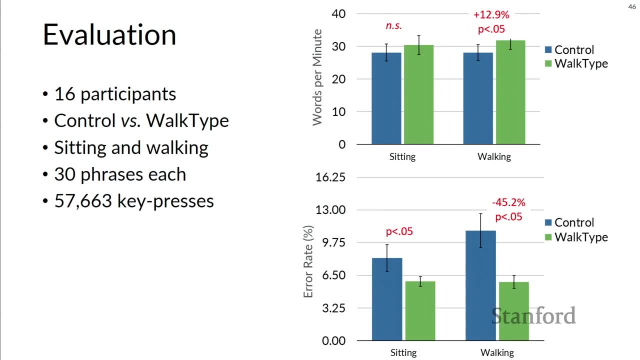 So we seem to have one of those nice results where we're not hurting anything and we're only helping, if anything at all. Also, 14 out of 16 participants, when asked which of the two conditions which they didn't know, because there's no visual difference. 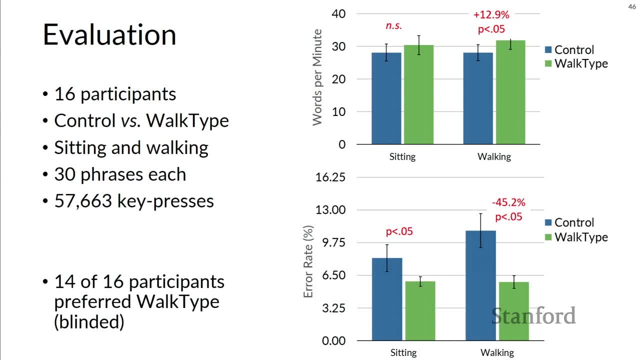 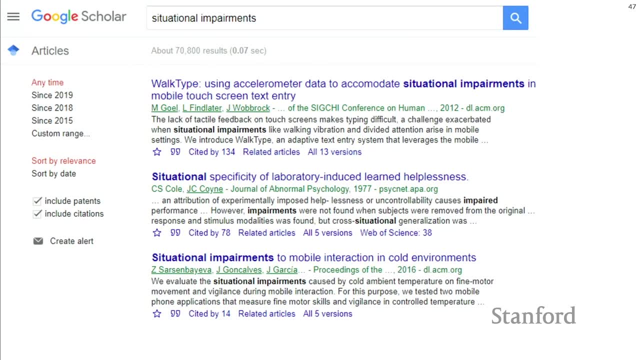 they preferred 14 of 16 preferred walk type it turned out. So that's kind of nice. If you type situational impairments into Google, Scholar walk type's the first paper to come up, So it's easy to find and it's kind of fun for us to see. 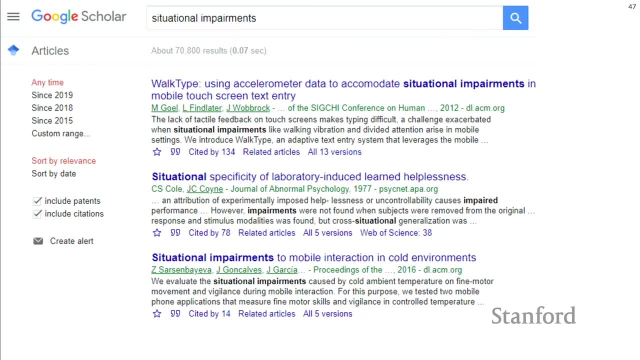 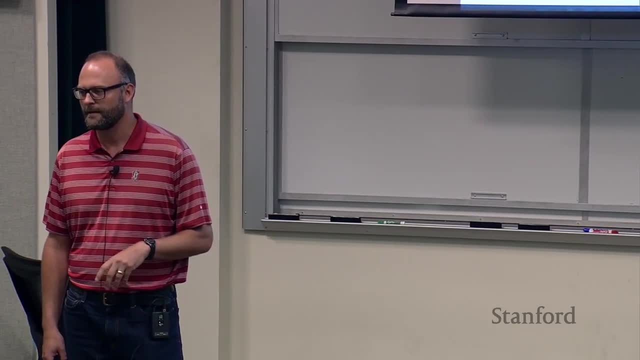 that it's become associated with that. Yeah, sorry, Did you try to train an NLP model, Because it seems like the letters just were kind of the neighboring letters. So how did that compare? Yeah, so no, because you could add language models. 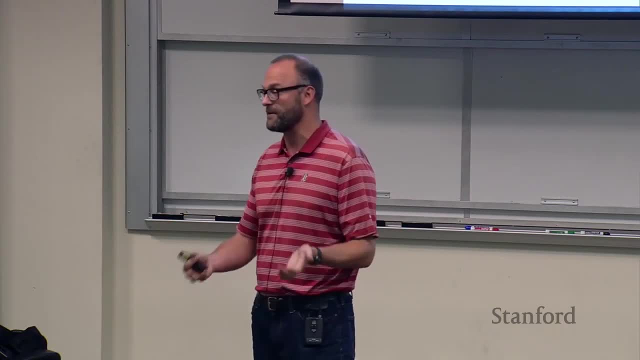 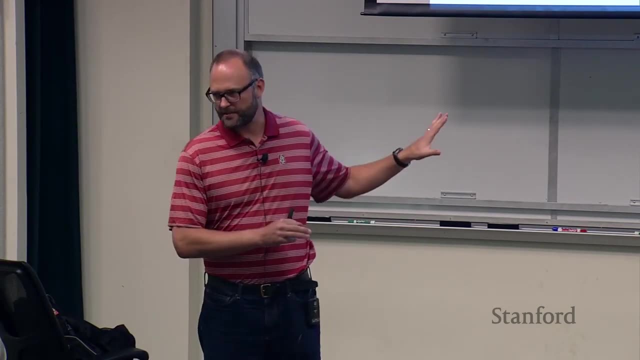 and stuff on top of these keyboards till the cows come home And modern keyboards now do much more of that than back then, But that would actually just make it harder to see the difference from the touch-based stuff, So we wanted to keep those concerns out. 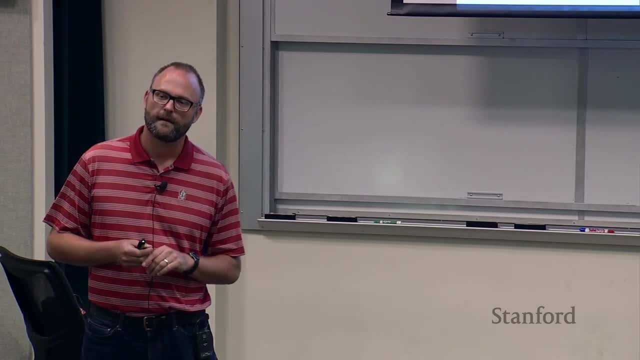 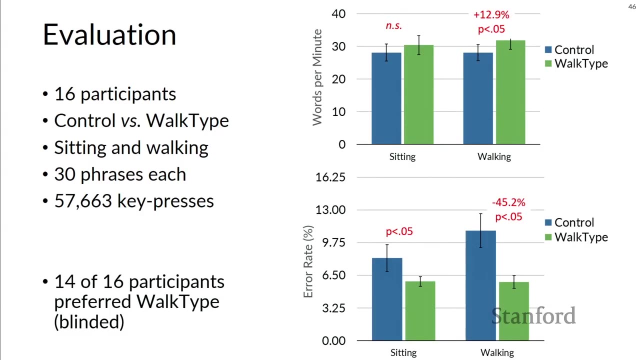 Yeah, Is there a reduction in the error rates in the sitting condition, Because your model wasn't optimized for that Right, I'm not sure. I don't know. We'll take it though. I might have known then It might. 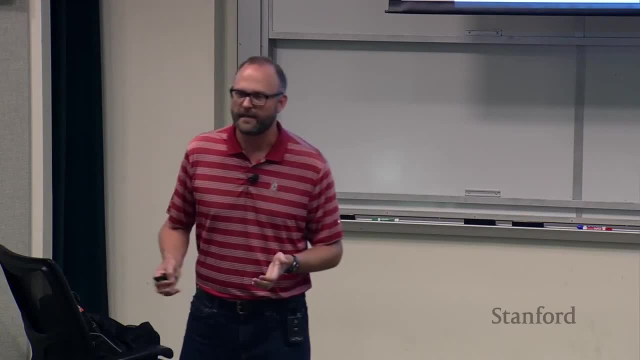 I mean you're still, yeah, you're still moving while sitting. I mean not as much, right, But you're still moving. So there's still the z-axis pressure and so on. I'll take one more, and then I want to keep moving. 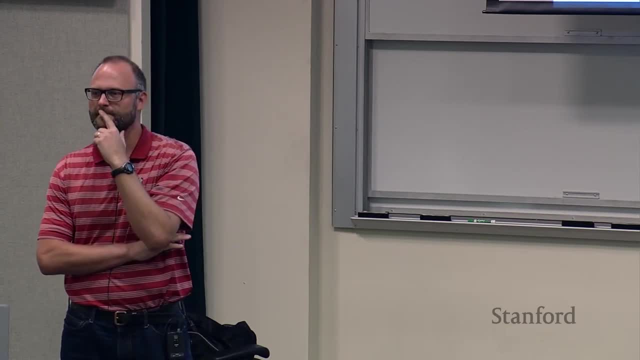 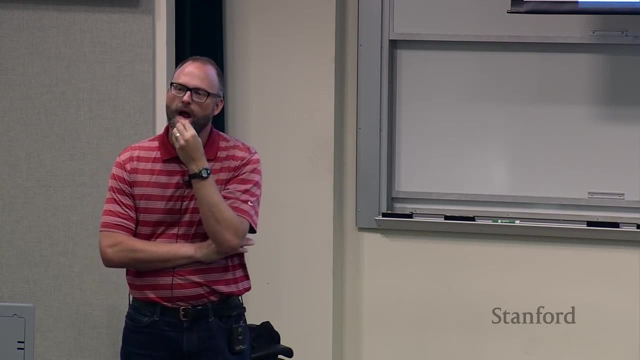 so we get through the other ones, Yeah, Yeah. So what about the comparison to voice? Yeah, You know, to handle a situational impairment, you might consider using voice, You might. yeah, I think you guys have shown it. 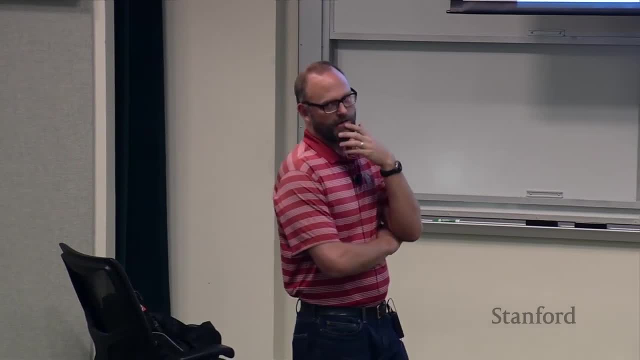 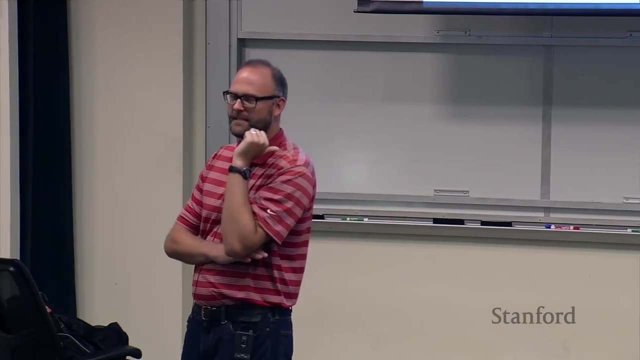 Right, Much more recently, yeah, Yeah, So voice back then was not like the Deep Speech 2 engine we used- we being James, and I and others used in our recent paper that I think you're referring to: Voice has, so voice has. 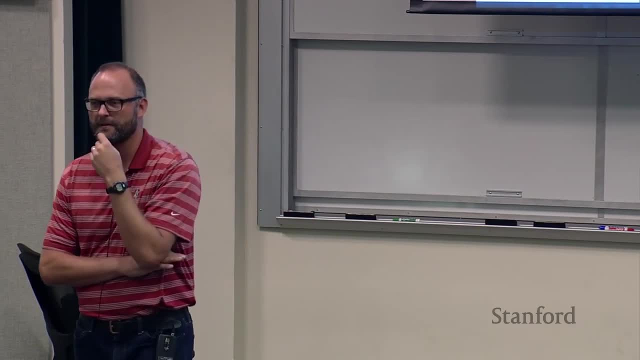 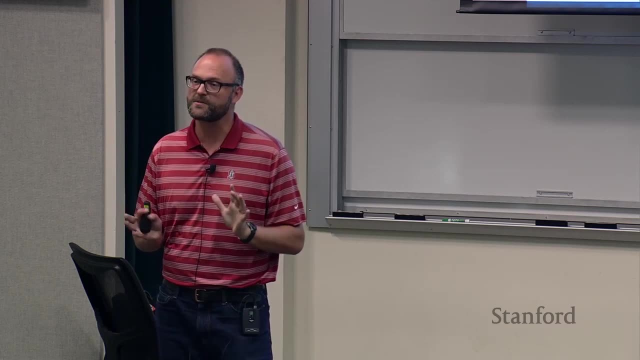 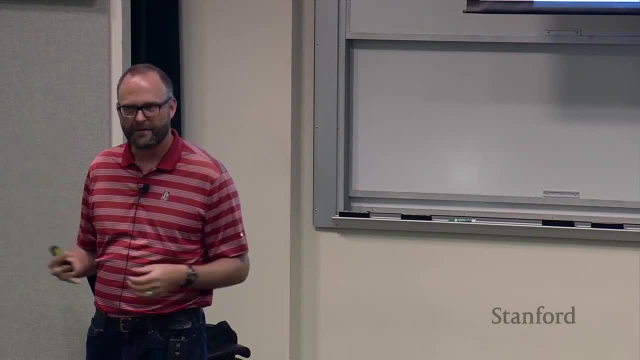 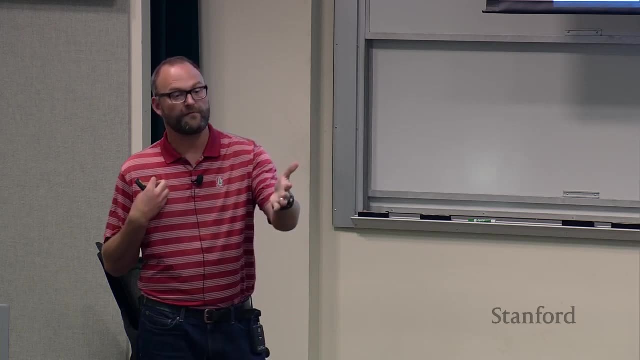 you know, situational impairments, But it it is certainly not the silver bullet because of all sorts of other factors like privacy, social issues, ambient noise, I mean they're just kind of apples and oranges, So I don't think. 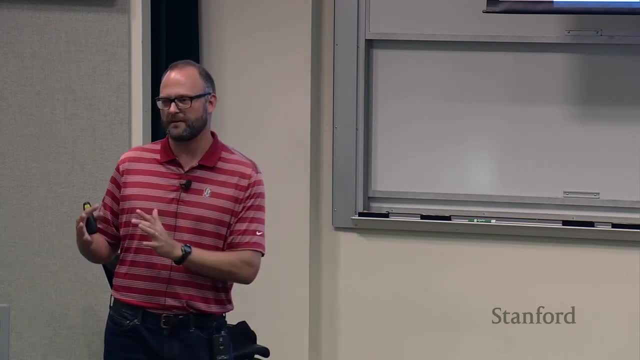 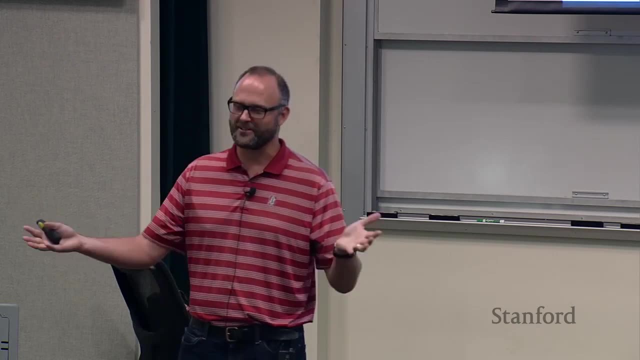 I'm certainly not and and we've never claimed, for example, that voice kind of means the soft keyboard on a smartphone is dead Right And and actually clearly it's not. In fact, right now it's not appropriate. 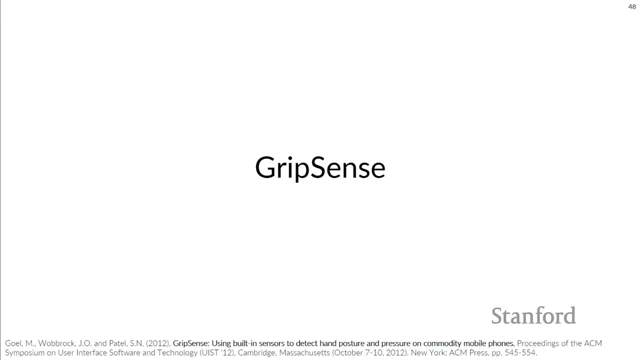 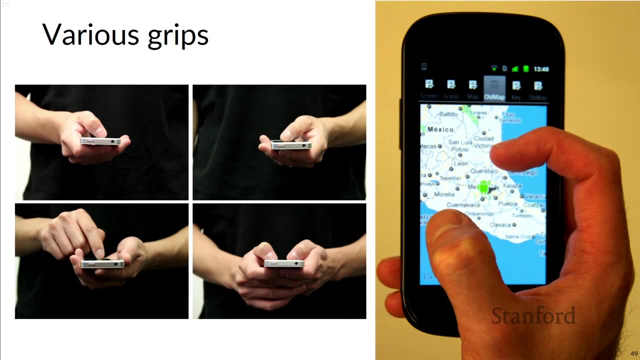 So I think it's a both, a both thing, you know. Okay, We'll go through GripSense quickly here. Let's see Watching the time a little bit. So this project was about trying to understand, just having a device know just this. 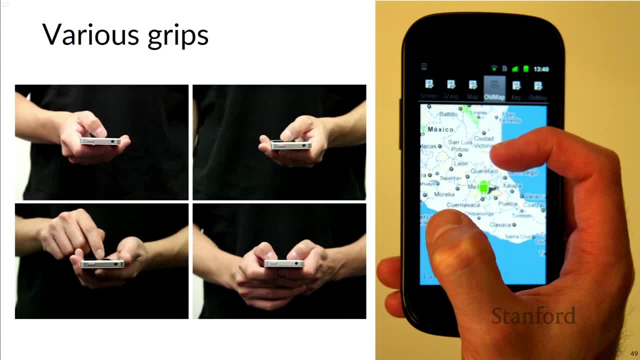 which is: how are you holding it? Just that much context about the user Right. Are you holding it in your right or left hand, two handed or interacting with an index finger? because you're holding it in an off hand Also. 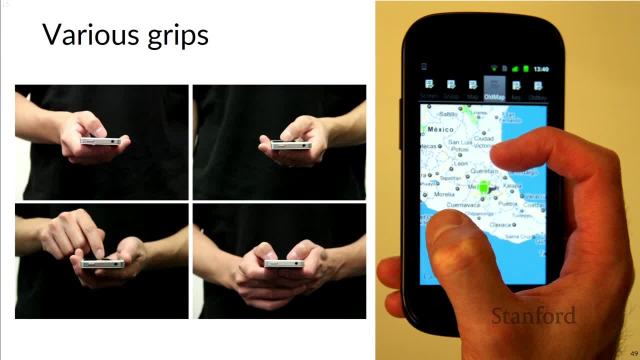 this for zooming in and out stinks. This is the one handed version of pinch to zoom. We've all done it, but it's no good Right. Why have you done it? Because your other hand or arm was busy. 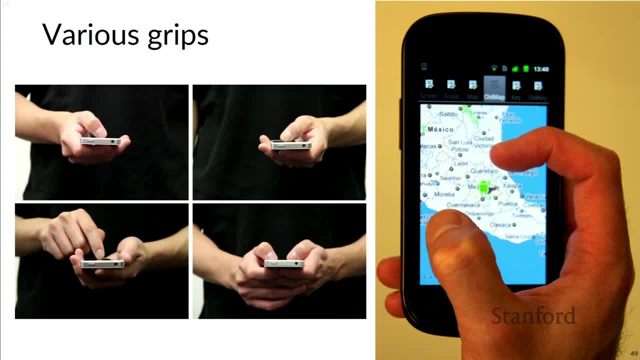 Or you were holding. you know you were holding on on the bus so you don't fall over or whatever. So there are times when we've all done that. I know you have. I won't ask for hands, But 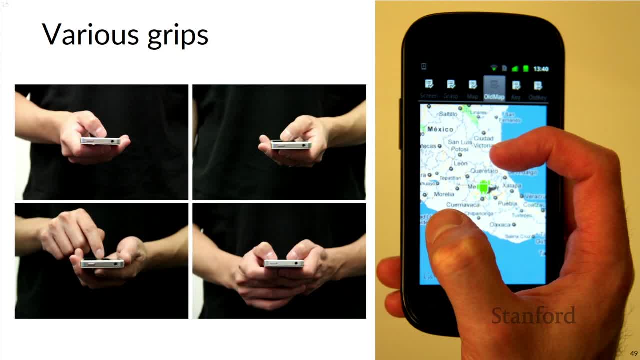 that's no, not a good experience. It's usually quite inaccurate, and so on. So you can do a one handed zoom with one finger, based on pressure, without a pressure sensing screen? And the answer is yes, And I'll just preview what we did. 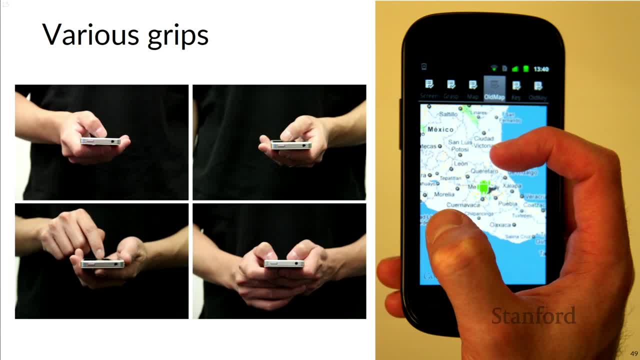 We actually pulse, as often happens with some vibrotactile feedback. we pulse the vibration motor when you press on the screen in an app where that would be relevant, And if you're pressing lightly it zooms out, And if you're pressing hard, 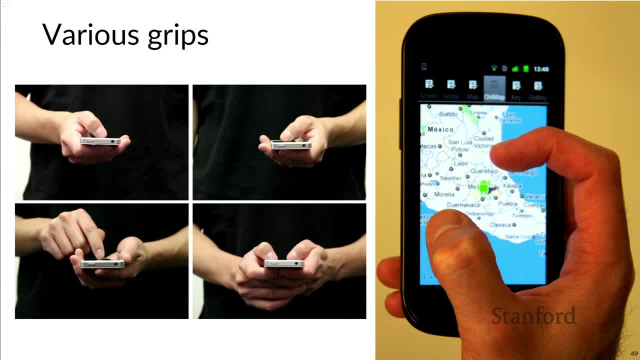 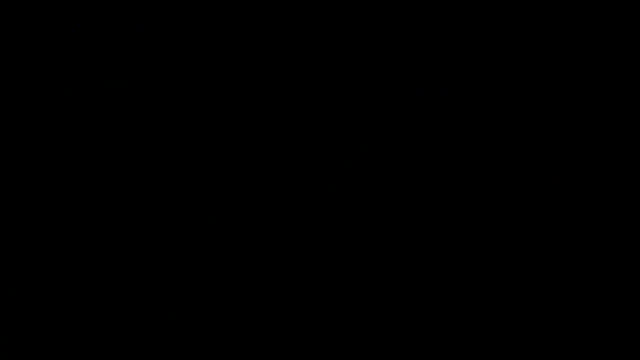 it zooms in. It actually feels pretty good. And we can tell because the gyroscope signal is dampened when you're pressing harder, So your pressure dampens the signal and so we know you're pressing hard. So it's kind of a straight forward. 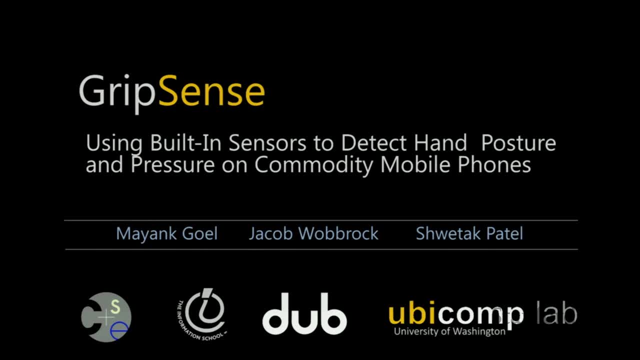 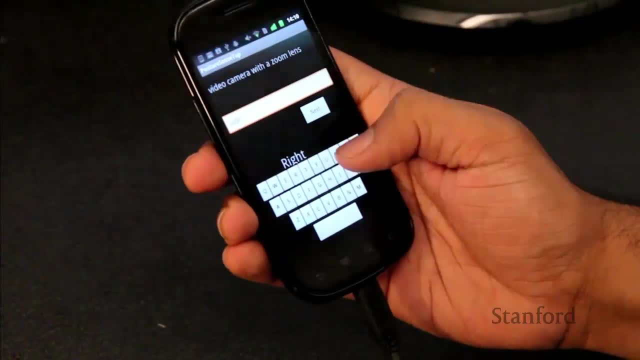 I won't play the whole video, but let's take a look for a moment here To infer user's postures, like whether the device is on a flat surface or being handled with an index finger or left or right thumb. It can also sense the amount of pressure. 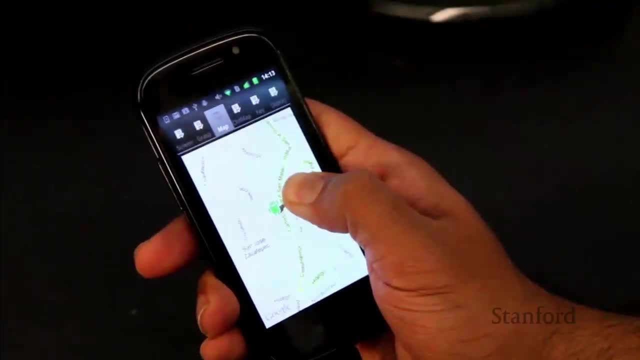 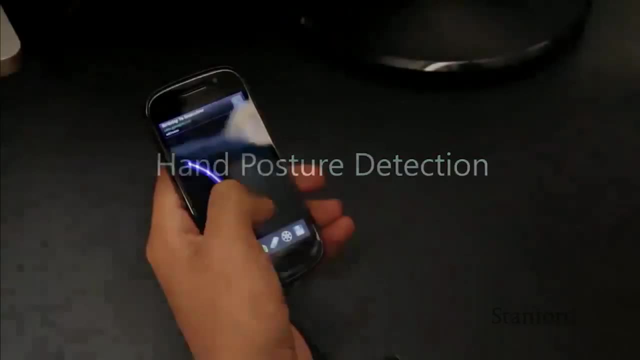 a user exerts on the touch screen without adding any new sensors to the device. There's the zoom. Users handle their devices in a number of grips. GripSense combines a number of phenomena to detect hand posture Because of the shape and position of the thumb. 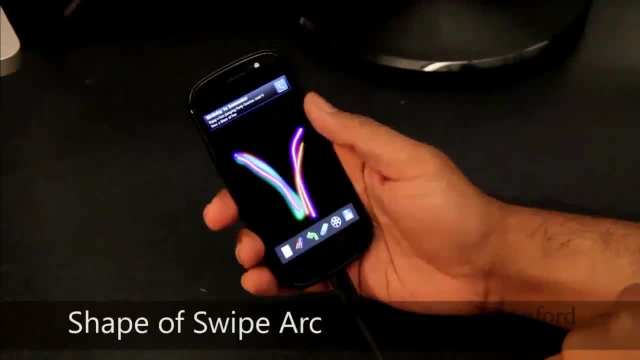 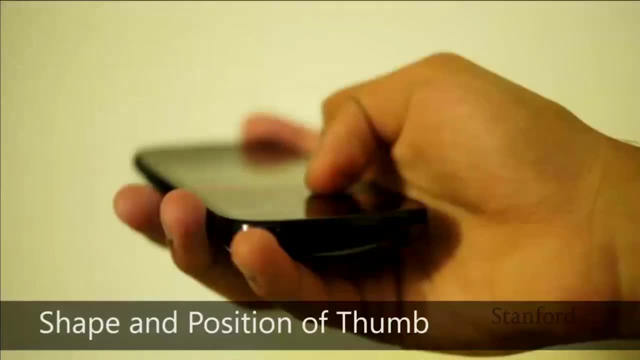 users often draw an arc when using their thumbs. These arcs have distinctly different shapes for both thumbs. However, while using index finger, there is no such arc Shape and position of the thumb also leads to different touch sizes when we touch different areas of the screen. 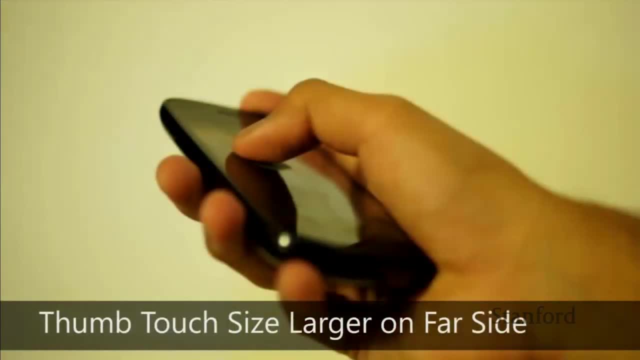 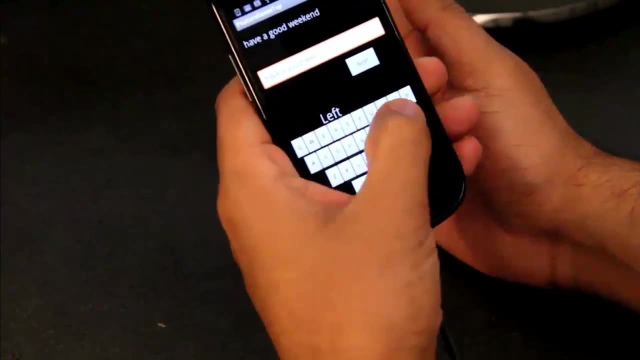 in different grips, The touch size on the same side as the thumb will be smaller than the touch size on the far side. Combining these phenomena together leads to a robust grip detection system. You can see there's a little delay between when it updates. 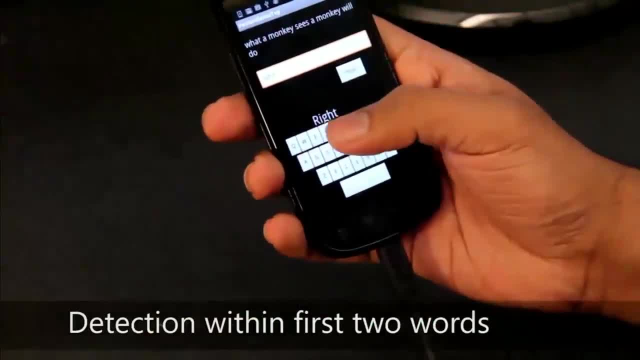 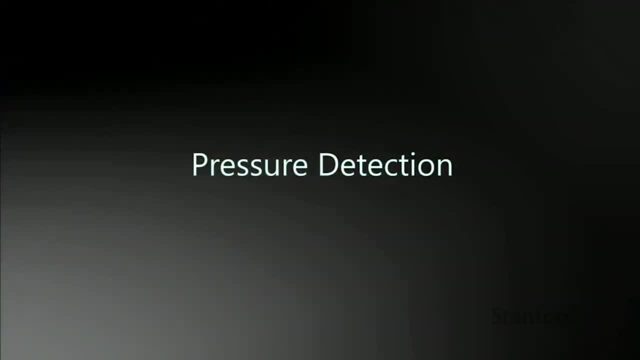 You'll switch hands and it'll say right, but it takes about five interaction steps. This means posture is detected before the user even completes two words while typing. GripSense uses a novel combination of gyroscope and vibration motor to infer pressure applied on the screen. 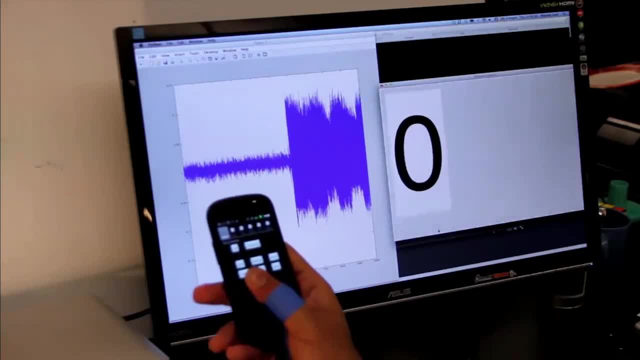 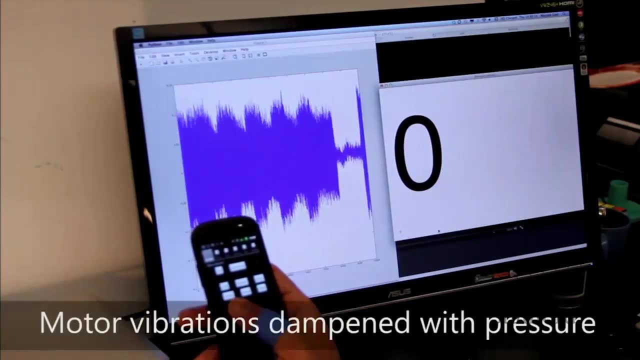 We trigger the vibration motor when a user touches the screen. Here on the right you can see the pressure values derived from a pressure sensor and on the left you can see the vibration information of the device. It is evident that the vibration of the device decreases with increase in pressure. 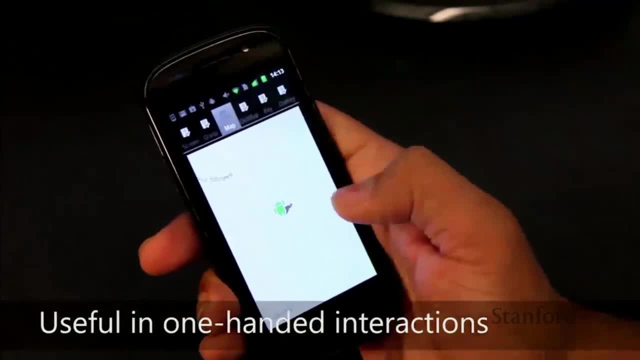 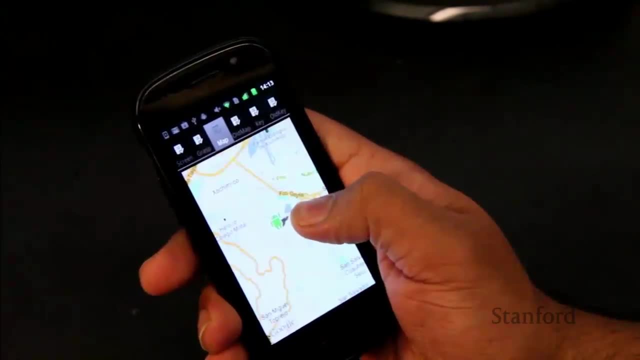 While using devices with one hand, users often feel the need for a robust and intuitive alternate input method. Here users zoom into a map by pressing hard, and light touch helps the user zoom out. This can be useful in a number of postures and situations. 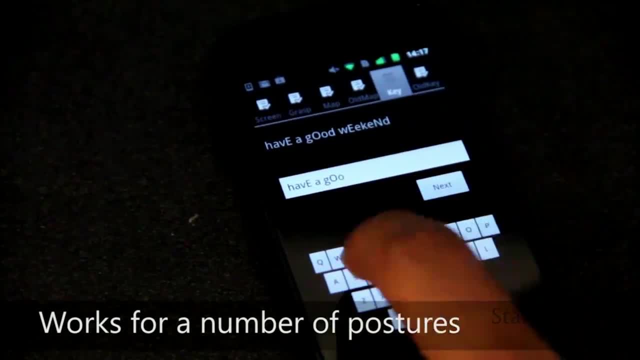 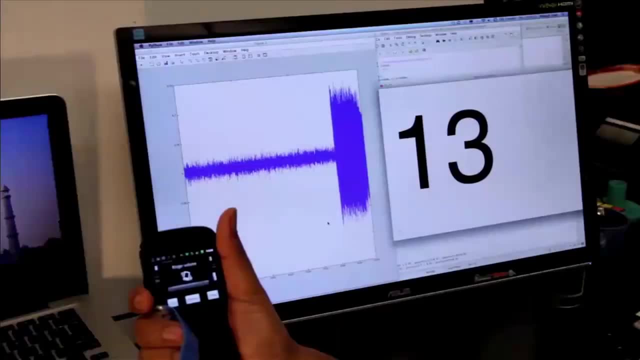 Here GripSense is used on a table to toggle between lower and upper case. User presses hard to enter upper case letters, whereas less pressure is used to enter lower case letters. Using similar techniques of pressure detection, GripSense also infers pressure exerted on the body of the device. 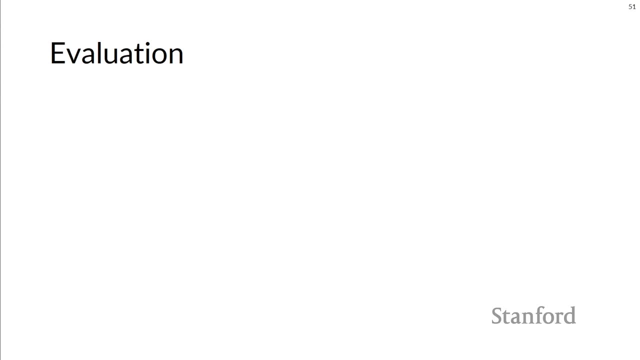 Okay, we'll stop there. So, essentially, we're leveraging features from the motion of the swipes and the tap size, essentially, and also, in the case of pressure, the dampening of the gyroscope signal. So, in an evaluation of both of these capabilities, with grip detection, 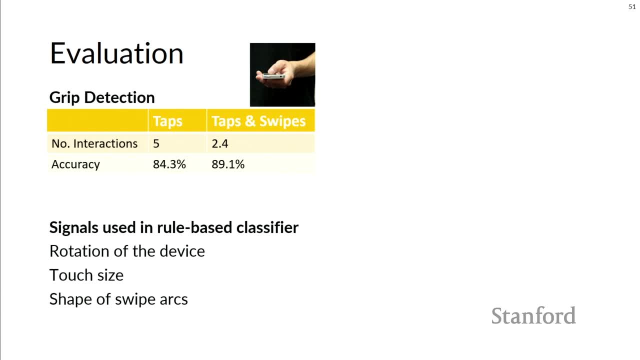 we saw that with about five taps. if we limited it only to tapping like on a keyboard, for example, we could be about 84% accurate with which hand is gripping the device. If we allow swipes into that, we can bring that down to 2.4 interactions. 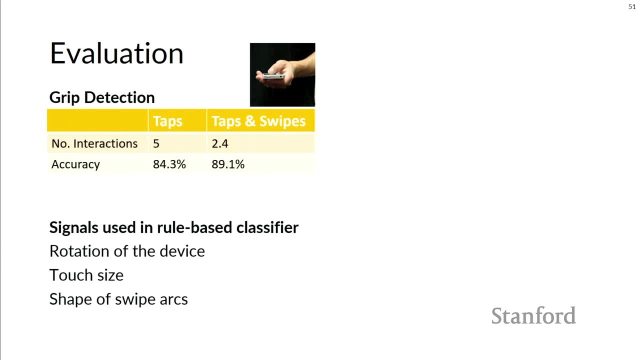 and increase the accuracy, because swipes give so much more signal, And we're doing this based on, like you saw, the rotation of the device, which is from the gyroscope, the touch size and the shape of the swipe arcs in the case where we're using those. 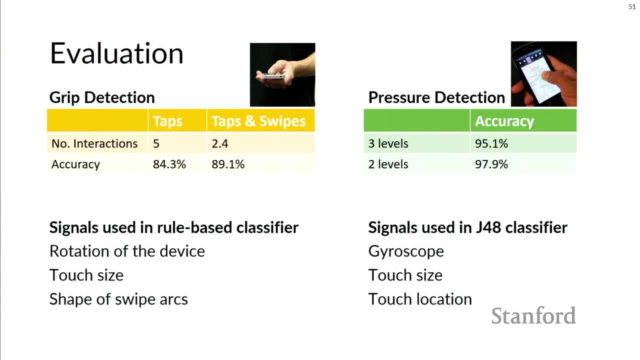 For pressure detection. if we want three levels of pressure distinction- this is through a decision tree- then we can do about 95% accurate. If we only want two, we can go up to about almost 98. And we're also here using the gyroscope. 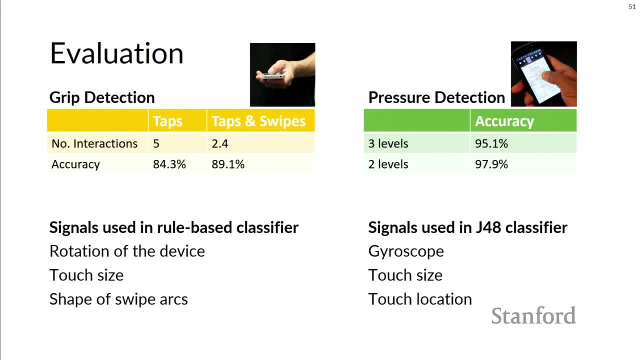 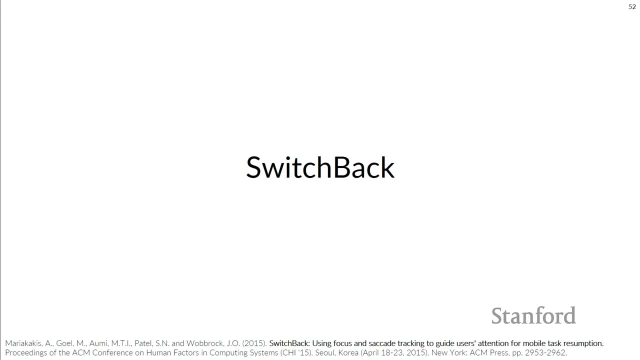 as you saw in the video, touch size and the touch location. So relatively simple models, but they can give information to the phone that it normally doesn't have. I'll make sure to finish with some time for questions so you can ask them then. Switchback changes things from the input side. 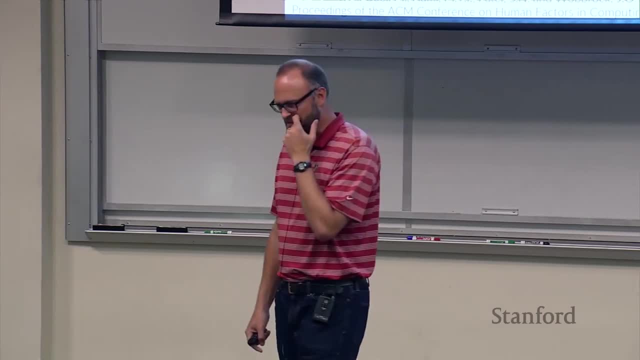 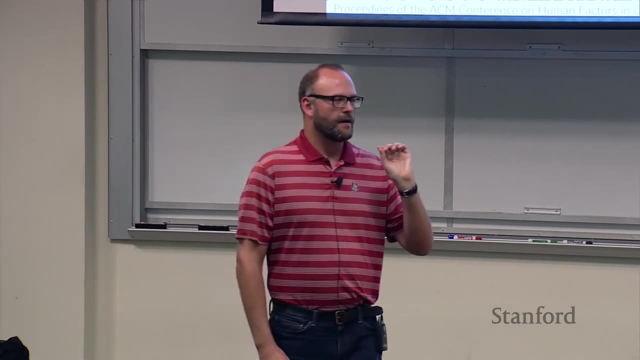 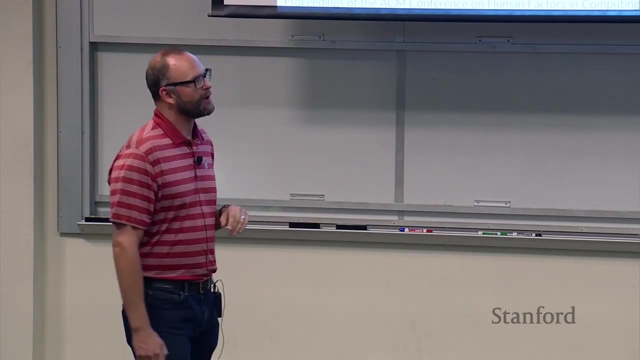 to the output side. So can we make the device a bit more aware of your attention, such that when you return it to the device after looking away, it can aid you in task resumption? So it's affecting the output of the display. So, as I mentioned before, 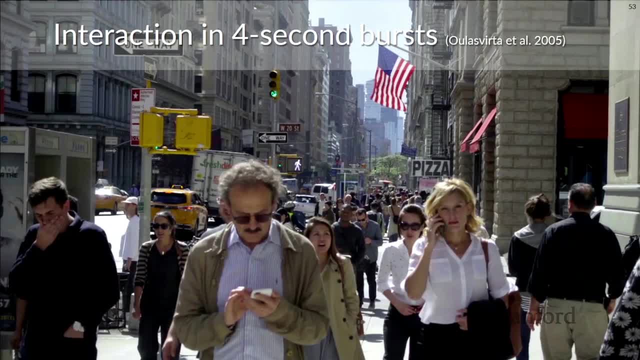 results show that there's about a four second burst of interaction. if you're mobile with your phone, You're not generally attending to the screen longer than that. Of course that's somewhat dependent on how crowded things are and how risky they are and all the rest. 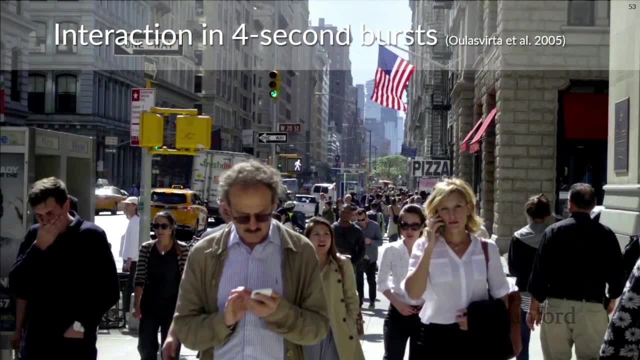 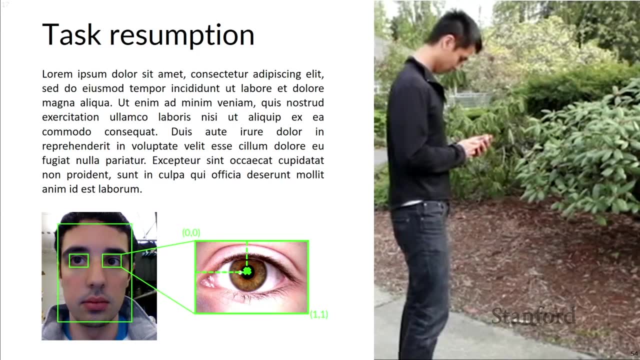 but that's a reasonable average. The point is it's a small number, small amount of time And with Switchback we applied it to reading, because how many of you had the experience where you've read? even in just an old paper book, you've read the page. 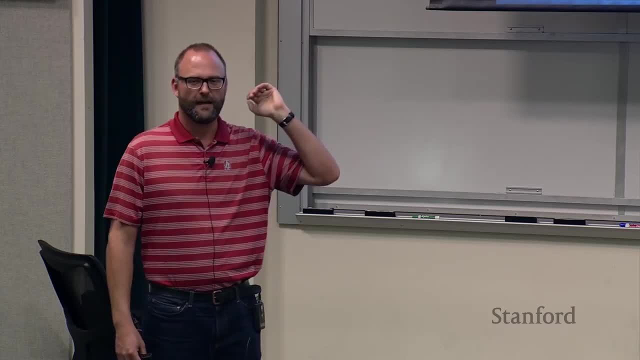 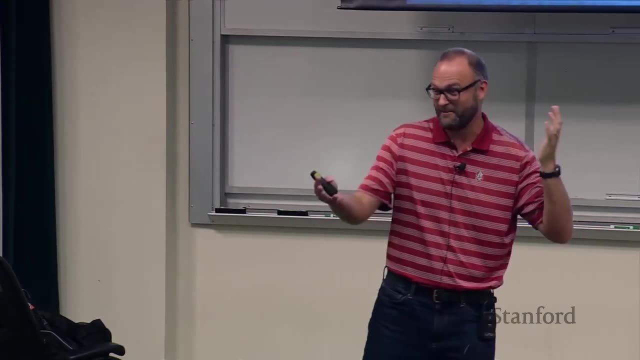 you look away, you look back and you start way above where you left off. I never started below where I left off. Anyone ever start further than they thought. Not so much Maybe. Yeah, You're living in your own future, But usually we kind of go to the top of the page. 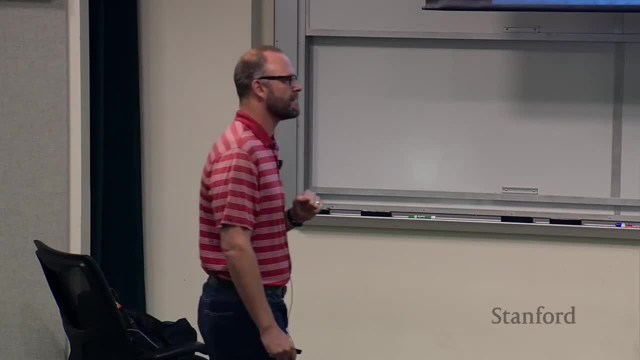 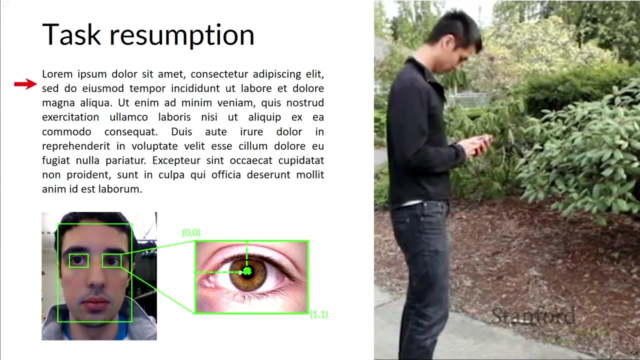 or some, maybe landmark. I'm not quite sure what the phenomena is there at work cognitively, But what we wanted is people can read and then so they're reading down the lines and then, as they look away- and we know they will- when they look back at the screen, 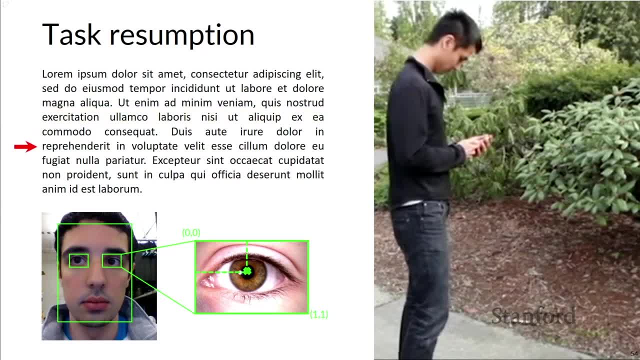 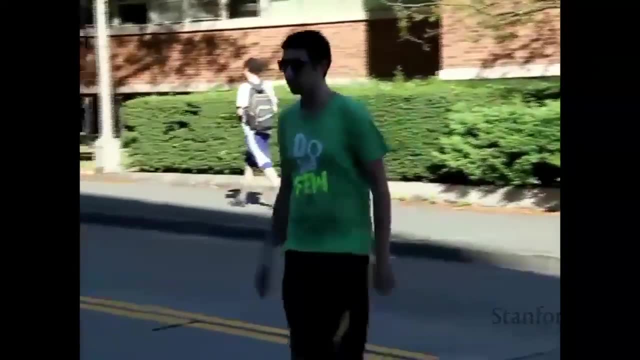 we do some highlighting- and we get inspiration here from Patrick Boudish's Phosphor desktop highlighting work and other things like that- and we kind of help them resume. Mobile devices are often used in environments that constantly change, forcing the user to break focus and attend to their environment. 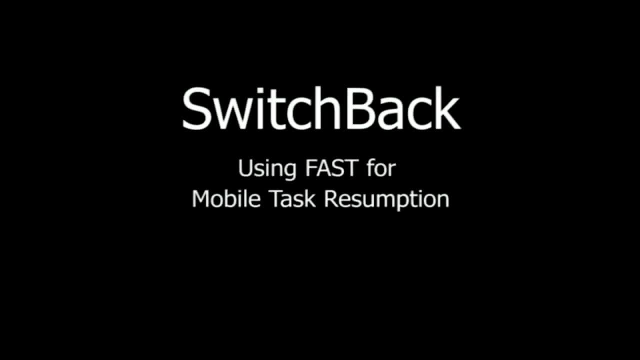 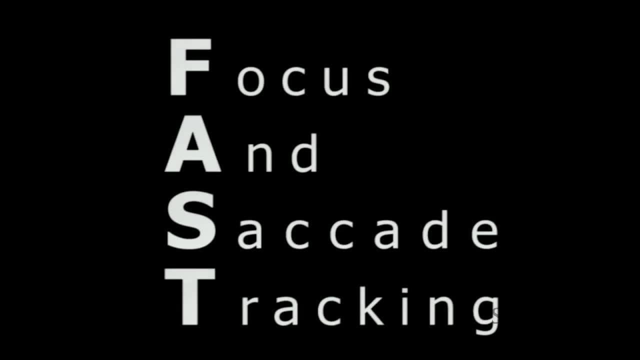 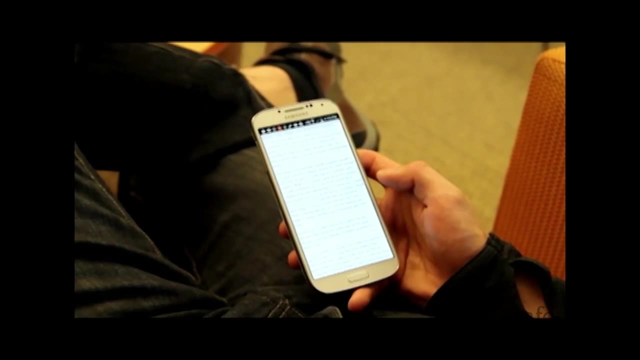 We introduce Switchback, a system that facilitates task resumption for mobile devices. Switchback is built upon our focus and saccade tracking, which uses the mobile device's front facing camera in two ways. Saccade tracking observes the user's gaze as it jumps to different parts of the screen. 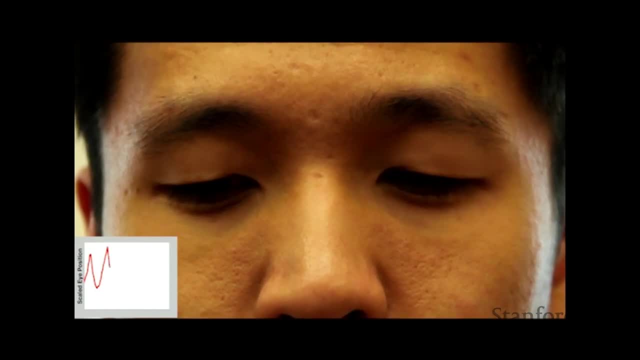 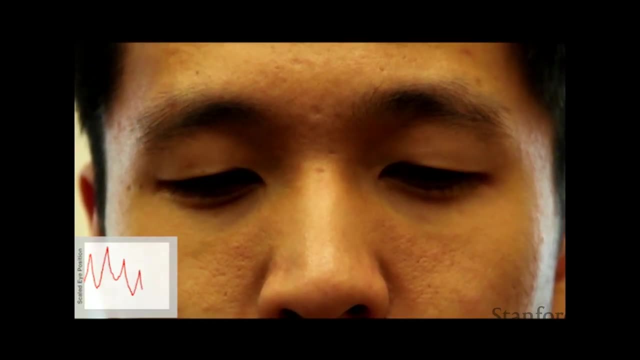 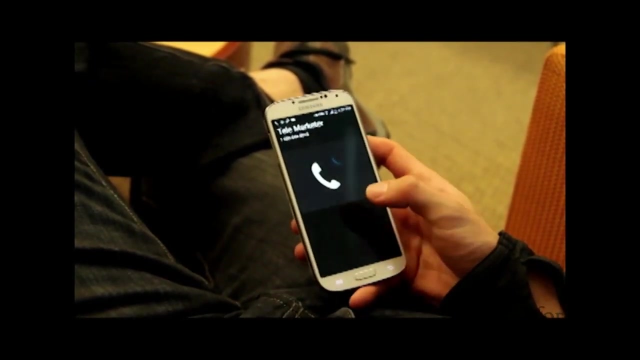 Here we show saccade tracking being used in the context of reading. Every large gaze jump across the screen corresponds to a new line being read. If the user becomes distracted, he risks forgetting where he last read. With Switchback, however, the system can highlight. 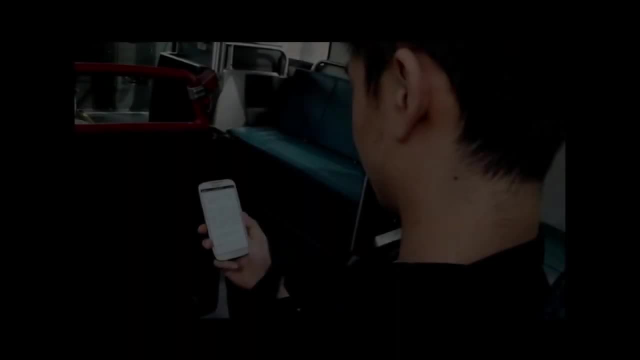 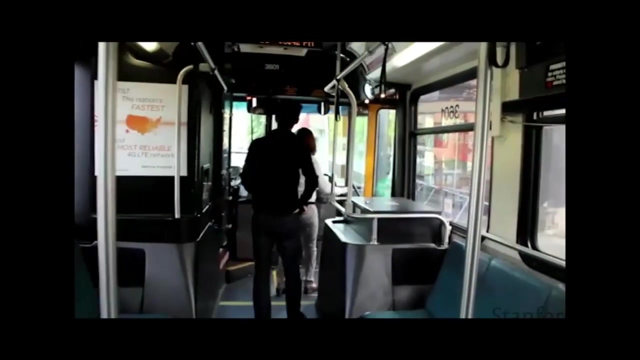 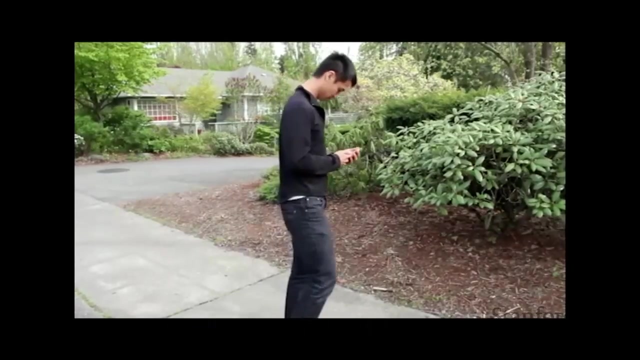 where the user had stopped. Focus tracking monitors the user's attention. As the user walks off the bus, he must look away from his device. Once the user returns his focus to the screen, Switchback can draw his attention to where he left off. So you might think. 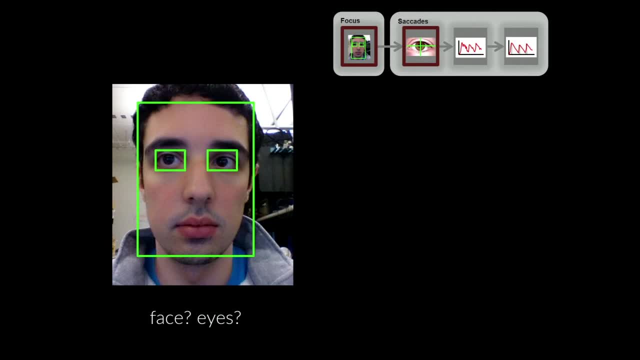 oh, just point the camera- the front facing camera- at the face and the eyes, track them and you can see the pixel they're looking at. That doesn't work. It's much harder than that It turns out. you can't get that level of resolution and accuracy. 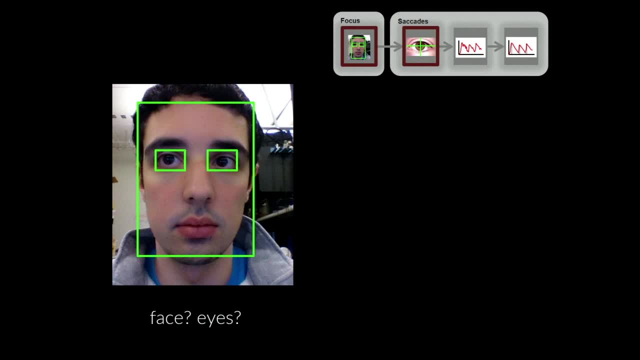 But you can do well enough to track, like we are, the eye movements in their saccades and generally the face at the screen and not and so on, And so you know, and that will improve over time and maybe eventually we'll have true eye tracking from a front facing camera. 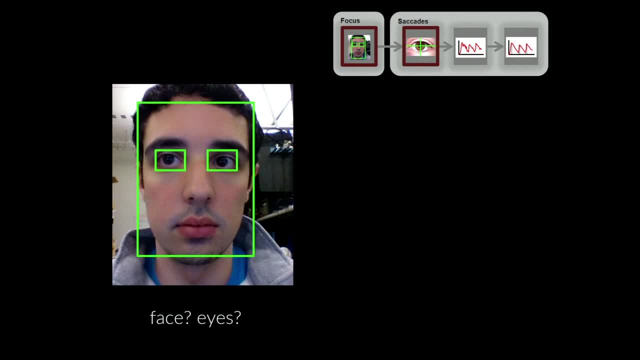 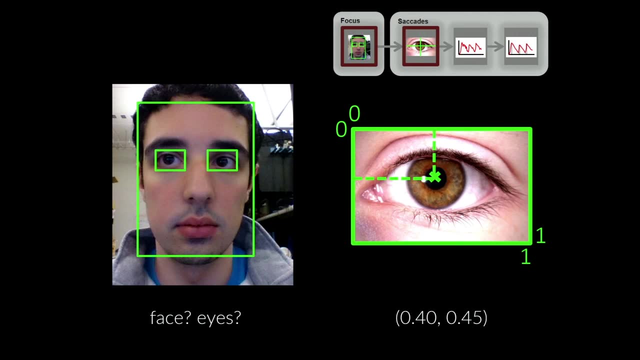 but we don't have that really yet. So we first check and see if they're looking at the camera or looking at the device rather, and where the pupil is. These are fairly conventional computer vision techniques And then, as you saw in the video, we can actually track the movement of the eyes. 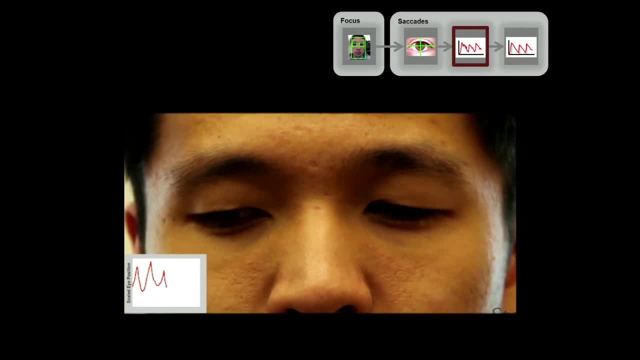 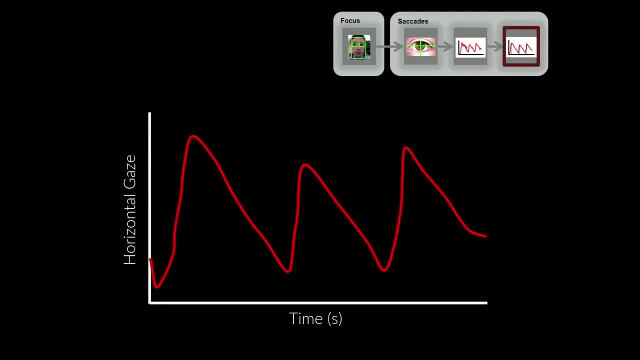 well enough to know where the saccades happen. The saccades are the jumps from the end of one line to the next, And so then, knowing that we can do some basic things like smooth the signal, find peaks and valleys, and then infer the saccades, 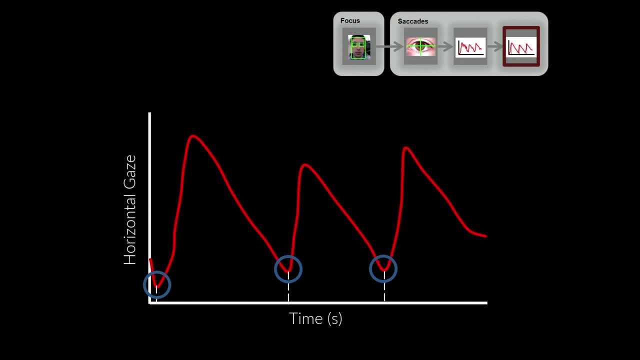 and therefore the lines red. So this is massive and it's mapped right now to reading. but that's where we found it's actually particularly problematic, because you've got a high resolution set of lines to read like a New York Times article or something and you're looking away. 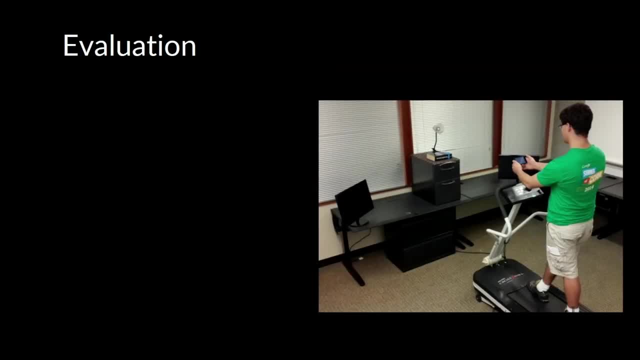 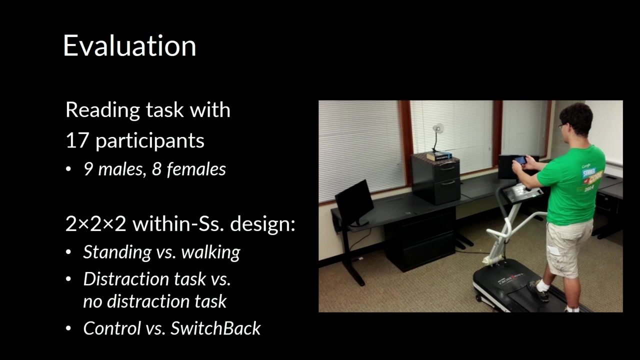 and it's hard to kind of resume. We did evaluate this in a controlled experiment. I'll quickly mention So. we had a reading task with 17 participants and they went through a two by two within subjects design, with these three factors of two levels each. 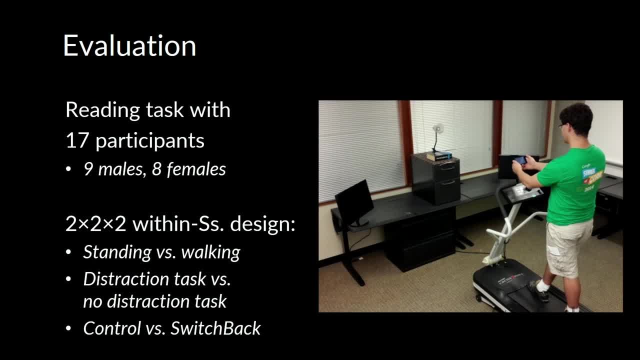 So they were standing versus walking- a distraction task that we took from psychology versus not having that, and then a control condition where they didn't have switchback and switchback. Their reading speed was validated with a comprehension test to make sure they actually did read it. 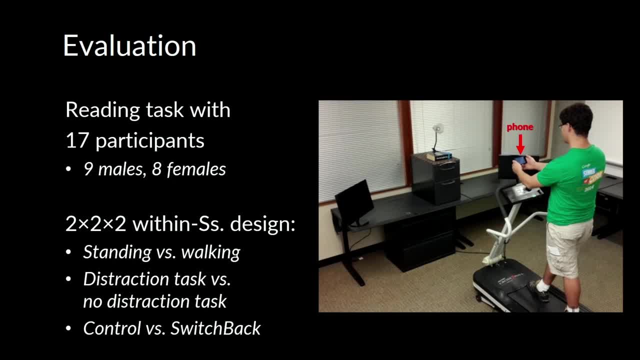 So the phone is here, they're on a treadmill, so there is that laboratory aspect to this. but the phone is there and then the distraction task for that condition does appear there, which essentially asks them to count the number of L's in a field of T's. 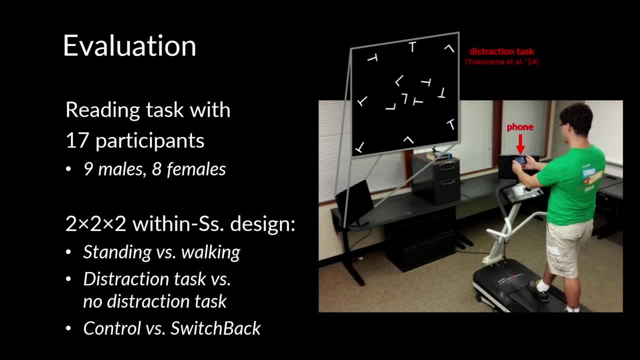 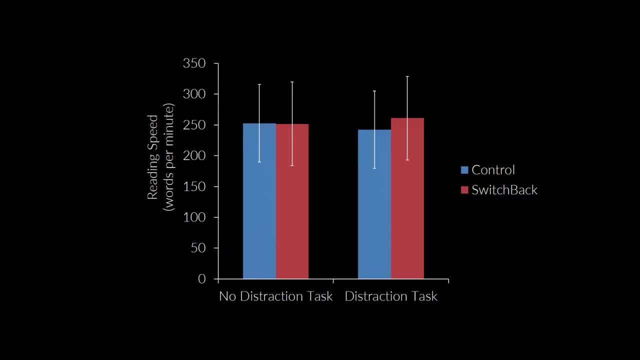 which is not that easy and takes a few seconds. so it forces them to look away and then by doing so, we can see how they resume And what we see for reading speed here on the left side, without the distraction task, there's no difference, So that's good. 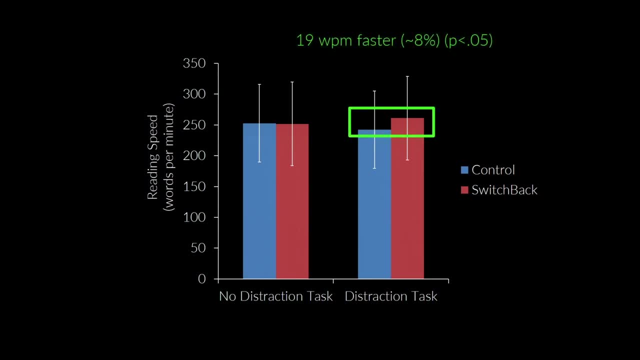 we're not doing harm, but when there is a distraction task we're getting about an 8% win in reading speed. It's not massive, but it's. it was statistically significant and more to the point. you know. we're seeing that there is some benefit here. 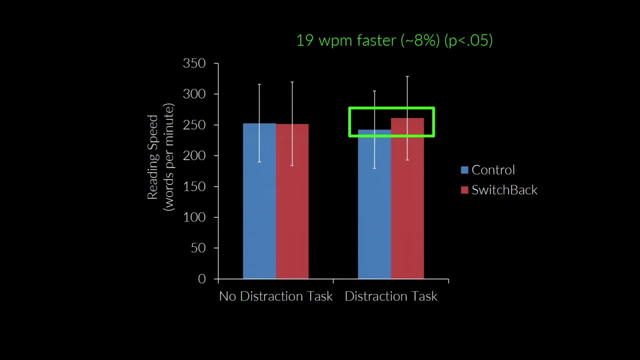 That's about 20 words a minute faster. That'd be great on an entry side. on the reading side it's a little bit of a less percentage, but it's still a nice outcome. And then the last one I want to touch on before I wrap. 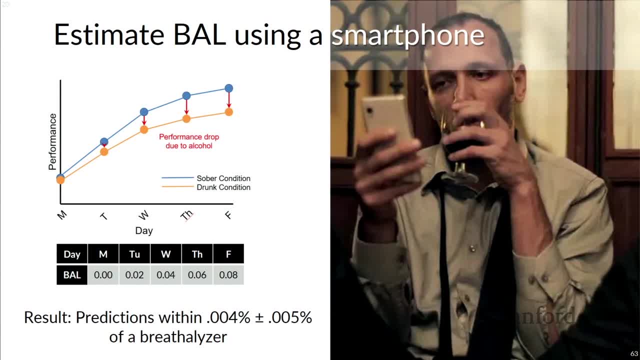 and take some questions. is DUIs Instead of GUIs? these are DUIs- drunk user interfaces. What are drunk user interfaces? So the idea was: can we actually estimate the blood alcohol levels of a person using a smartphone? This turned out to be a very popular study. 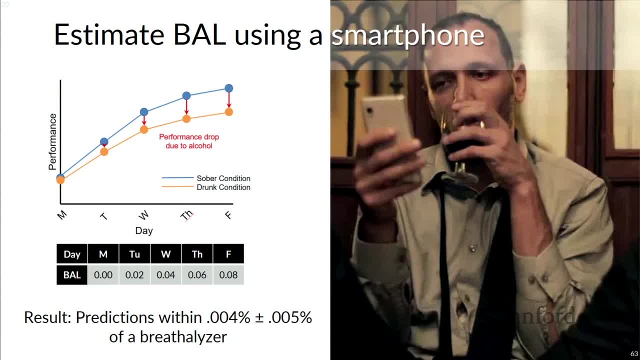 among the students 21 and older at the university. We got lots of people to sign up for this because we got them drunk over the course of an entire week And this was all totally approved by the IRB. That was, I just want to make sure. 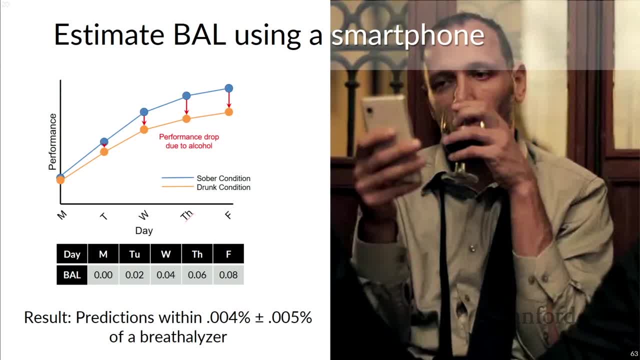 that's on the video. But we actually had them go from a completely sober condition all the way up to the legal limit. We did not push them beyond that for ethical reasons. Just so you know. 0.04 is what the national health standards say. 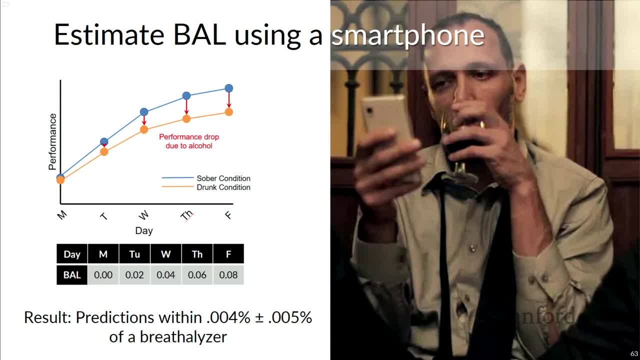 is the decision boundary between if you're beyond that, you're drunk, and if you're or you're not sober, I should say, and below that you're still considered legally sober. And so we developed some tasks, which we call drunk user interfaces that help us model. 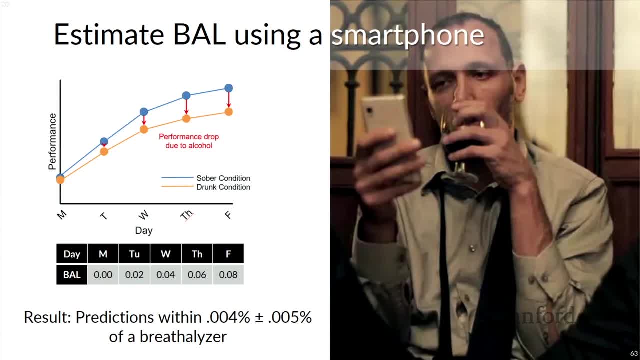 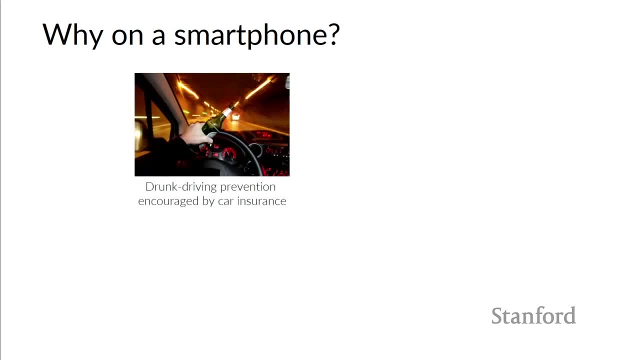 the change in human performance when you're drinking, or drinking alcohol, or drinking alcohol under the influence. Now, why would you want to do this on a smartphone? And we're not reading blood levels, right? We're not pricking people, They're not pricking themselves. 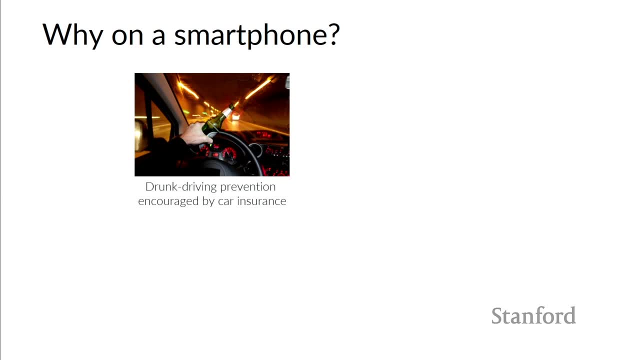 with their phone? We're not. it's not a direct reading. Well, you know, people might want to prevent drunk driving and maybe their car insurance says: you know you get this app and you use it after 10 pm if you're going to drive. 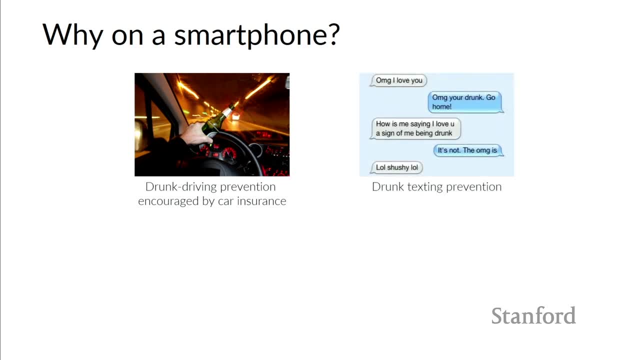 and we'll give you a discount. Or maybe this is the best use case on campuses: drunk texting: perfection: OMG I love you, OMG you're drunk, go home. How is me saying I love you a sign of me being drunk? It's not. 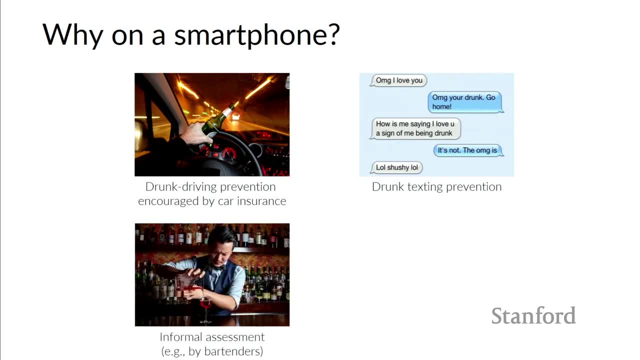 The OMG is. I think that's funny. Apparently you don't as much. That's okay. Informal assessment situations do happen, So bartenders sometimes want to verify or know if someone's maybe had too much, or maybe you want to do that for yourself. 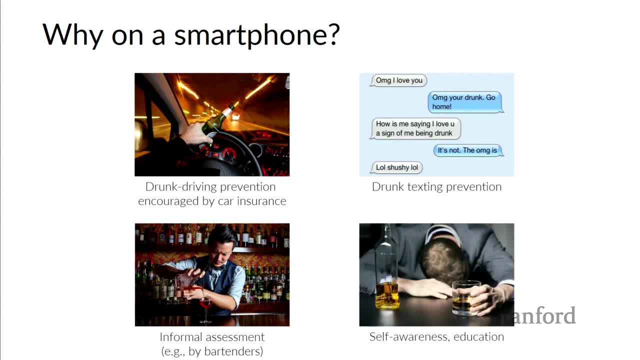 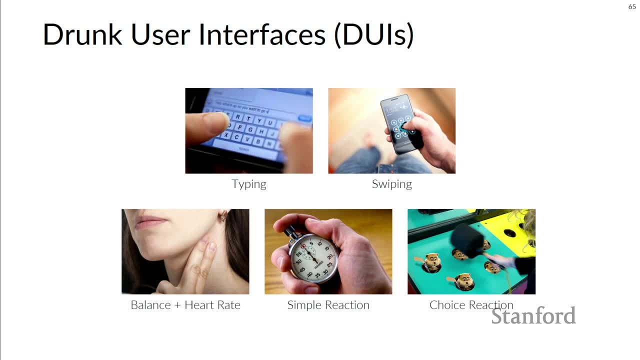 So self-awareness education, things like that. So these are the five tasks that, after exploring the whole range of human performance tasks and other types, we came to Typing: swiping combined balance and heart rate task- It's hand balancing, not the whole body. 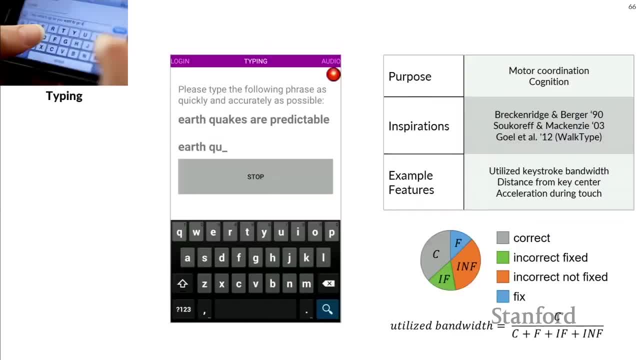 Simple reaction time and choice reaction time. So some of these are very old psychology tasks. In text entry they enter some phrases. There are a lot of different features we could pull off. this One is called utilize bandwidth. This is a text entry measure. 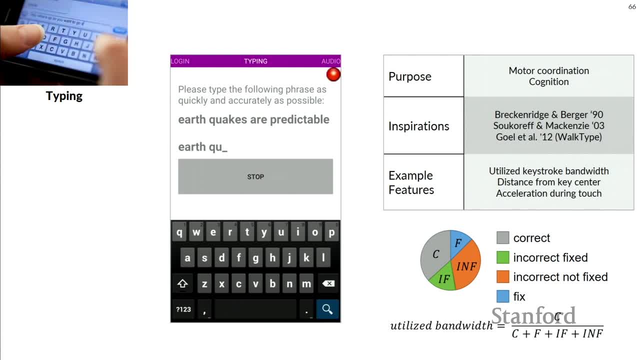 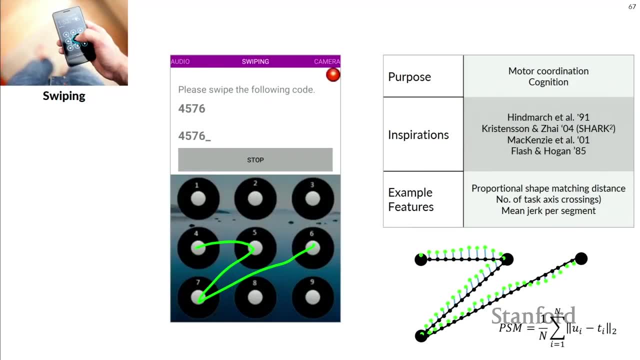 But it amounts to basically how many of the characters you strike are useful in the phrase you're typing. Another one is having them swipe on a lock screen and actually taking their the difference at each point from the idealized trace path between the centers of those targets. 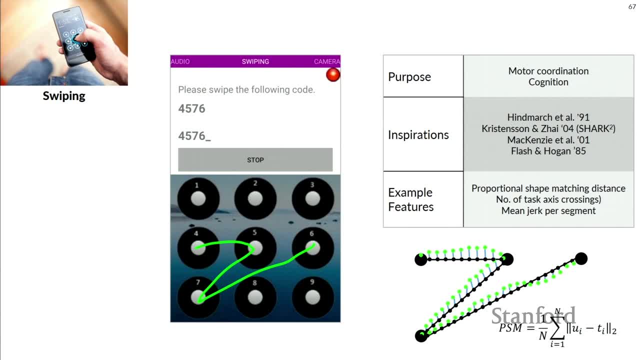 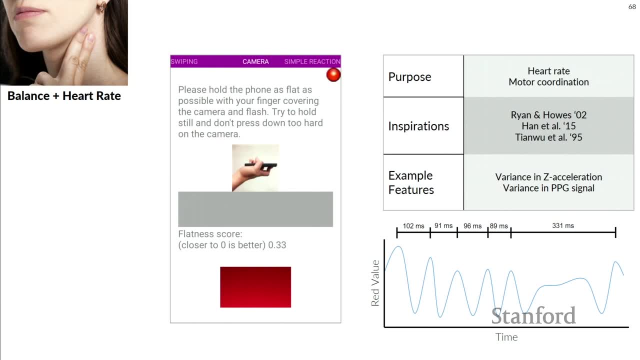 You might not be surprised to learn: the more drunk you are, the harder that is to do. This one's actually quite cool. The balance and heart rate is such that you hold the phone with the flash on, but you're covering the camera And we can read. 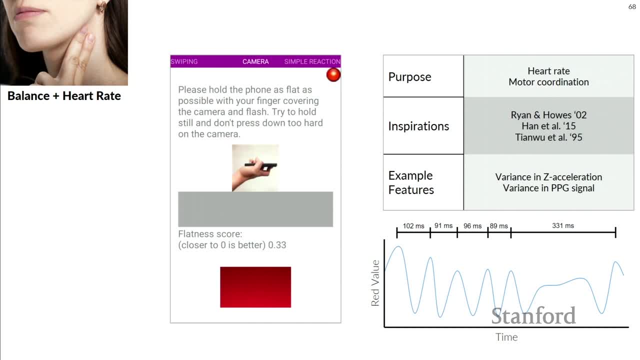 the color of your blood, And that turns out to be a medical property that has a really long name that I can't remember. It starts with a P. I should have put it on the slide. But the color, the variance in the color over time. 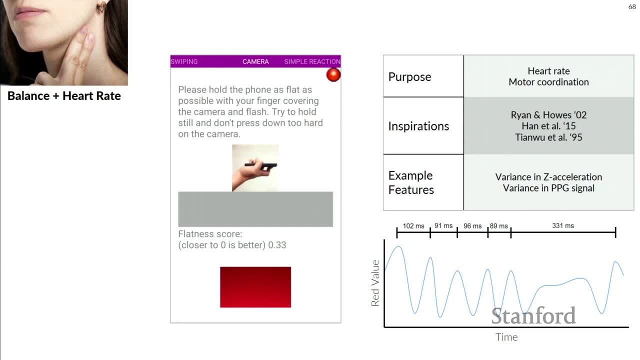 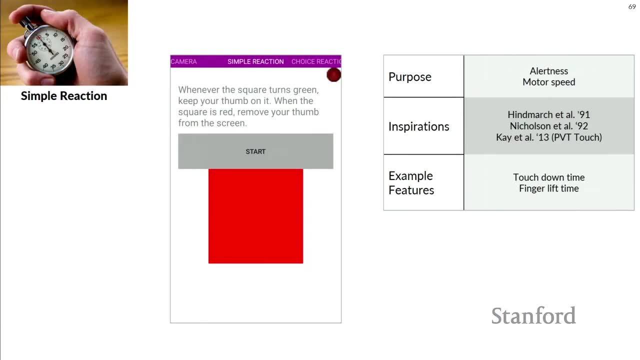 will tell you how much alcohol is in the blood And we can read that through the through the camera, when it's illuminated enough by the flash. Simple reaction time. So goes to green, touch it and then it actually goes back to red. release it and choice. 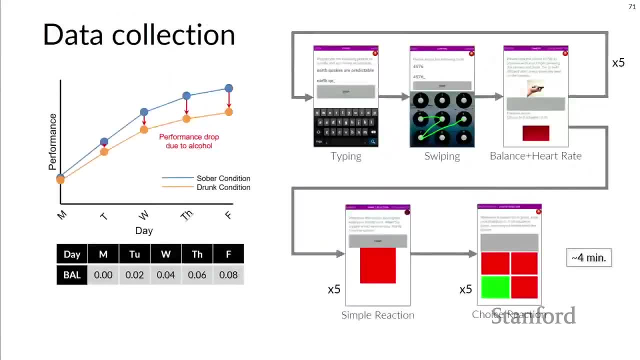 So multiple options? Okay. So what do we do with that? Well, we had people go through this process. It takes only about four minutes to run those first three, five times each. So a phrase, a swipe and the balance and heart rate and do that loop. 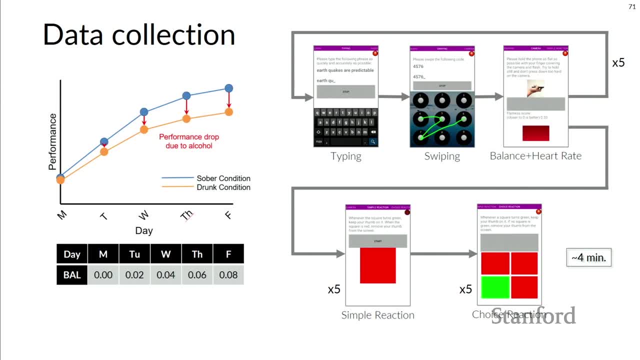 five times And then do simple reaction and choice reaction as well. That whole thing takes about four minutes And progressively across a week at 5 pm. that was the start time. we had people come in and normalize for fatigue and other factors, come in and drink. 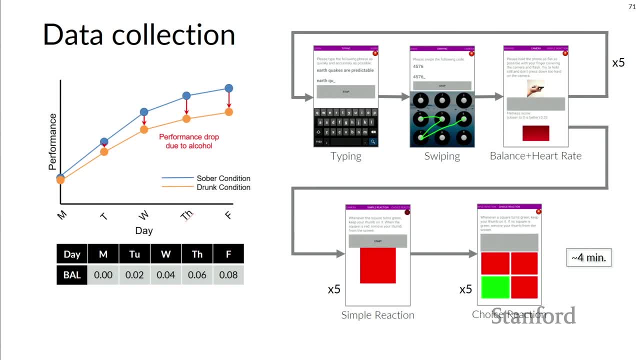 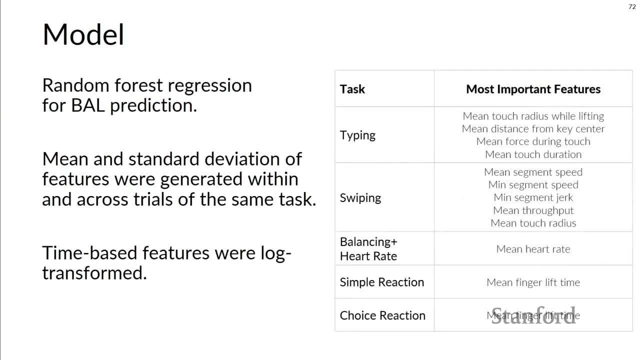 screwdrivers until their breathalyzer measurements got them, showed them at the right level, And then we know kind of ground truth where they're at. And then we built some random forest regression models that had a number of features. if you want to see them all there in the paper. 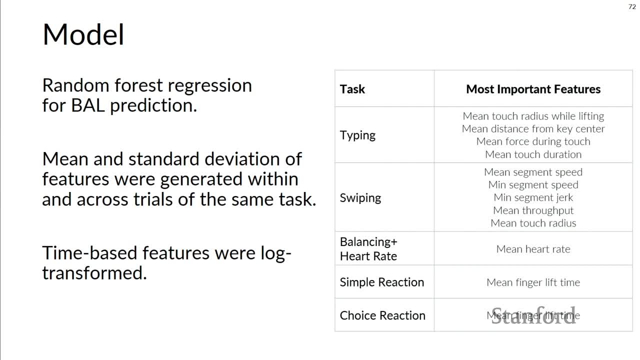 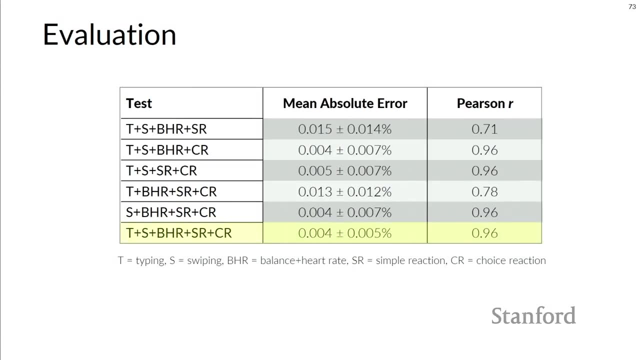 Here are some that are that were important, But essentially they're kind of what you'd expect. You know the times and distances and errors and things, And it turns out when you combine all of those tasks you can do pretty well. So we were within. 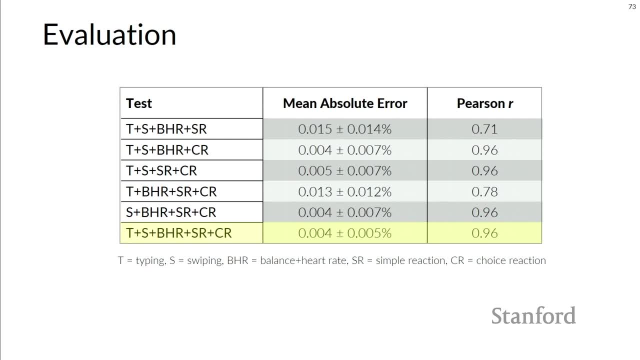 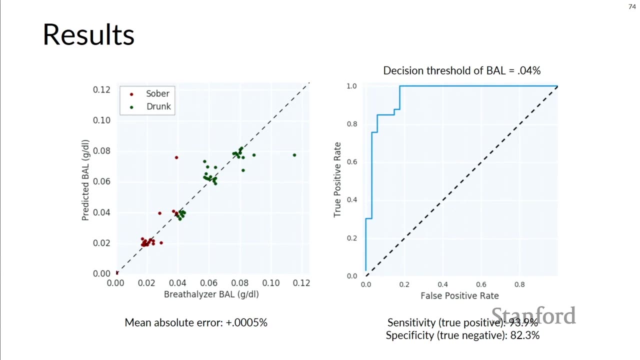 .004% of the ground truth breathalyzer measurement with a standard deviation of .005% And the breathalyzer and our measurements correlated with about a .96 measurement. You can see that here on the left, The model predictions and the actual breathalyzer measurements. 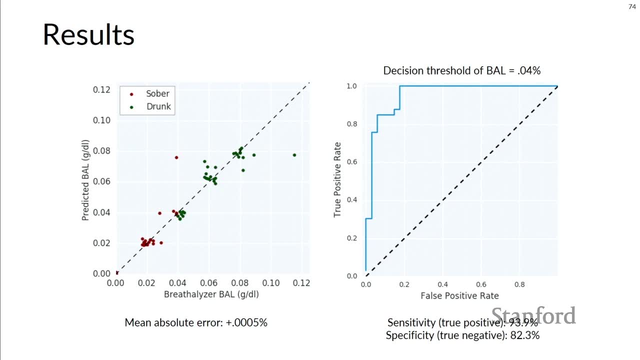 are pretty close, And if sensitivity is we say you're drunk and you're actually drunk, and specificity is we say you're sober and you're actually sober, and that's at the decision boundary of .04, then those are our numbers for sensitivity and specificity. 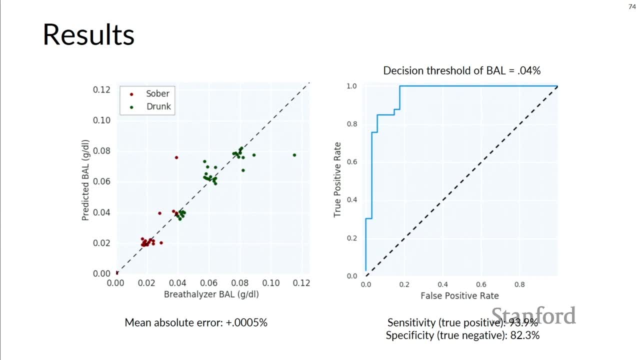 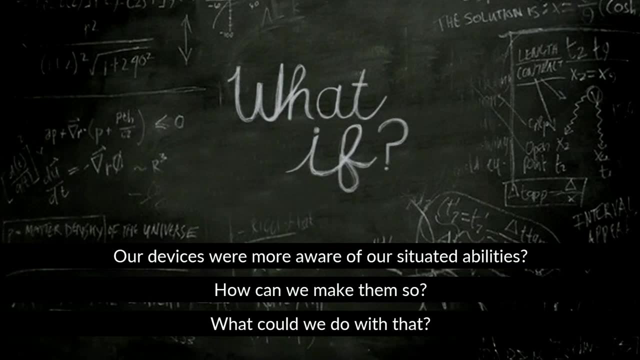 So it's kind of a fun project to explore what's possible there, But the predictions are actually pretty good in the end. So let's return to these questions here. Our devices were more aware. what if our devices were more aware of our situated abilities? 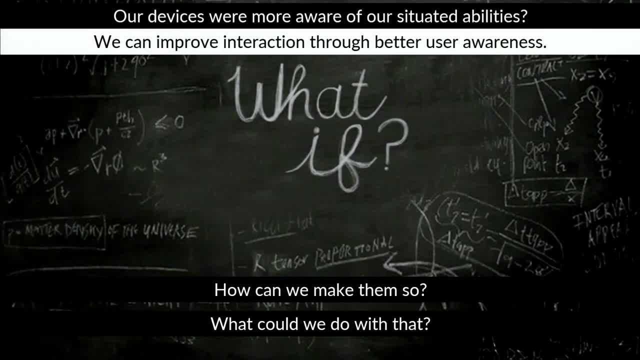 how can we make them so and what can we do with that? So I would say, and I hope you will agree, that if we can make them more aware, we can improve interaction through better user awareness, The device being more aware of the user, And we can make them. 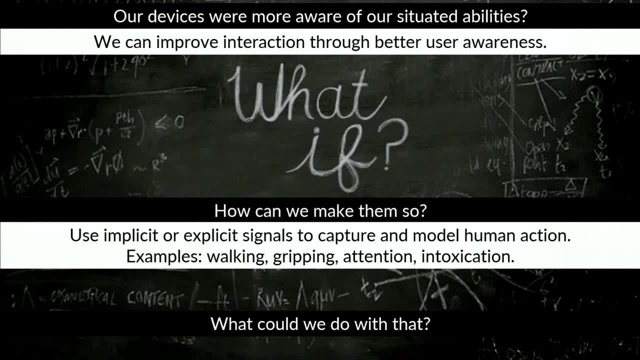 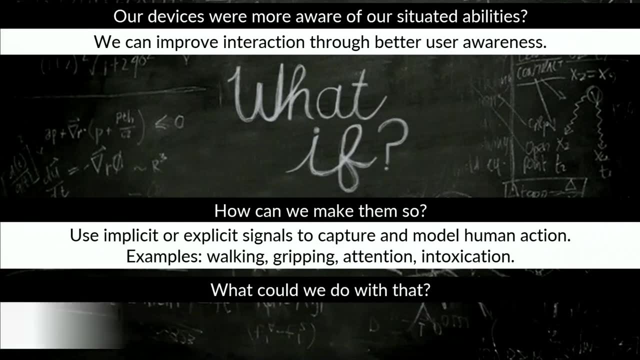 this way, with implicit in most cases. so most of the project. three of them were implicit signals, one was explicit and the other one was not. So we can structure and model human action and we can do that with walking, gripping attention and intoxication, and others as well. 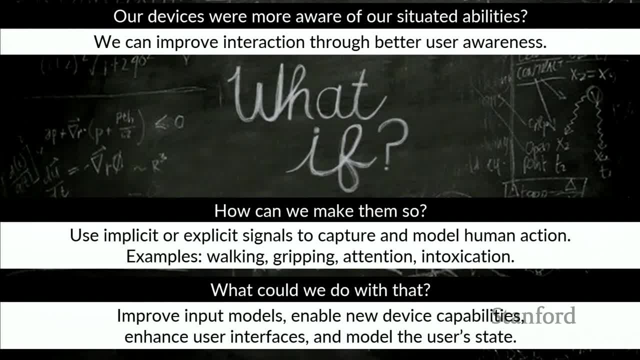 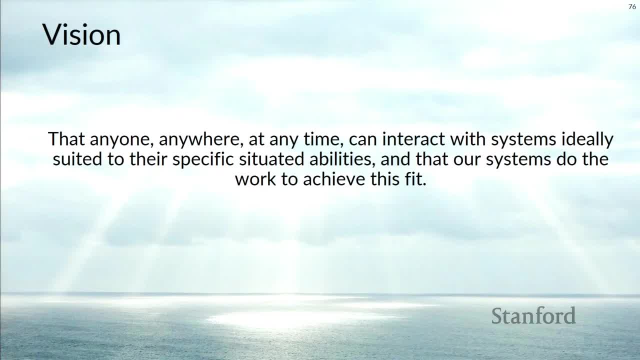 but these are the ones we saw. And then what can we do with that? Well, I hope you'll agree that you saw that we could improve input models, we can enable new device capabilities, we can enhance user interfaces in some cases and we can model the user's state. 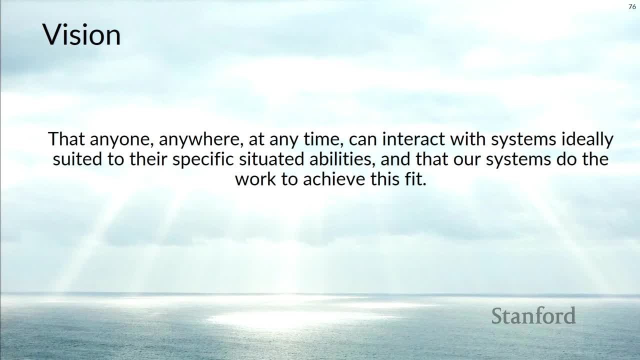 I think there's a larger vision at work here than you can imagine or see yourself in it. Imagine a world in which anyone, anywhere, at any time, can interact with our computing systems that are ideally situated to their specific abilities- sorry, ideally suited to their specific situated abilities. 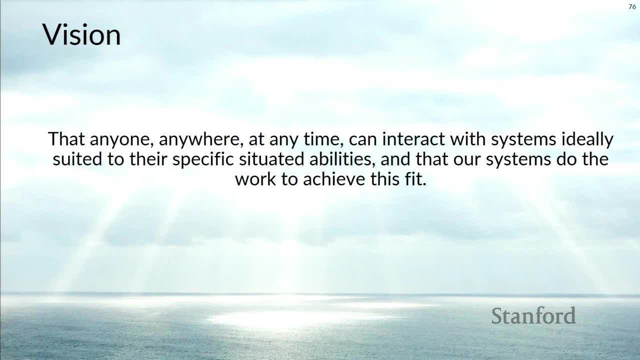 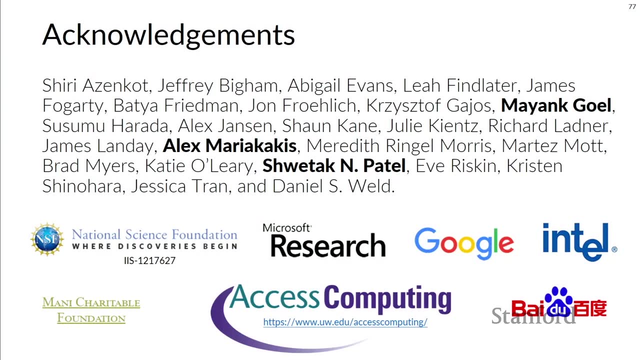 and that our systems do the work to achieve a fit instead of us doing the work to accommodate them- kind of flip that burden around. I want to acknowledge a number of people I've put in bold here and others who maybe weren't as directly involved with these projects. 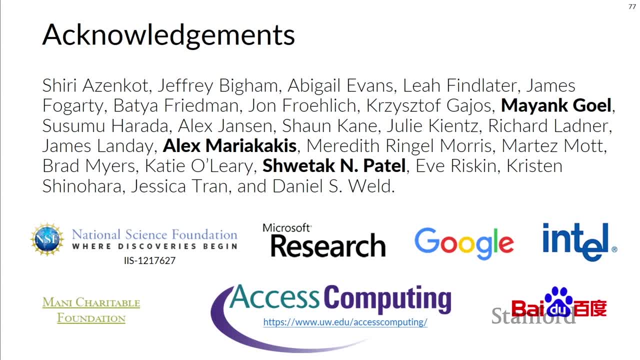 but have been part of my projects for many years. James is there just to make sure you see that and I'll stop there, Thank you.